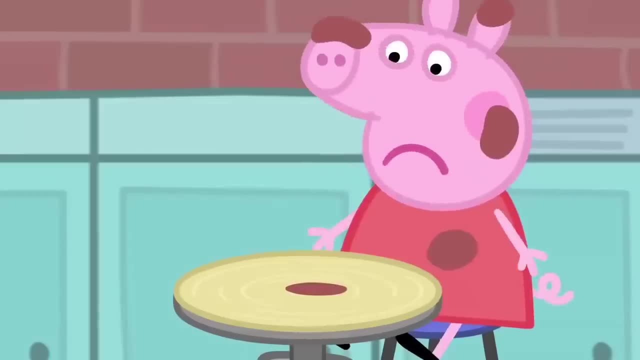 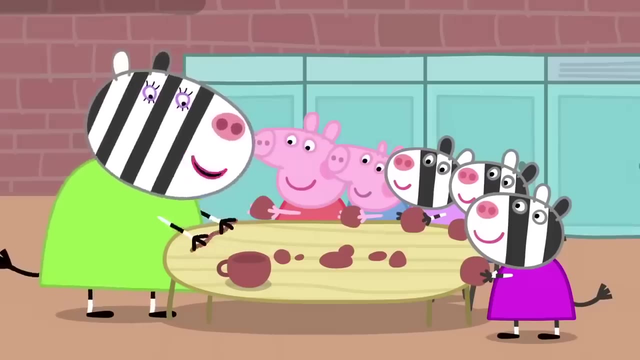 Making a cup on a potter's wheel Is not easy. There is an easier way to make a cup. First, we roll the clay into a long worm like this. It's a wriggly worm, I'm a wriggly worm. 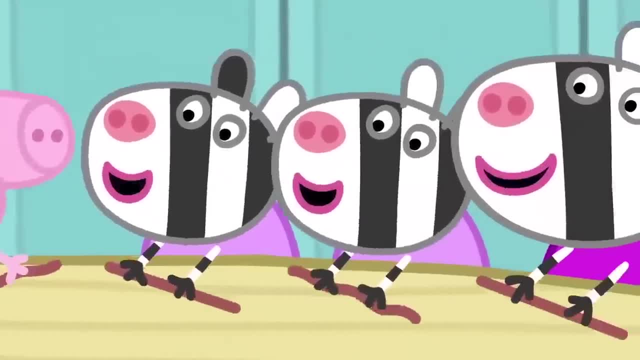 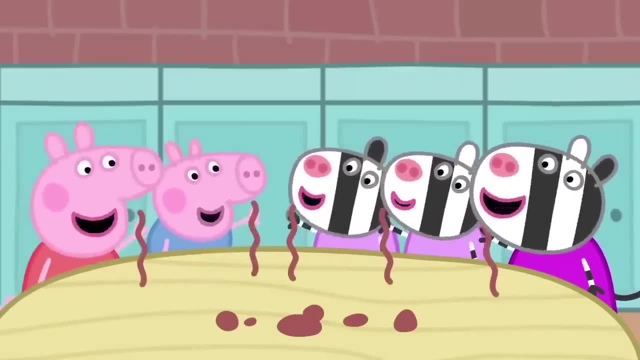 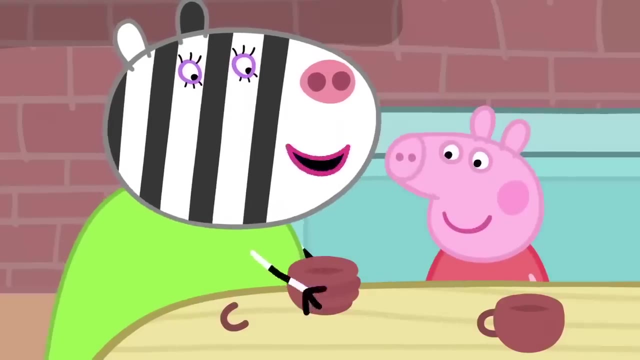 I'm a wriggly worm. I'm made of clay. What shall I make today? I'm a wriggly worm. We wrap it round and round like this. It's a bit bumpy. Now I smooth it out with my hands. 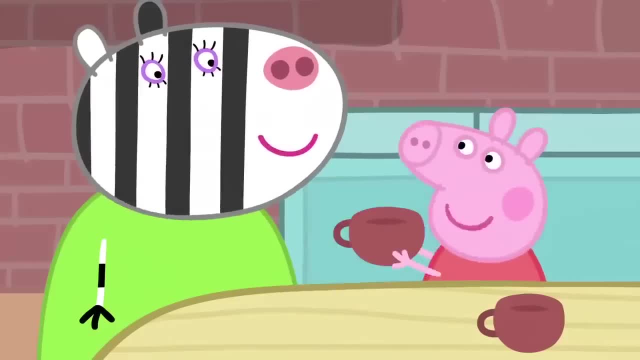 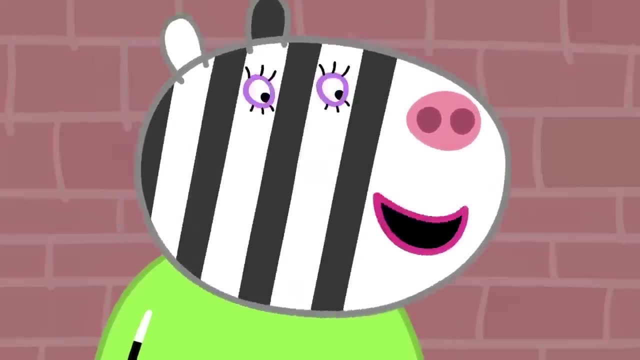 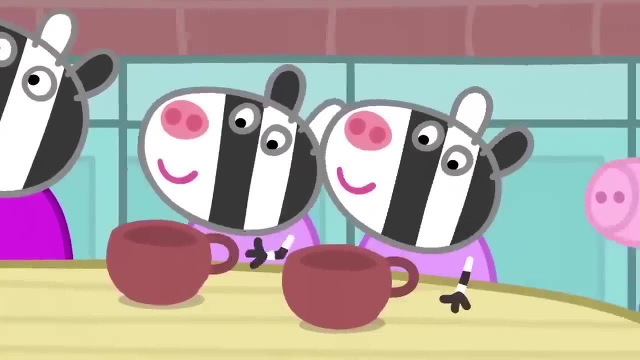 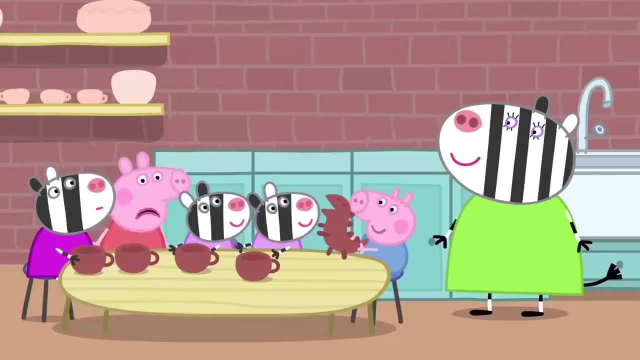 And I add a handle. It's a cup. Now we have two cups. Yes, but a tea set needs more than two cups. We'll all make cups. Yes, Dinosaur George has made a dinosaur. George always makes dinosaurs. 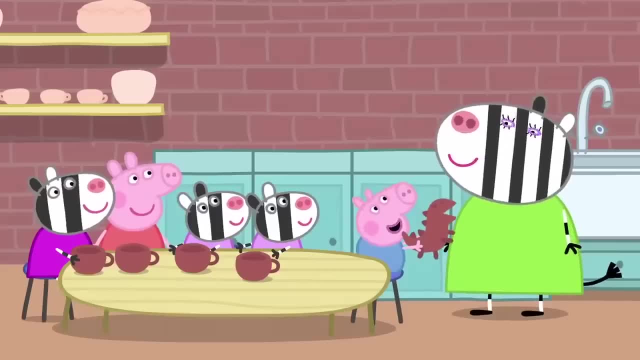 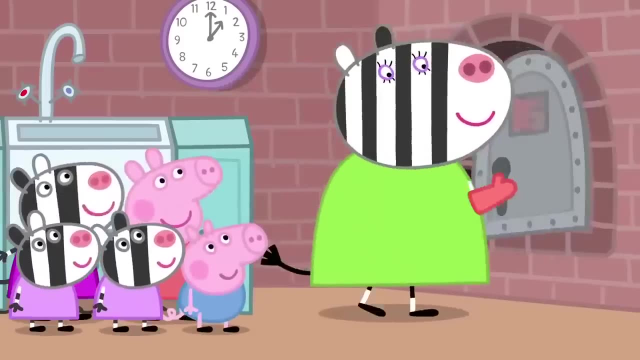 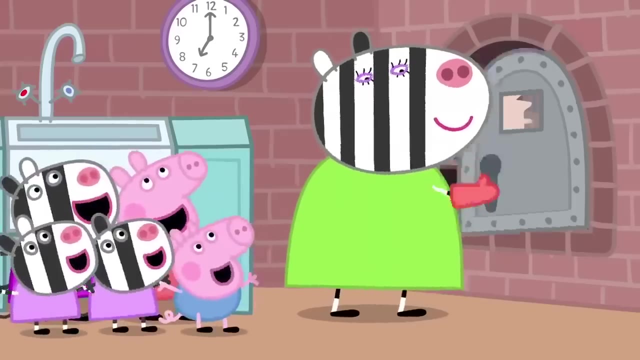 Oh, what a scary dinosaur. Now we need to bake the tea set in a kiln. A kiln is an oven that cooks the clay and makes it hard. The tea set should be ready. Hooray, Now we paint them. 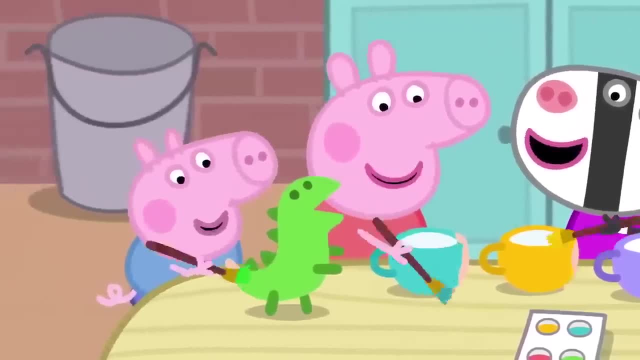 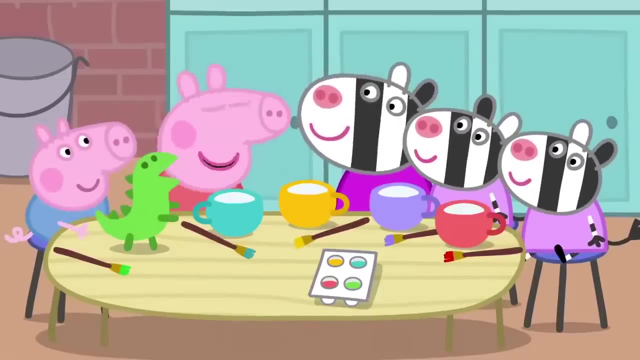 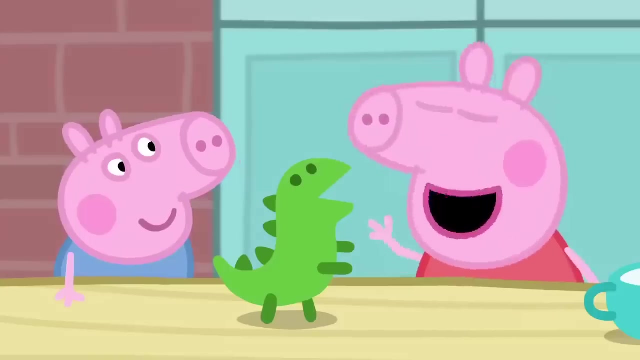 The children are painting the tea set Lovely bright colours. The tea set is finished. Now we can have our tea party. There's a cup for everyone. Oh, we forgot to make a teapot. I know George's dinosaur can be the teapot. 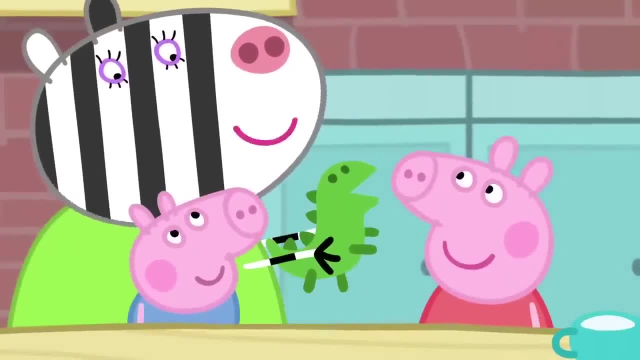 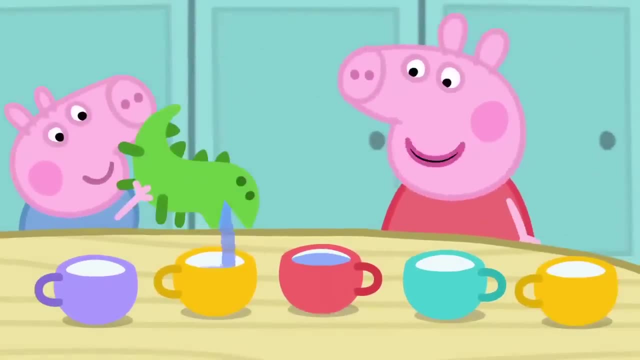 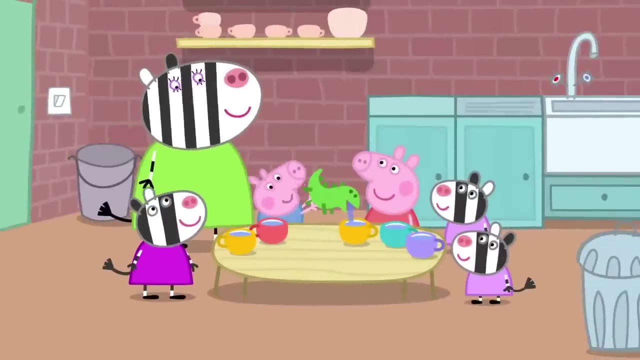 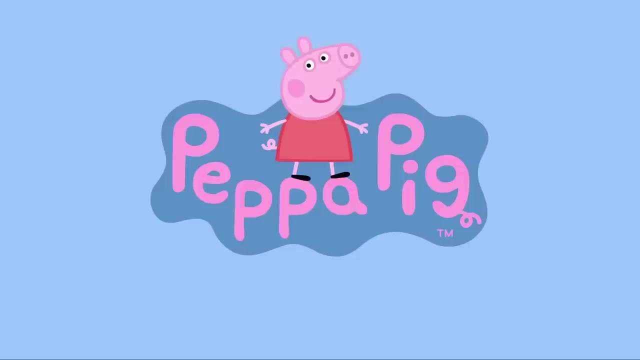 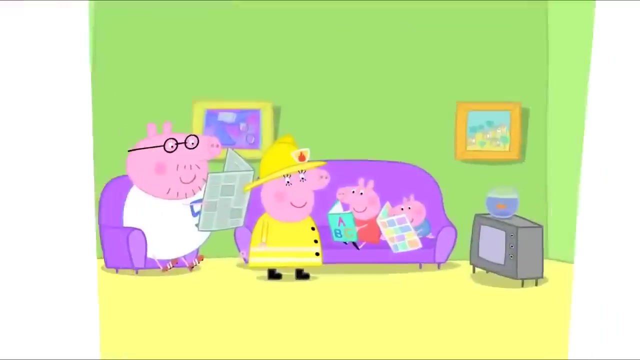 Yes, Let's fill it with water. This is the best tea set in the world. Everybody knows that all the finest tea sets have a dinosaur in them: Teapot, The fire engine. Mummy Pig is dressed as a fireman. Mummy, why are you dressed like that? 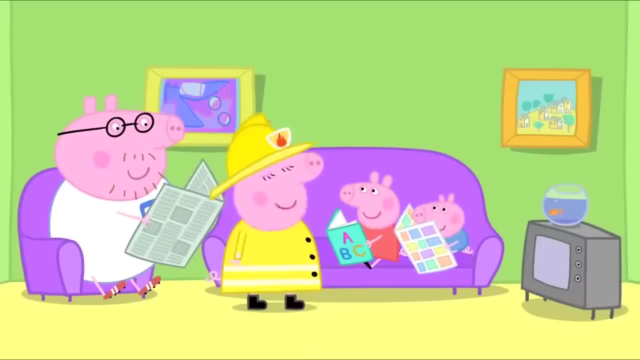 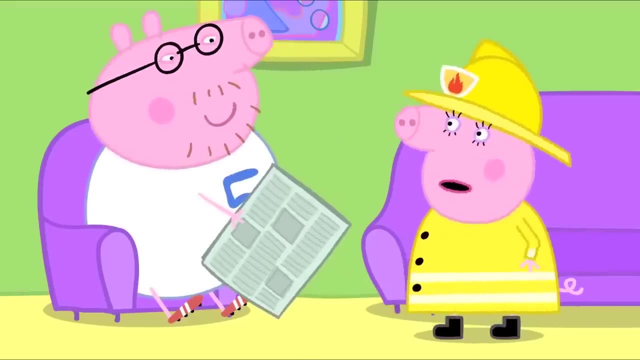 I'm going to the mummy's fire engine practice. Ooh Ho ho, It's just a good excuse for a cup of tea and a chat. Well, what are you doing today, Daddy Pig? I've got a very important meeting. 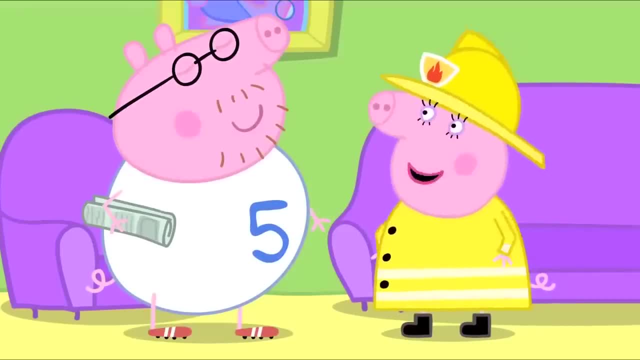 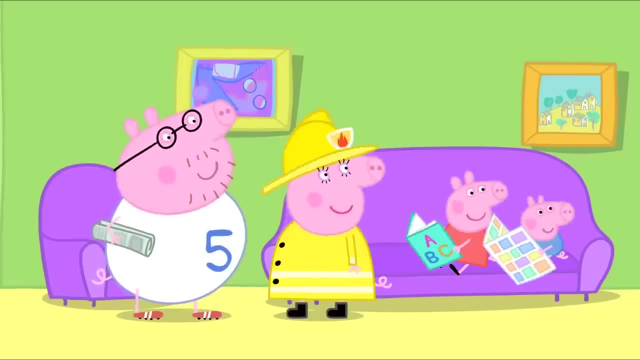 with the Daddy's football team. That's just a lot of grown-up boys kicking a football around. We're having a barbecue as well. Here are Mr Bullf, Mr Rabbit, Mr Pony and Mr Zebra Moo. 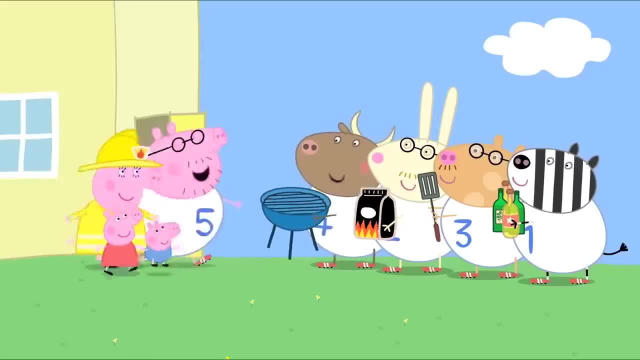 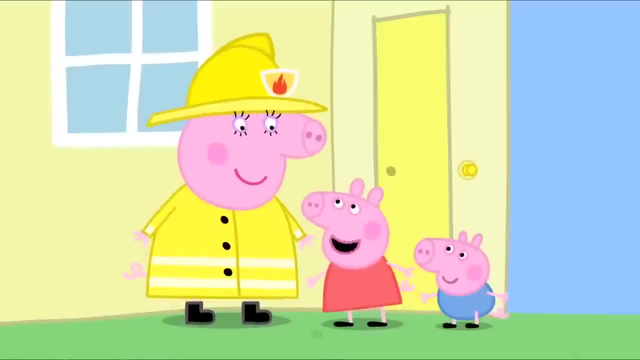 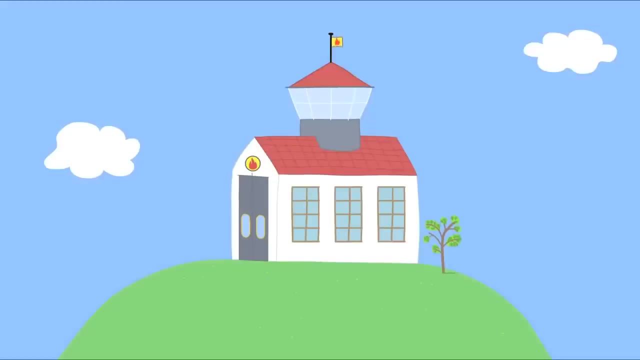 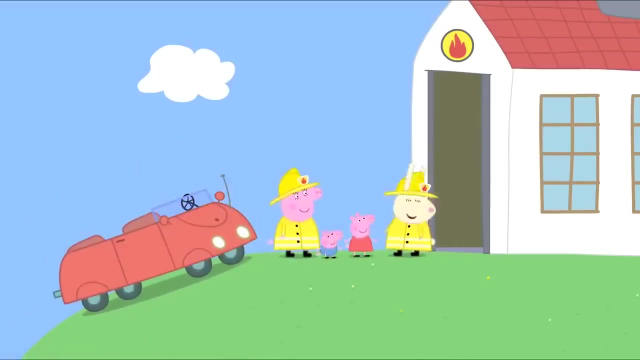 Is Daddy Pig coming out to play? Come on, Ho ho, ho, Mummy. can we see the fire engine? Yes, Oh goody, This is Miss Rabbit's fire station. Hello Peppa and George, Come and see the fire engine. 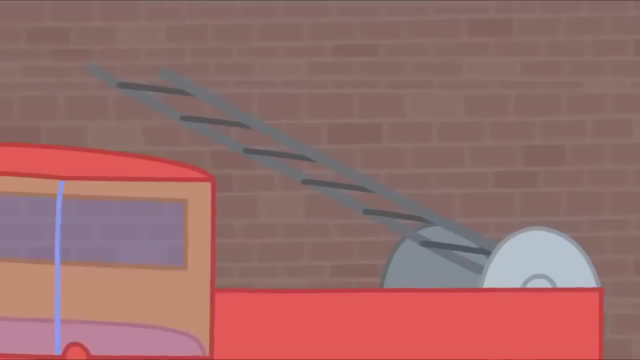 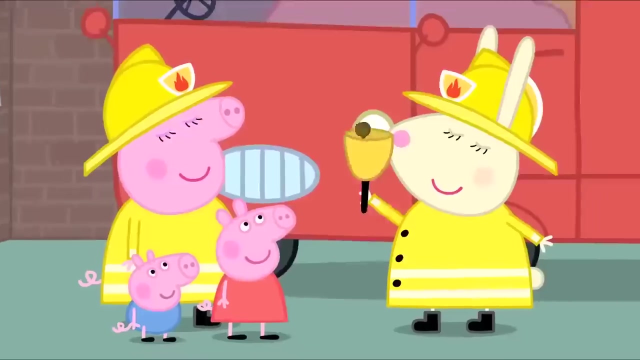 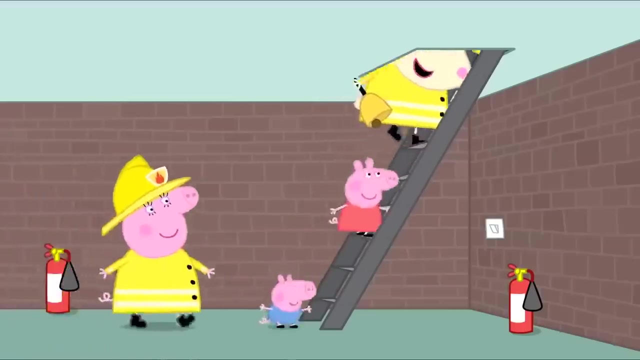 Wow, Fire engine. There's a ladder for climbing, a hose for squirting water and a big bell to ring Ding-dong, Ding-dong. Now let's go up the tower and look for fires. Hello everyone, Hello Peppa. 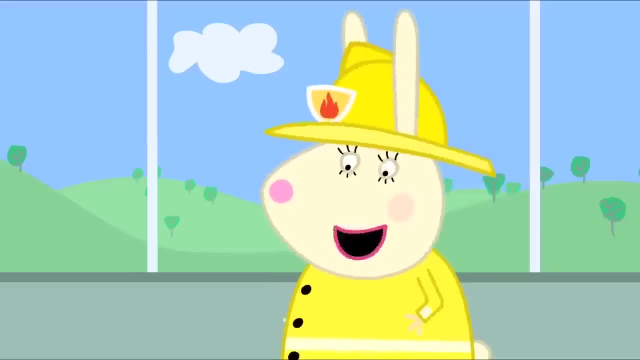 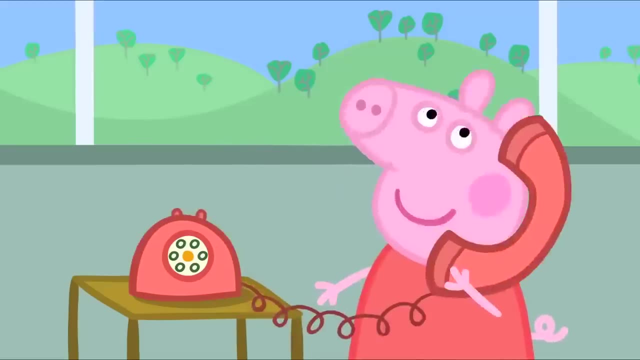 Hello George, Hello Peppa, Hello George. Oh, who's for a nice cup of tea and a chat? That sounds nice. Ooh, a telephone. Peppa, that is the fire phone. It's only to be used when there's a fire. 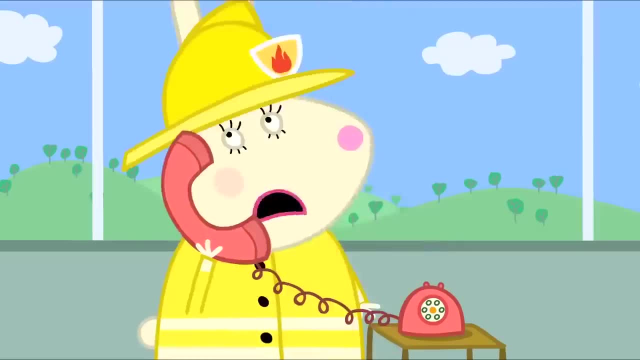 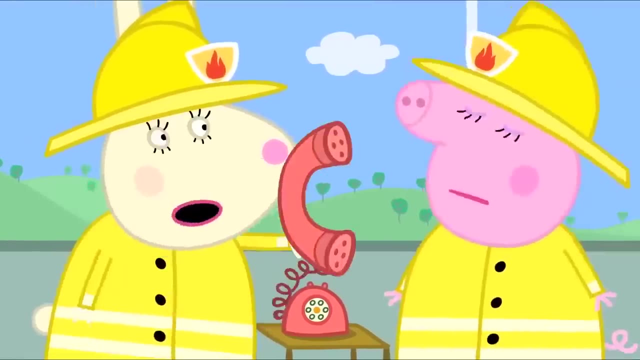 Ah, Fire, Fire, Fire station. Where's the fire? Where's the fire? Can I speak to Mummy Pig please? Oh, it's Daddy Pig. Daddy Pig, you're not supposed to ring on this phone, It's only for emergencies. 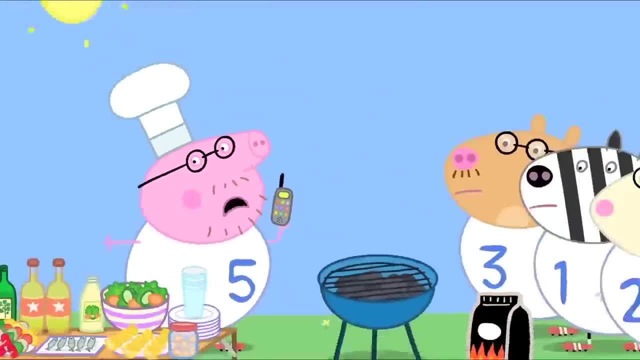 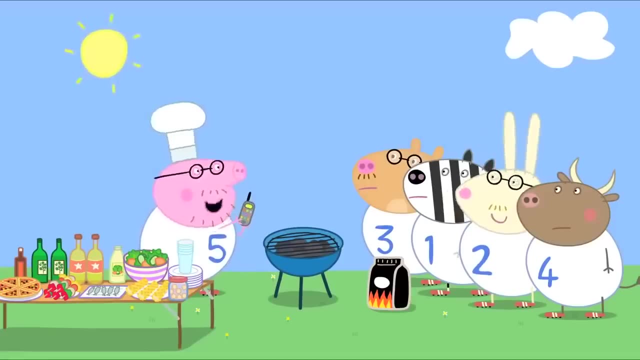 This is an emergency. I can't find the tomato ketchup anywhere. Daddy Pig, shall I light the barbecue now? Yes, please, Mr Rabbit, Do be careful with the barbecue. Daddy Pig, Trust me, Mummy Pig, We daddies know all about barbecues. 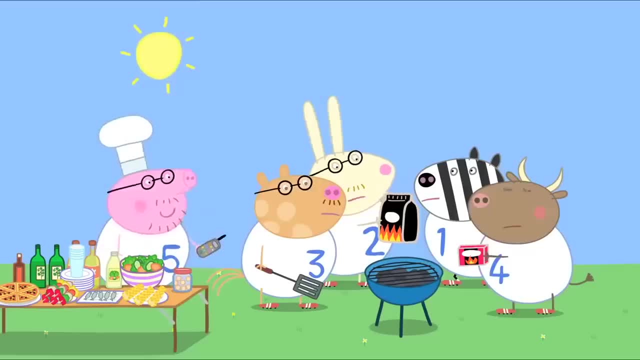 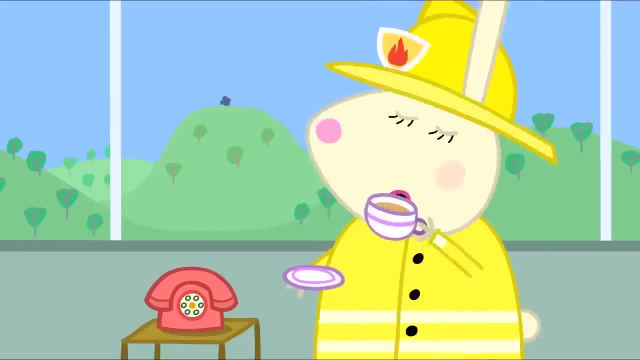 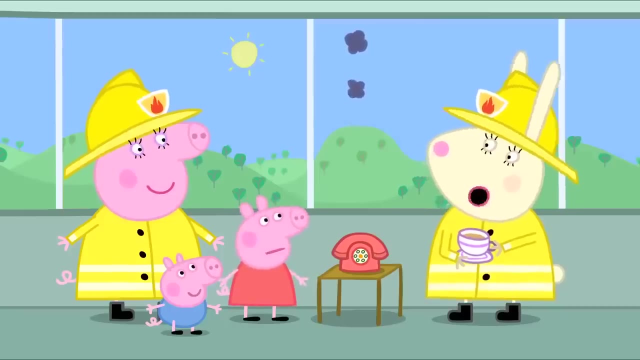 Bye. Maybe it needs more charcoal. Give it a bit of a blow, Put a few more fire lighters on. Now we just have to wait for a fire. How long do we have to wait? Oh, it could be a long time. 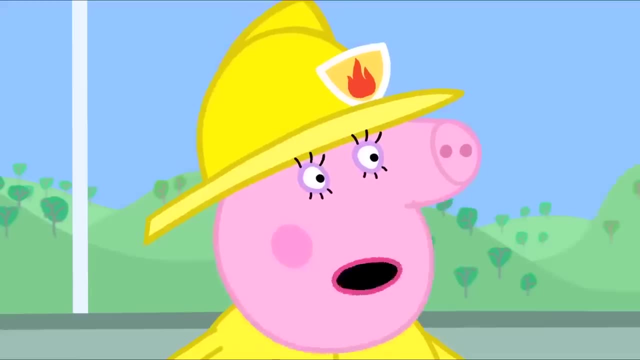 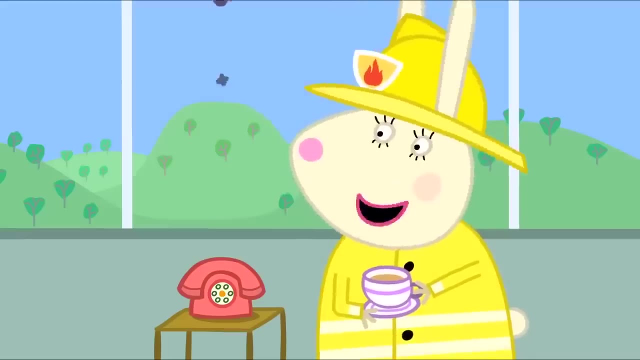 I've been waiting ages. How many fires have you actually put out, Miss Rabbit? Uh, none, Not one fire. But you've got to be ready. It's the fire phone. Oh, can you answer it, Peppa? 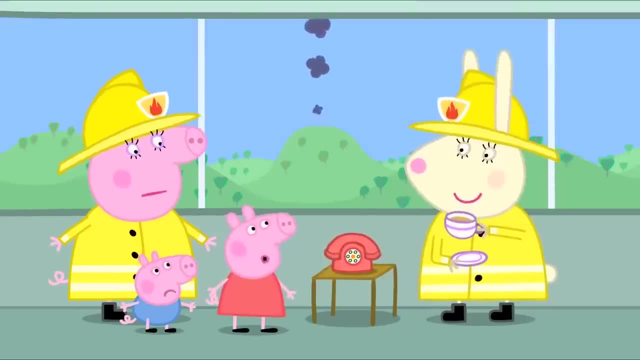 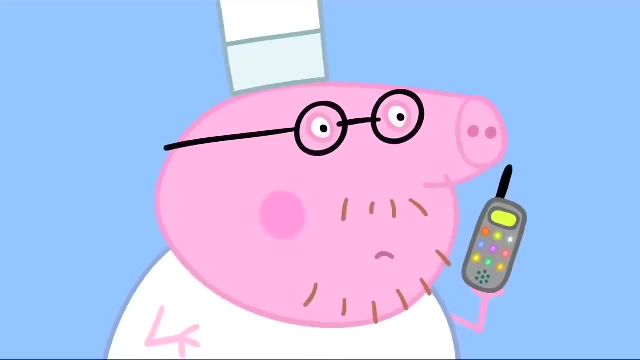 It'll probably be your Daddy again. OK, Hello fire station. Hello Peppa, Oh Daddy, it is you. You're very naughty. This phone is for fires. only Can you put Miss Rabbit on, please? There's a good girl. 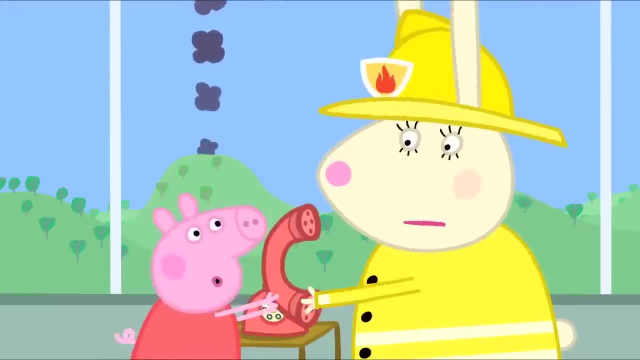 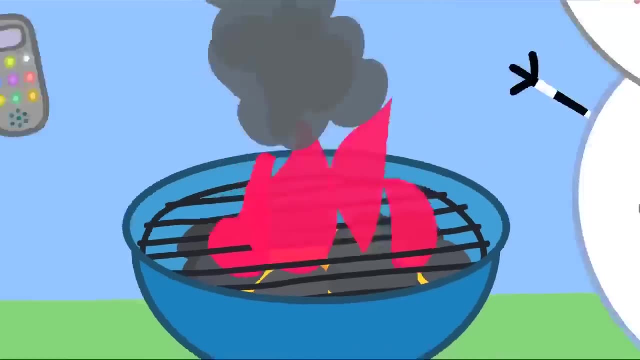 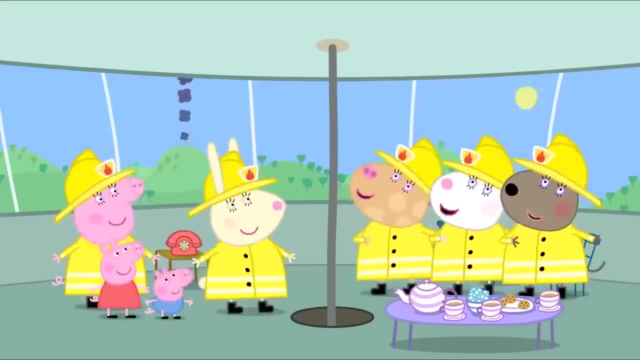 Daddy wants to speak to you. Hello Daddy Pig. Hello Daddy Pig, This phone is only to be used when there's a Fire, Fire. Oh dear Daddy Pig's barbecue is on fire. Fire, Fire. Mummies to the rescue. 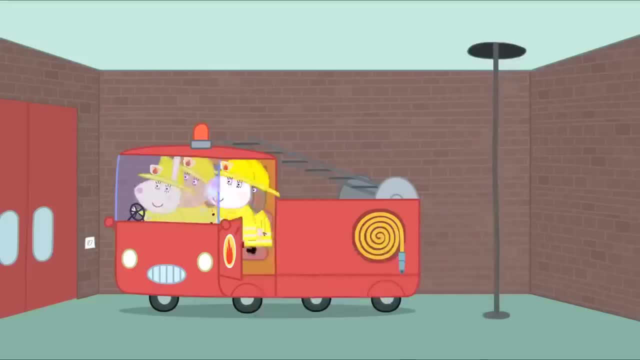 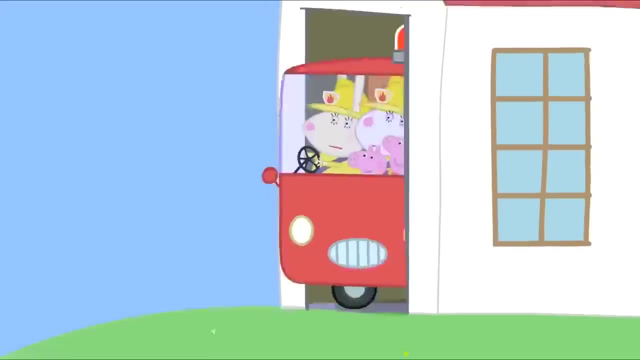 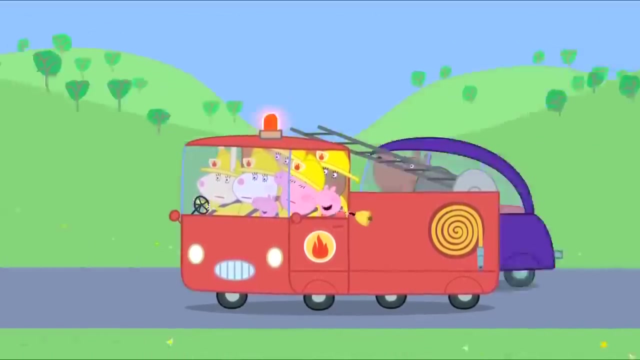 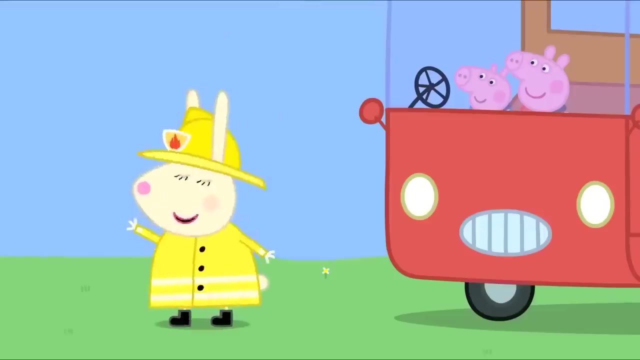 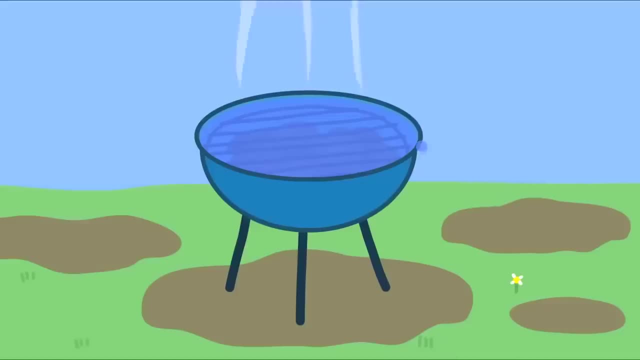 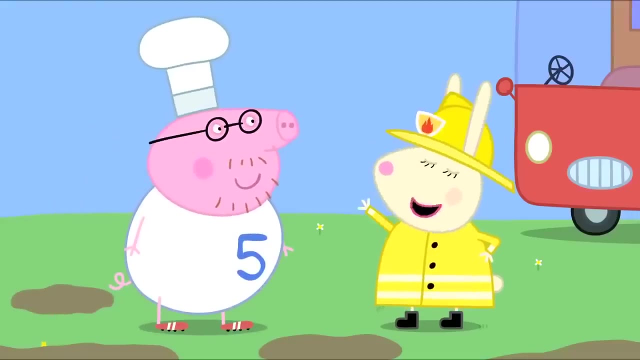 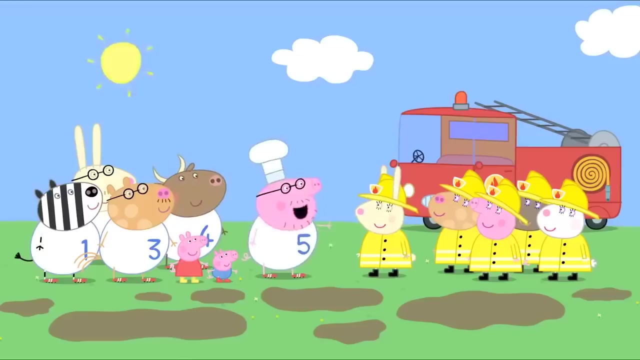 Stand back, Daddies. Mummy Dog, Turn on the water. Aye, aye, Mummy Pig, The fire is out. Hooray, Thank you for saving us, Miss Rabbit. No problem. And now that Miss Rabbit has kindly flooded our garden, 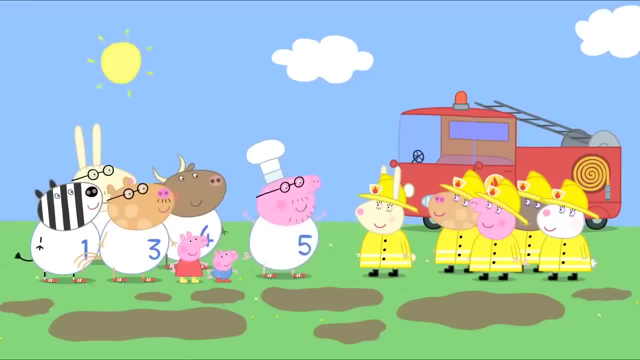 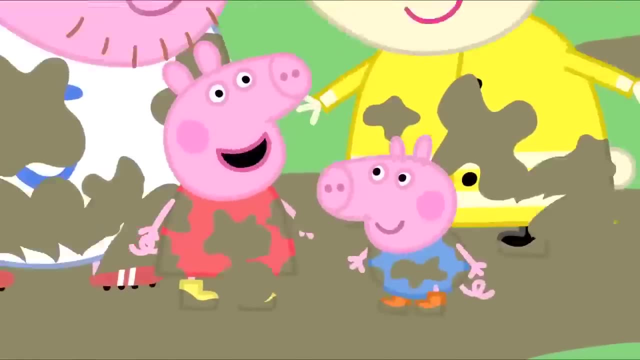 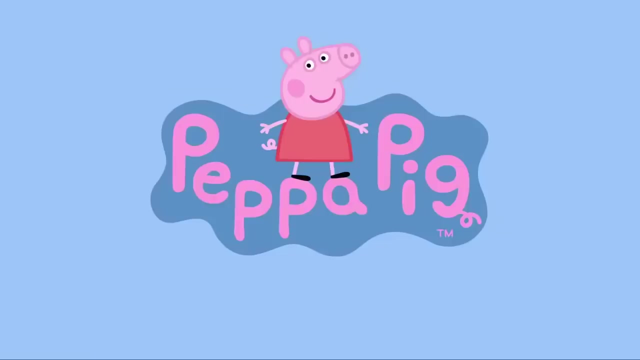 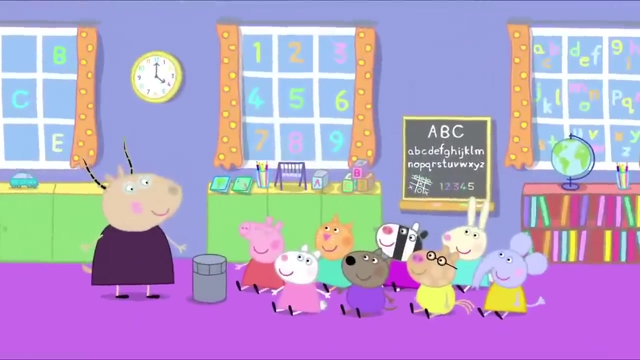 we can all jump up and down in muddy puddles. Hooray, I love fire engines, Especially when they make muddy puddles. Peppa and her friends are at their playgroup. Today we are going to make a time capsule. 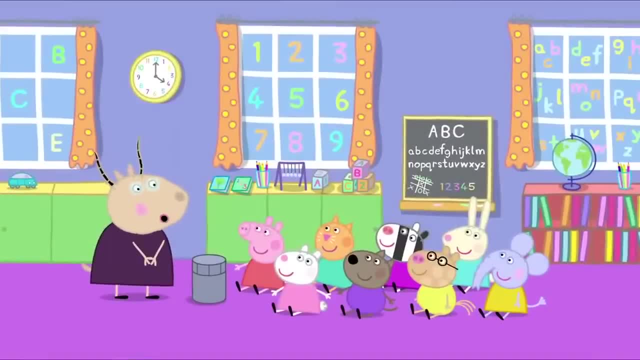 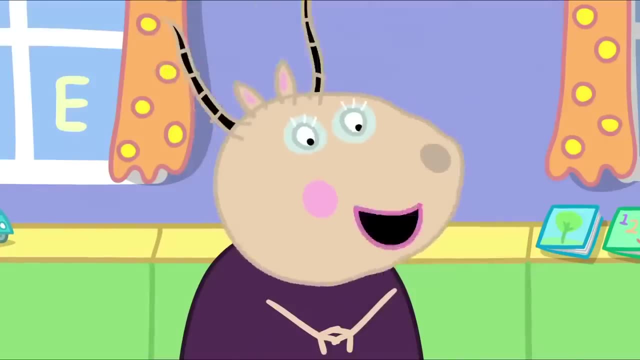 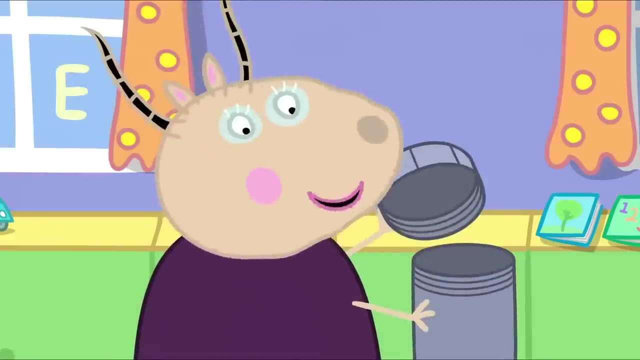 What's a time capsule? A time capsule is something that will show people in the future how we lived, How We'll put special things in this box and then we'll bury it in the school garden. Will it grow? No, Suzy. it will remain in the garden. 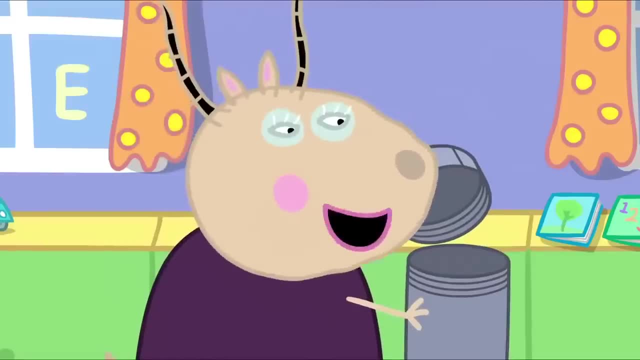 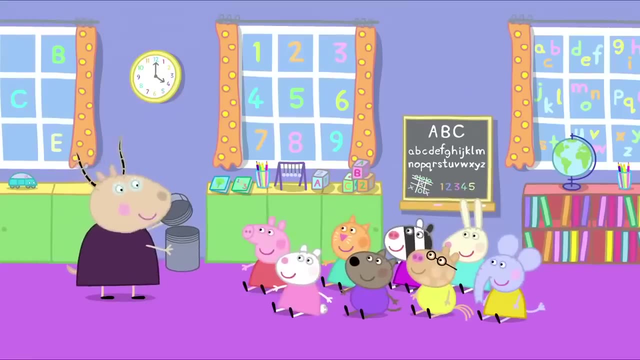 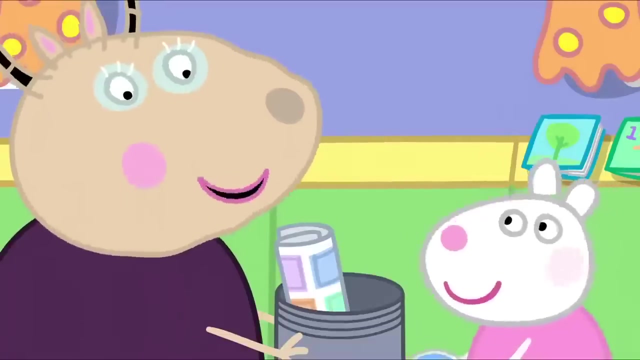 Peppa and her friends are at their playgroup, Remain in the ground for many years. Ooh Now, what things should we put inside? A comic? Very good. Peppa Music- Very good. Suzy A toy. 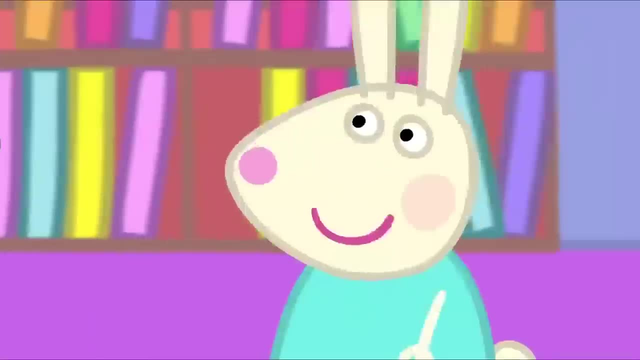 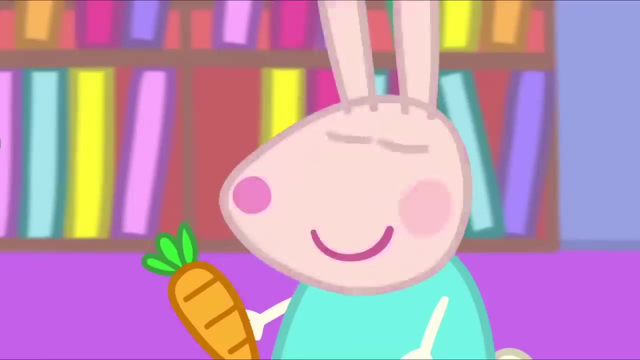 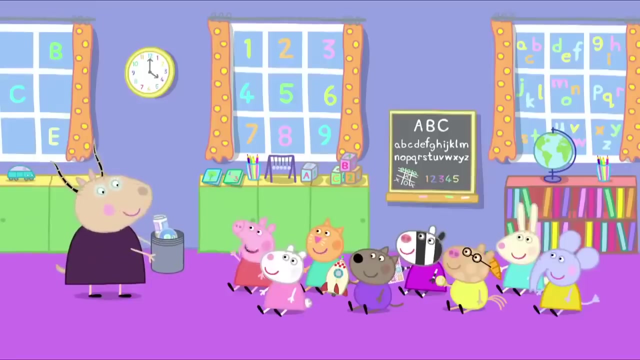 A coin Stamps A carrot. You do like carrots, don't you, Rebecca? Yes, All those are excellent things to show our daily lives. Madam Gazelle, what will the future be like? What do you think it will be like? 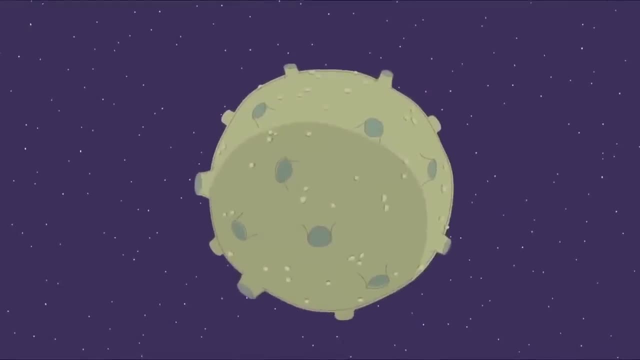 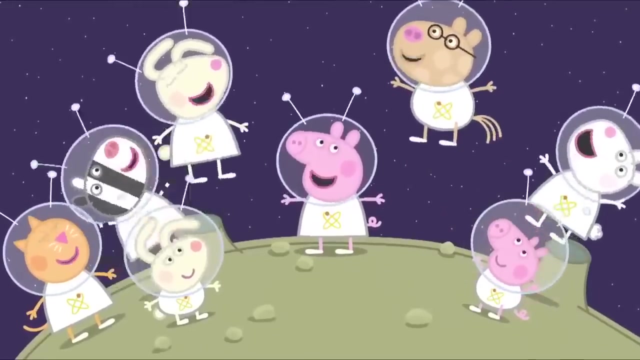 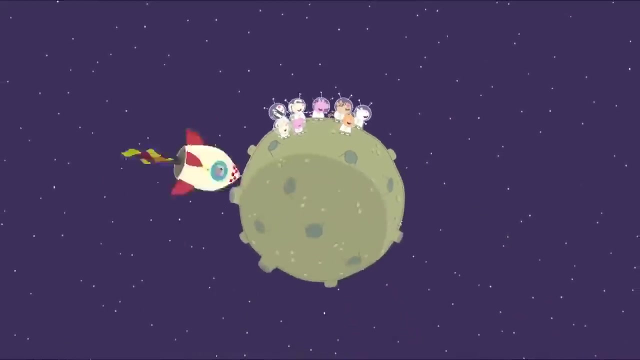 I think in the future I will live on the moon And all my friends will come to visit And I will fly a space rocket. Hello Now. we'll record a message for the people of the future. Say hello to the future. 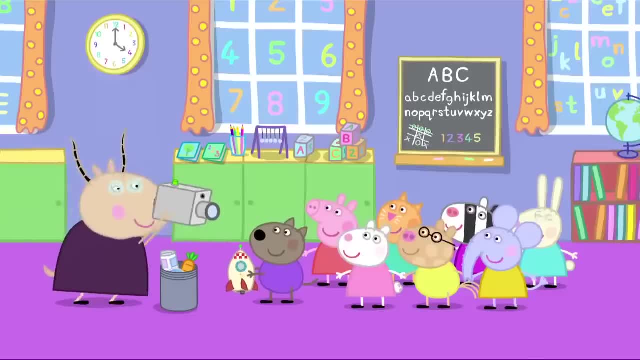 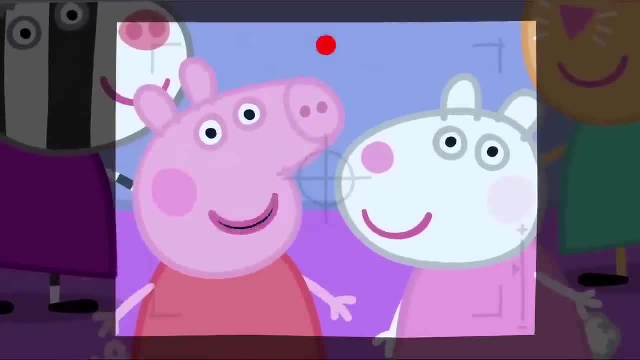 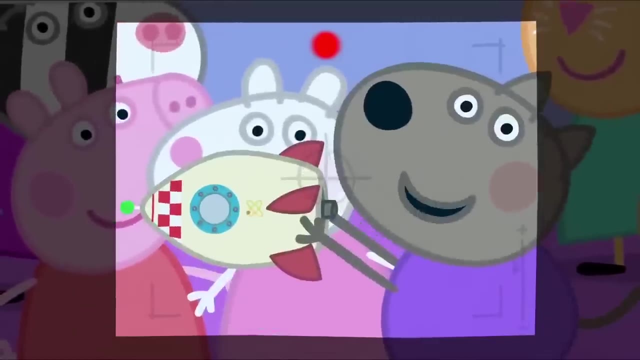 Hello to the future. You're probably all living on the moon now And going on holiday to Mars And flying around in space rockets- Wonderful, Now what will the future be like? Wonderful, It is nearly home time and all the parents have arrived. 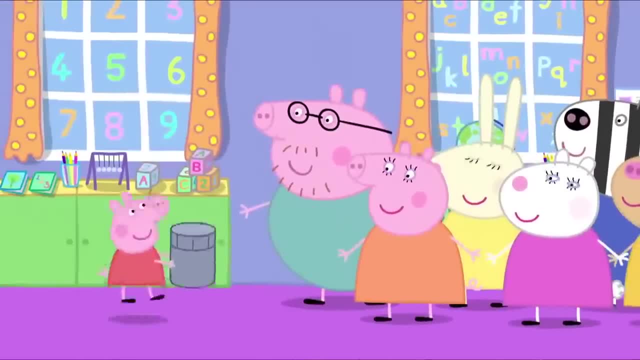 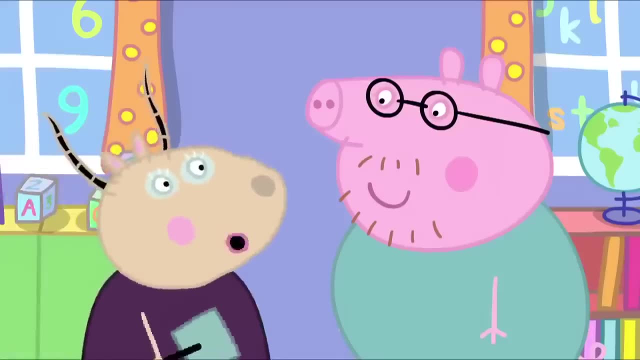 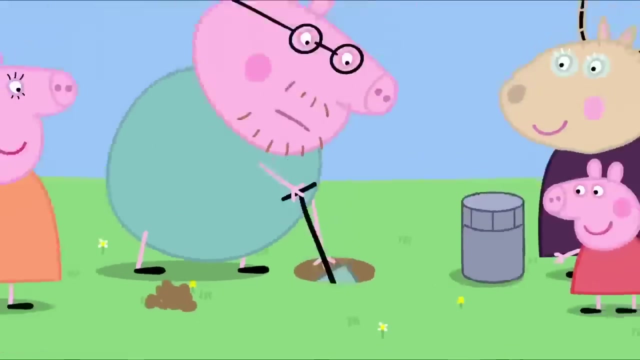 Mummy, Daddy, we've made a time capsule. Ah, Daddy Pig, you're just in time to help us dig a hole. Yes, of course Daddy Pig is digging a hole in the school garden for the time capsule. He's digging a hole in the school garden for the time capsule. 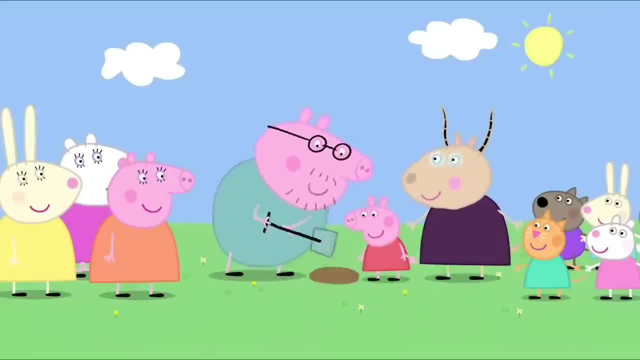 He's digging a hole in the school garden for the time capsule. He's digging a hole in the school garden for the time capsule. There, Can we dig it up now? Ha-ha, It will remain in the ground for many years. 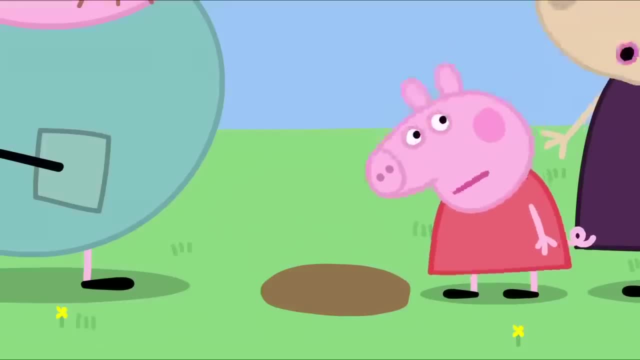 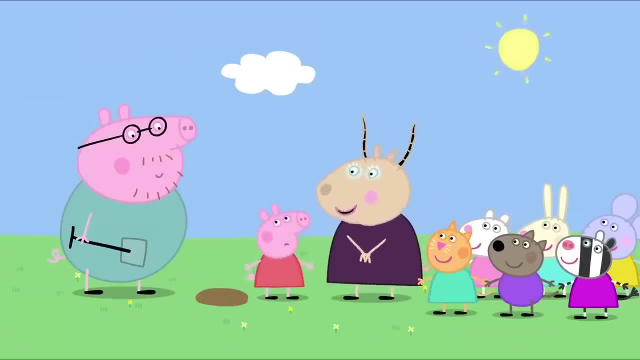 Aw, but I can't wait that long. Peppa, you are just like your Daddy when he was little, Am I? Yes, I remember when I was his teacher. Did you teach my Daddy? Yes, I taught all of your mummies and daddies. 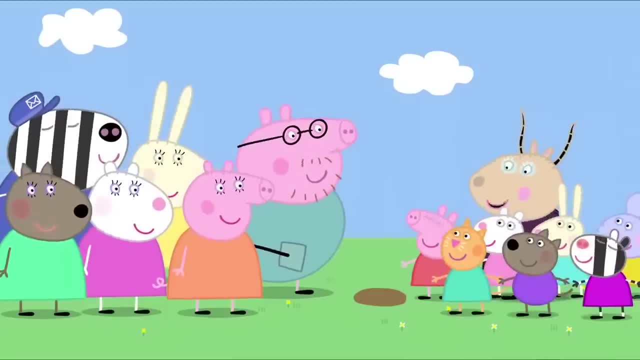 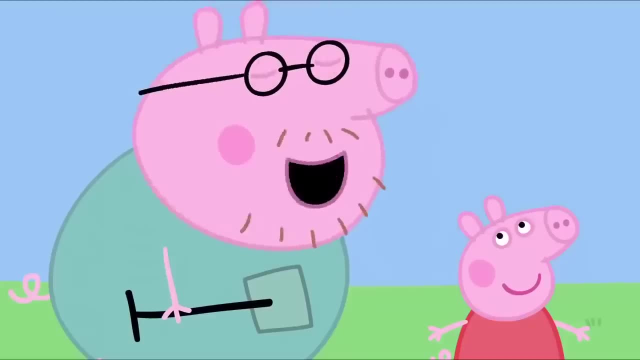 Didn't I? Yes, Mademoiselle, When your mummies and daddies were little, they made a time capsule too. Yes, we did. We buried it next to a little tree. Can we dig it up? Yes, I think we buried it over here. 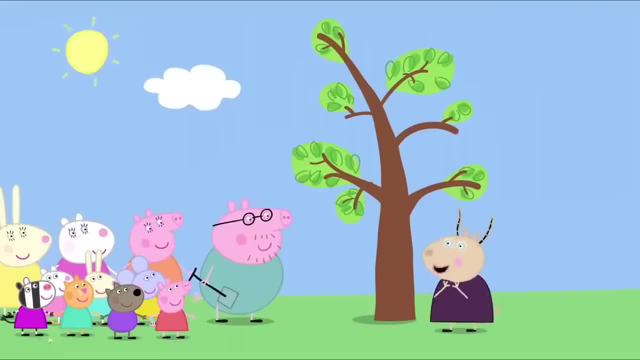 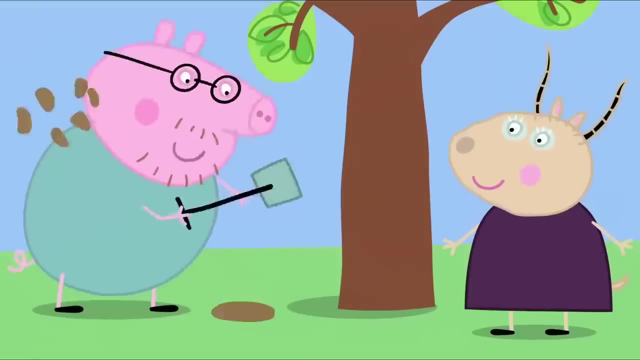 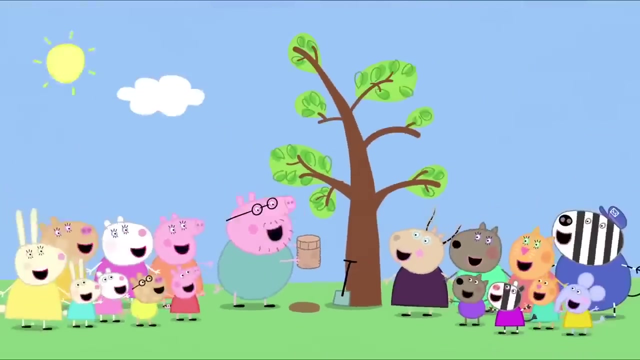 Oh, I thought it was a much smaller tree. Oh, it was a long time ago. The tree has grown a bit since then. I've found something. It's our old time capsule. Our old time capsule, Hooray. I can't wait to open it. 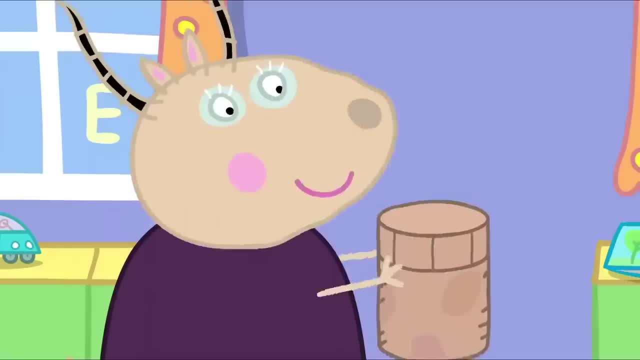 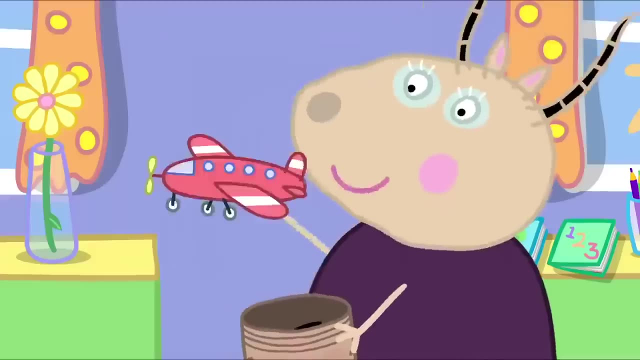 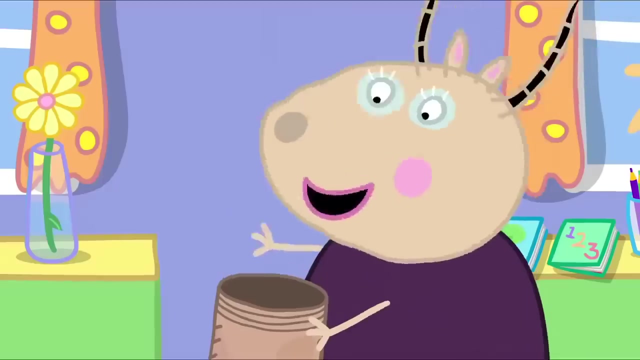 Stand back, children. Yes, Mademoiselle, What do we have here? Oh, an old comic- That was my favourite comic- A tin toy, My favourite toy, Music, My favourite record And a very old carrot That's mine. 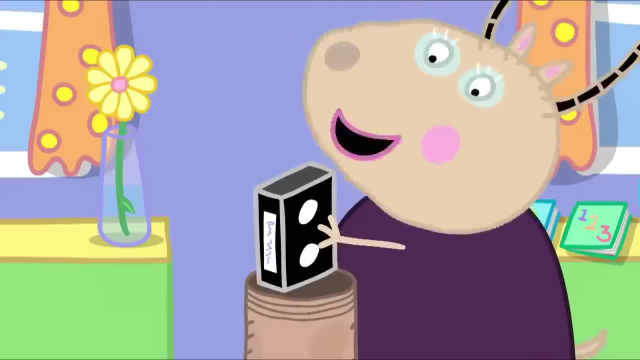 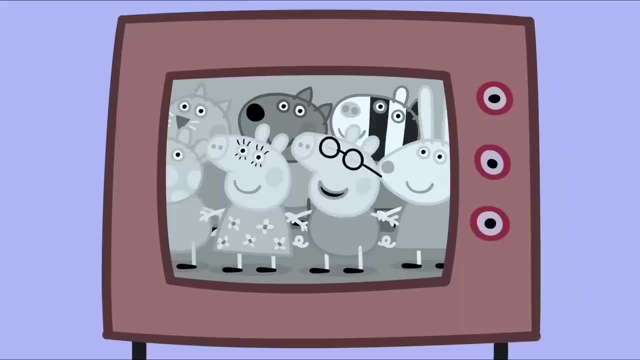 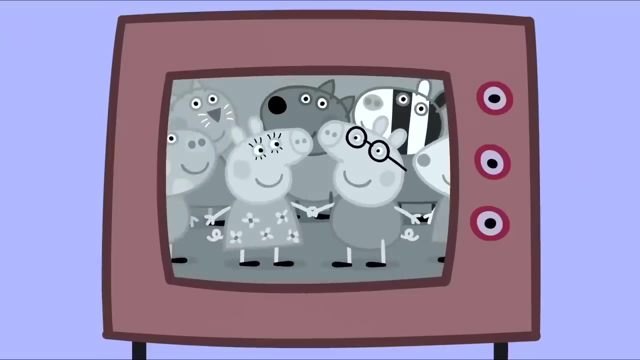 What a good choice, Mummy. Oh, and a videotape of your mummies and daddies when they were little. Ooh, Who's the little piggy in the glasses? Oh, that's Daddy Pig. Oh, and that's me. 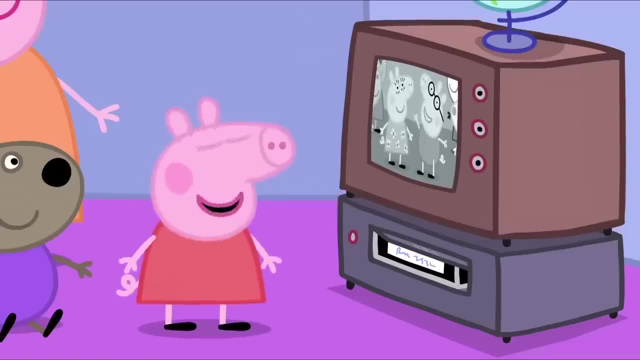 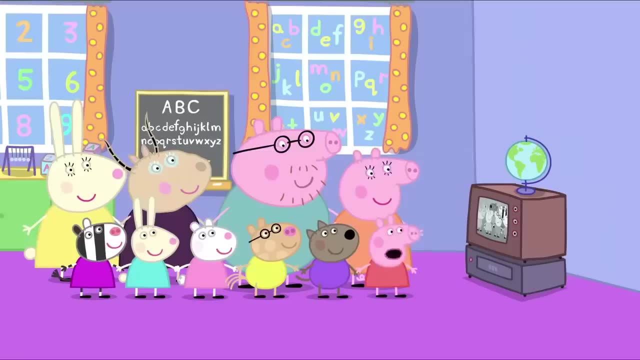 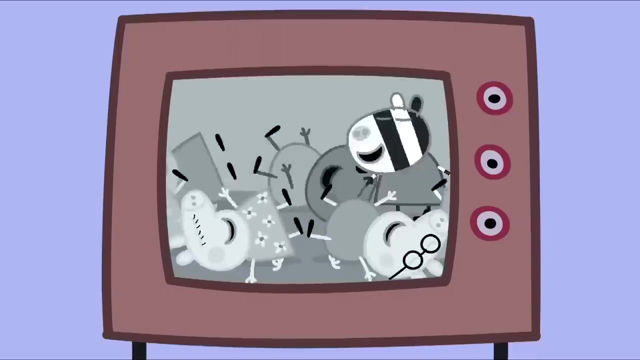 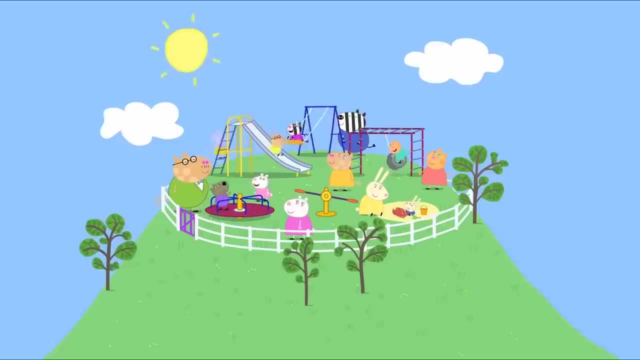 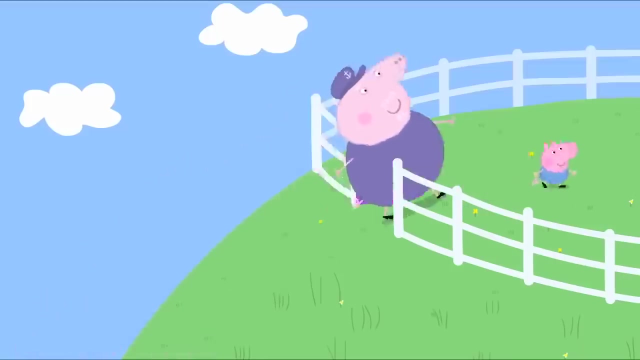 Hello to the future. What a squeaky voice you have. You're probably living on the moon now. Silly little Daddy Pig. Making time capsules is such fun And finding them is even better. Grandpa at the playground. Grandpa Pig is looking after Peppa and George today. 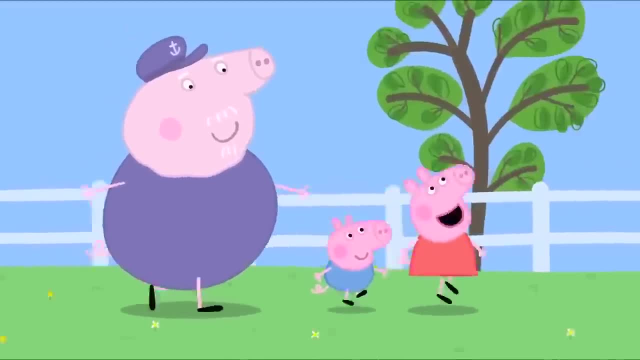 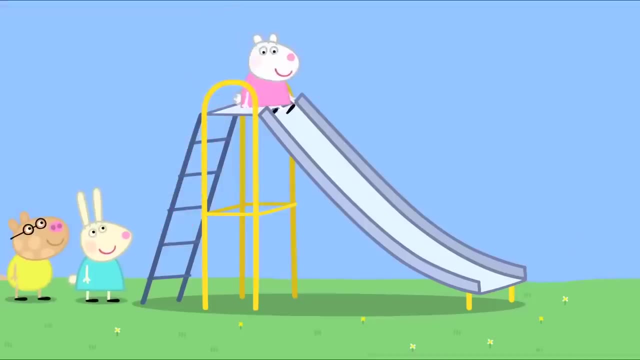 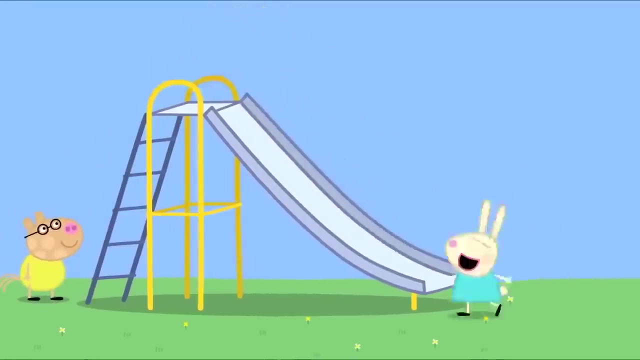 Now, Grandpa, I will tell you how everything works. This is the slide. You climb up here and you slide down there, Whee, Whee, And everyone takes it in turns. Ho, ho, I know what a slide is, Peppa. 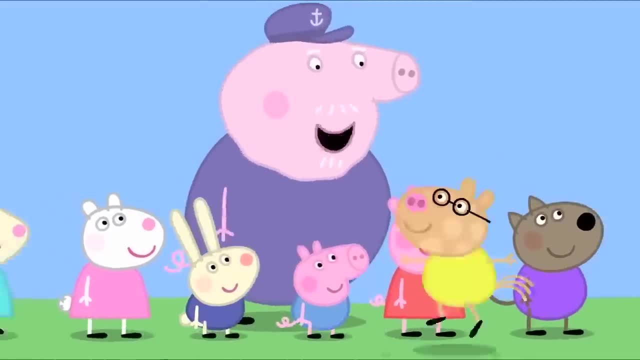 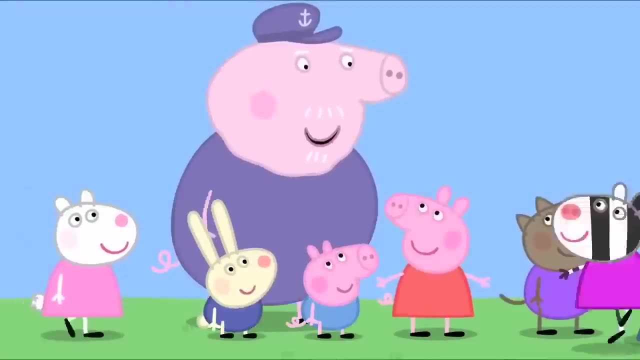 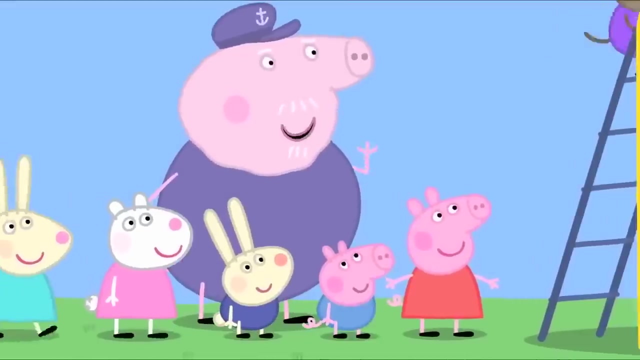 I used to play on one myself when I was a little piggy. Did you have swings too in the olden days? Ho ho, we had swings and climbing frames and roundabouts. Ooh, But my favourite was the slide. It is my favourite too. 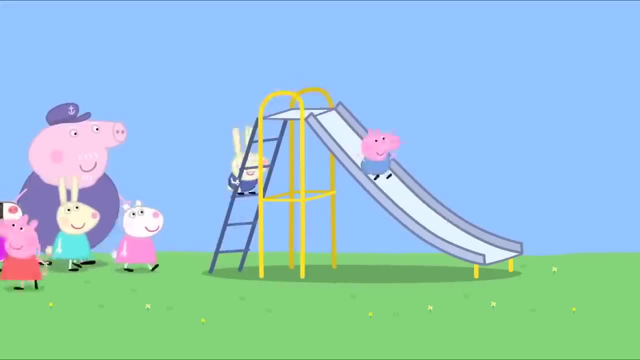 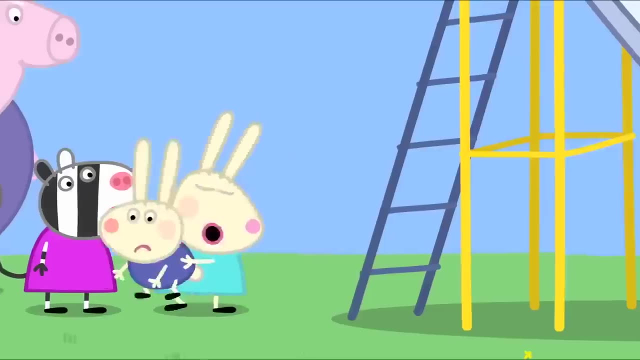 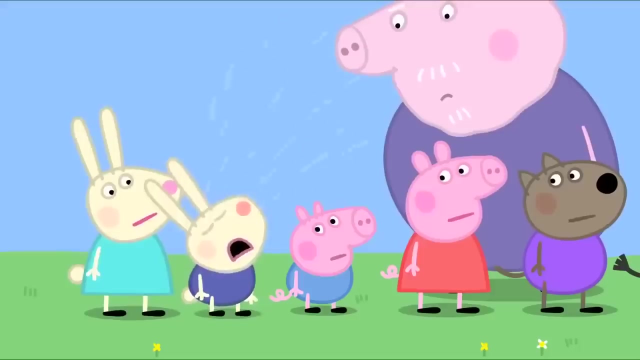 Whee, Everyone takes it in turns to have a go on the slide. Whee, Naughty Richard, You know you have to wait your turn. Richard Rabbit finds it hard to wait his turn. Whee, Oh dear. It's not easy being small, is it Richard? 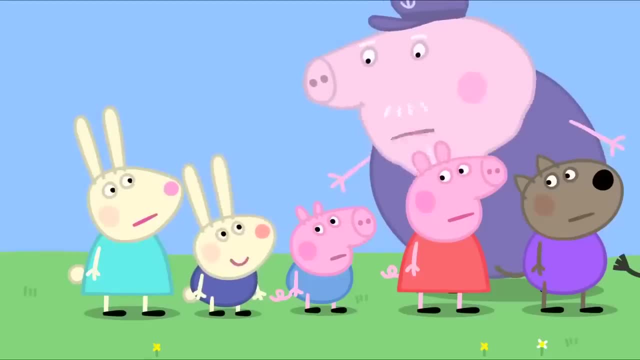 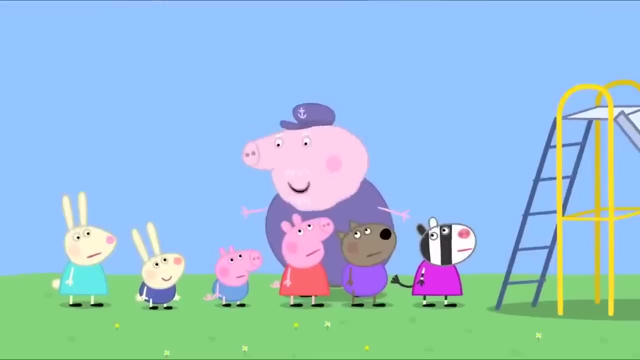 Because Richard is little. I don't think he should have to wait. I wouldn't change the rule. I wouldn't change the rules if I were you. Grandpa Peg. Nonsense, The children understand, don't you? Ha ha ha. 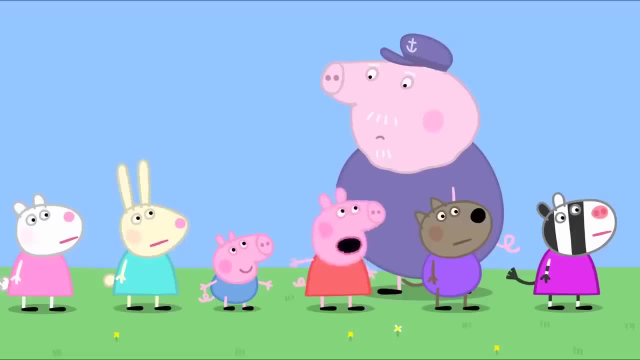 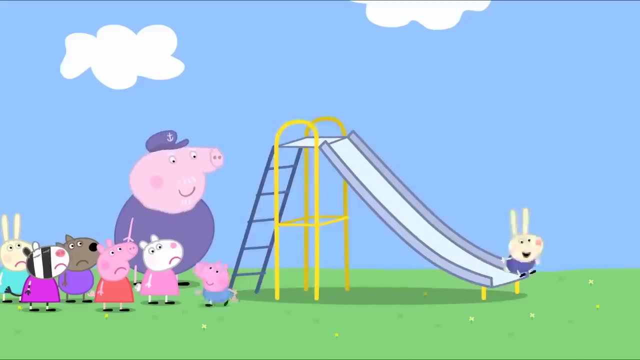 Whee, But Grandpa George is little and he has to wait his turn. Whee, Yes, George is little, so he shouldn't have to wait either. Whee, Ha, ha, ha, Whee, Oh dear. 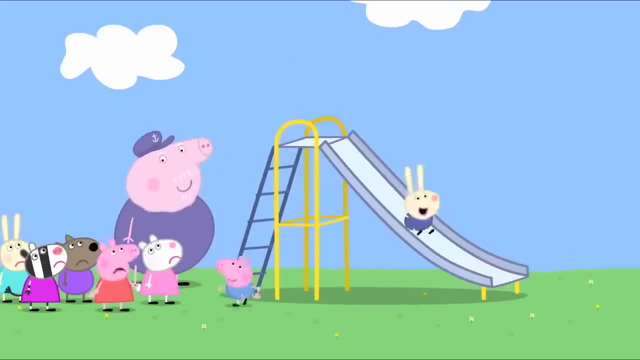 He has to wait all the turns on the slide. Grandpa, when do we get to go on the slide? Don't worry, Peppa, They won't be on it for long. I'm bored of waiting, Me too. Let's play on the swing. 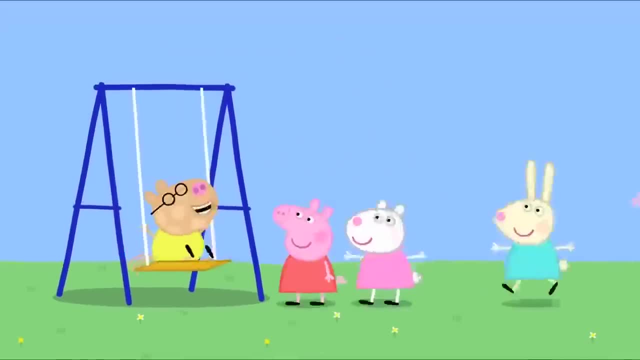 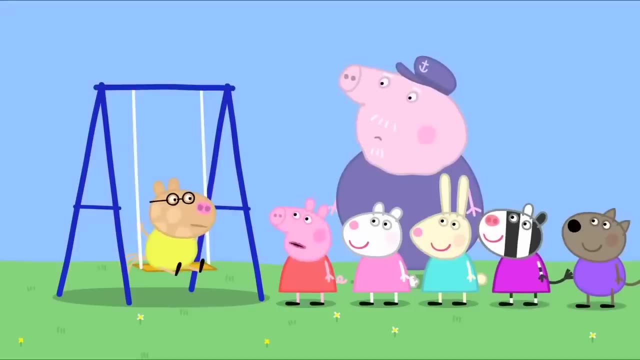 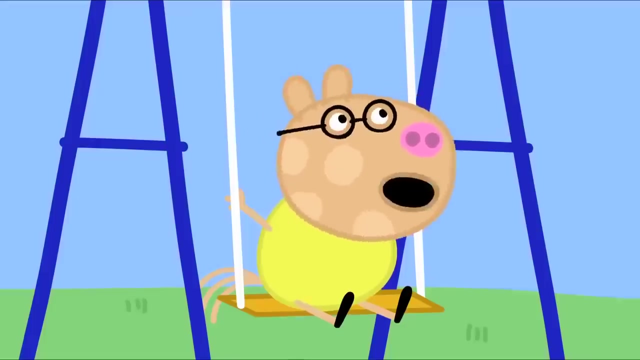 Ha ha ha. Here is Pedro Pony on the swing. No, Pedro, can I have a go now? I just want to swing a bit more, But you've been on the swing for ages. Grandpa Pig, can you push me a little bit please? 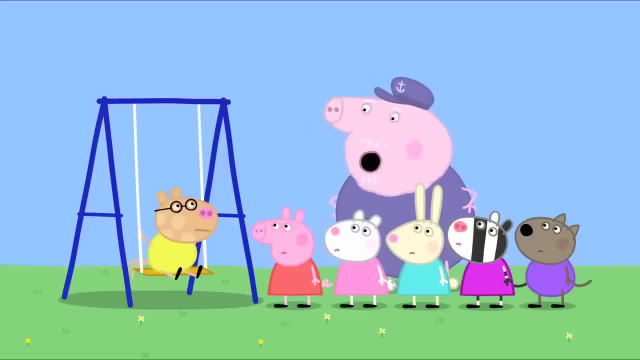 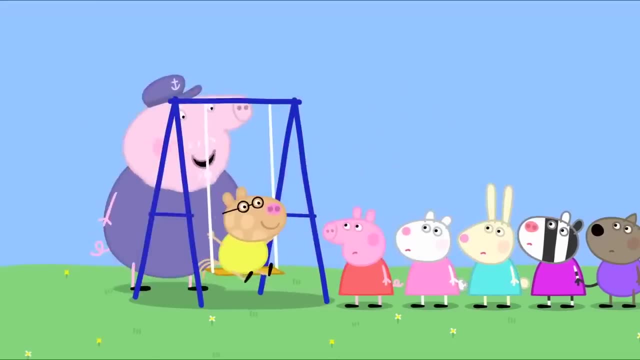 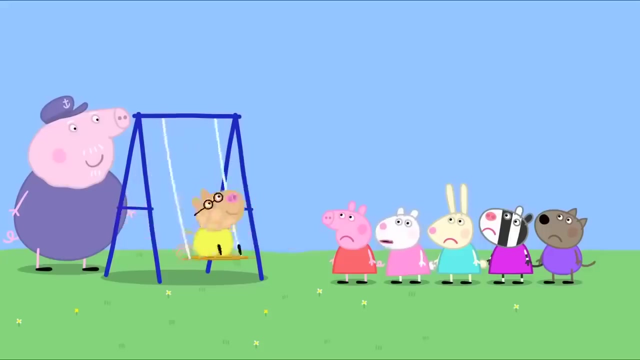 I think it is someone else's turn now, Pedro, But I have to go home soon. Oh, I see That's different. Let me push you then, But, Grandpa, Ha ha ha, I'm bored of waiting. 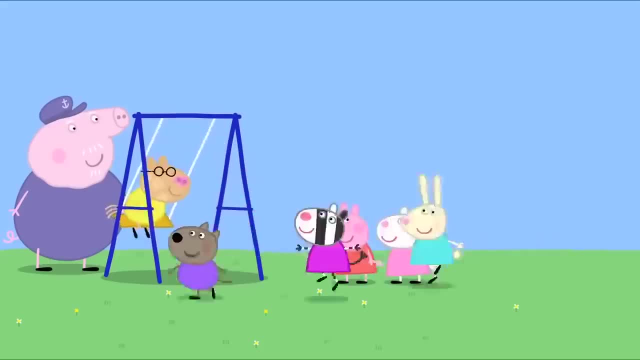 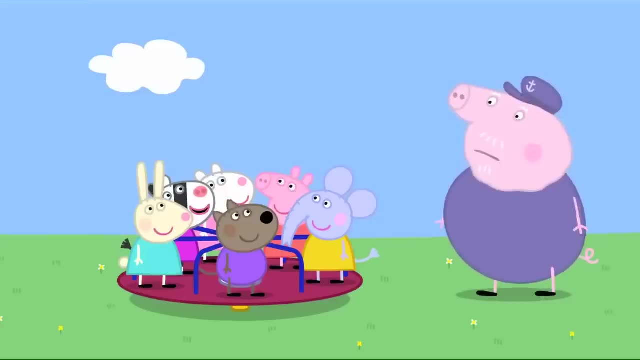 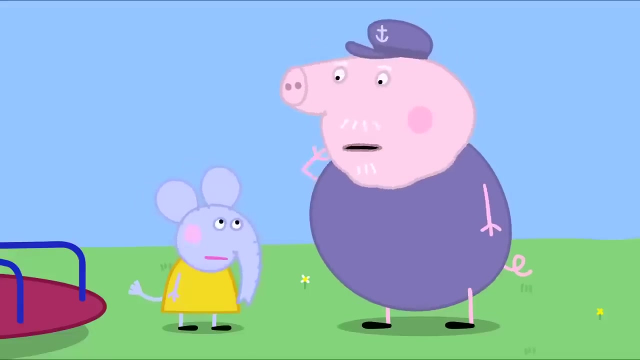 Me too, And me. Let's play on the roundabout. Everyone wants to get on the roundabout. Too many children on the roundabout, Everybody off But Grandpa Pig. I was actually here first. Ah, then you can get back on the roundabout. 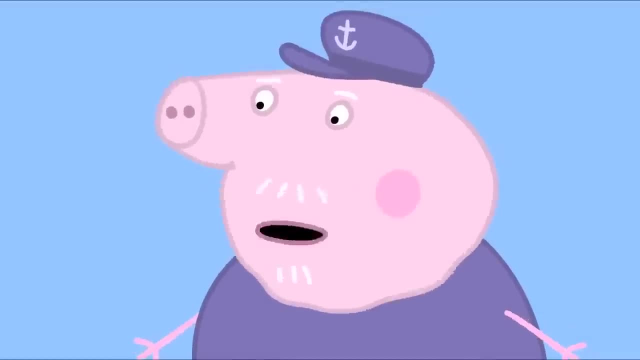 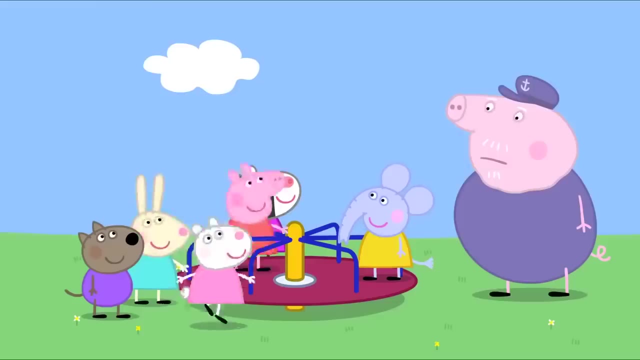 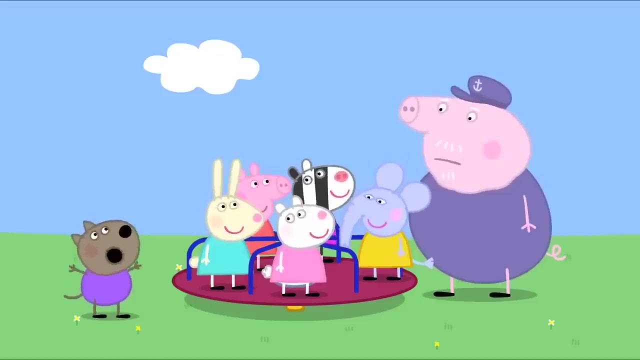 I need to get on too. Why is that, Rebecca? Um, because it's my birthday soon, Oh, okay. And me? Oh, all right. Is everybody ready? Yes, Stop. There are no boys on the roundabout. 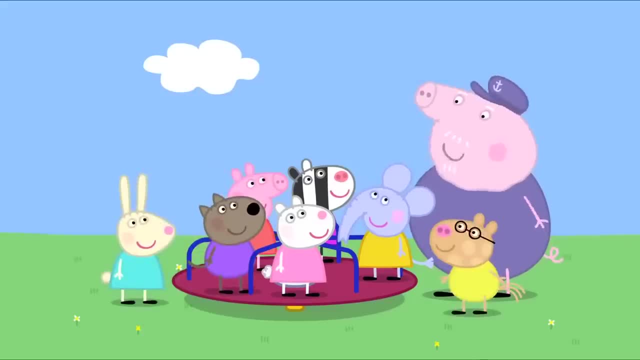 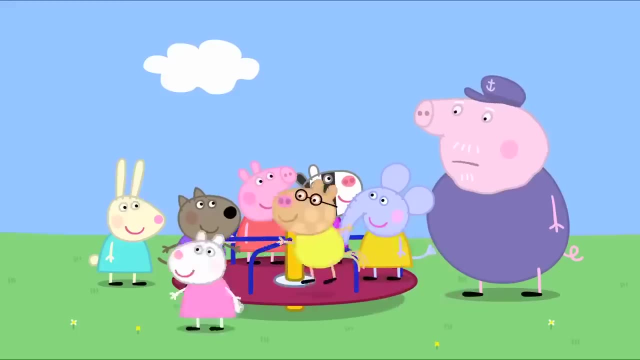 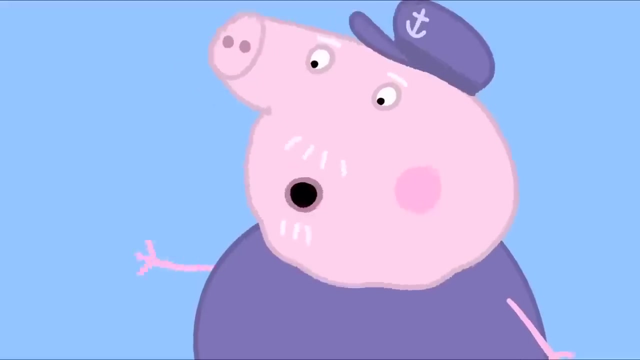 Um, Now is everybody ready? I'm wearing glasses. Can I go on, please? The children are making up their own rules. I need to get on because I like carrots. Now are you all ready to go? No, I have to get on because I can do this. 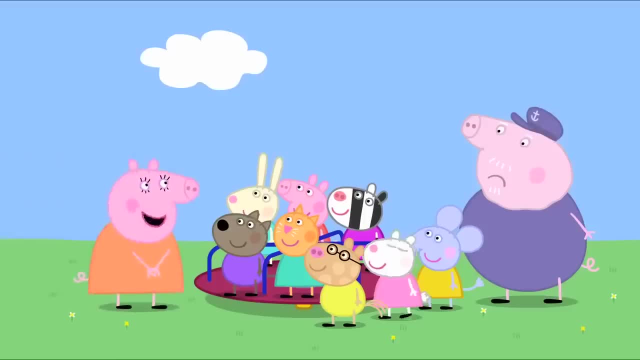 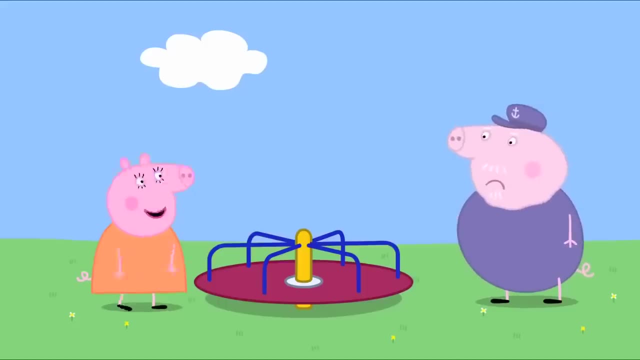 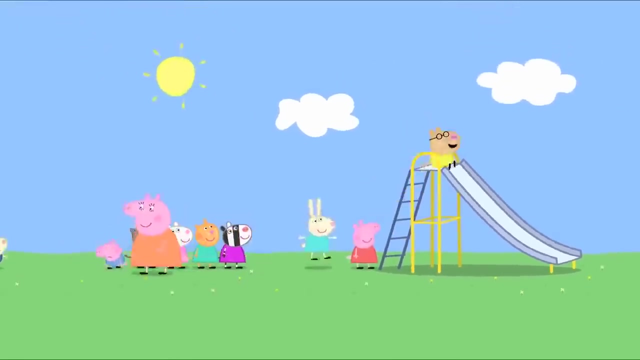 Here is Mummy Pig. How are you getting on, Grandpa Pig? I'm confused. These playground rules are too complicated. There is only one rule, Grandpa Pig, and that is. everyone waits their turn. Whee, What, Even the little ones. 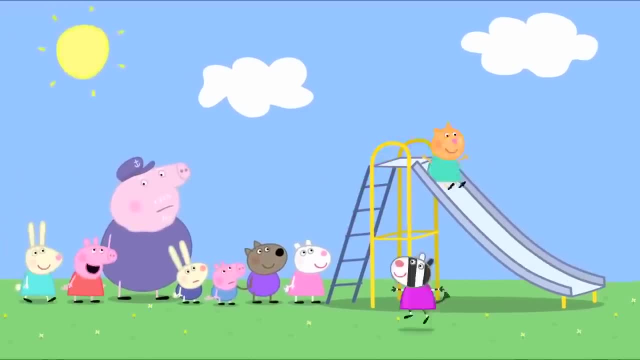 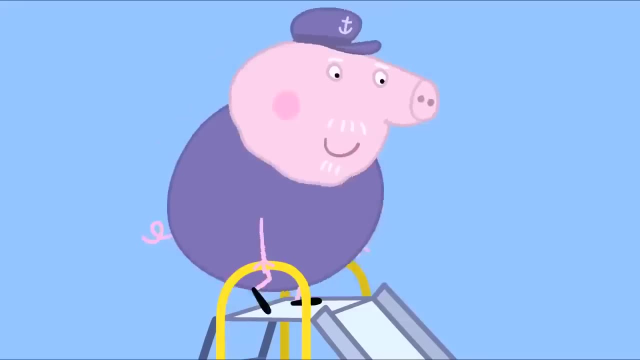 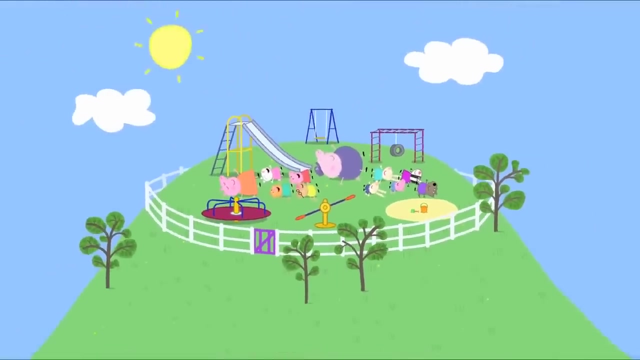 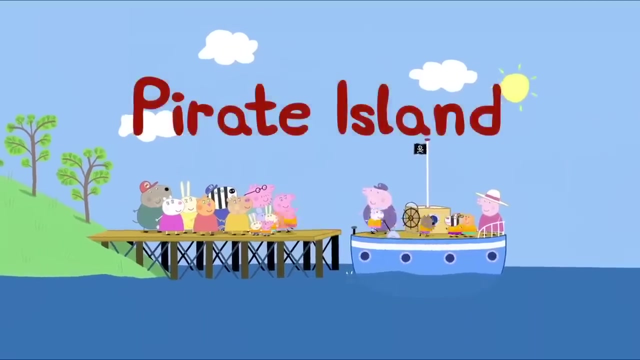 Even the little ones? What about the very old ones like Grandpa? Even the very old ones like Grandpa? At the playground, everyone has their turn. Whee, Pirate Island. Grandpa Pig is taking Peppa and her friends for a day out on his boat. 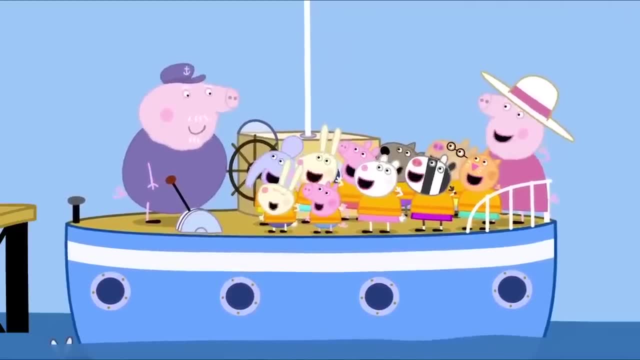 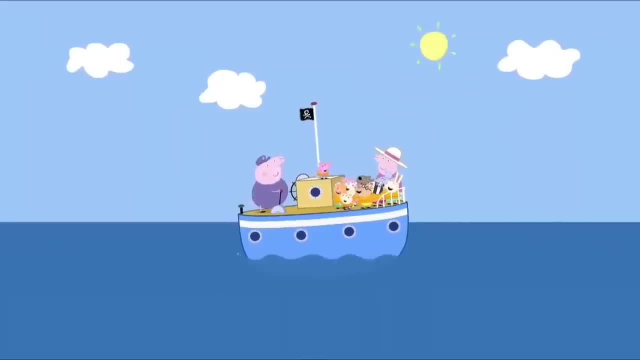 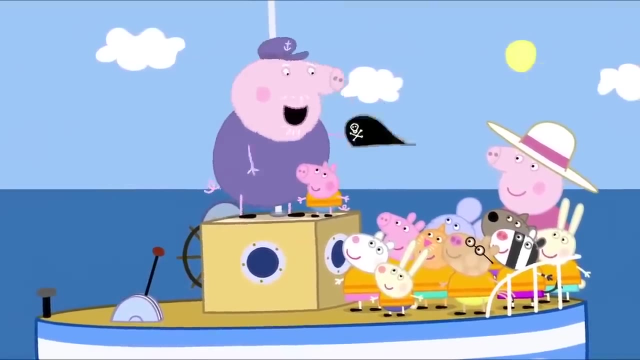 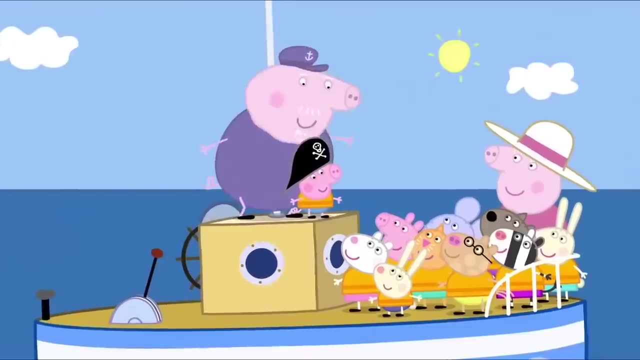 Everyone on board. Aye, aye, Captain, Grandpa Fools, See you later, See you later, See you later. Peppa and her friends are all wearing life jackets. George, you could wear my pirate hat. Today we are sailing to Pirate Island. 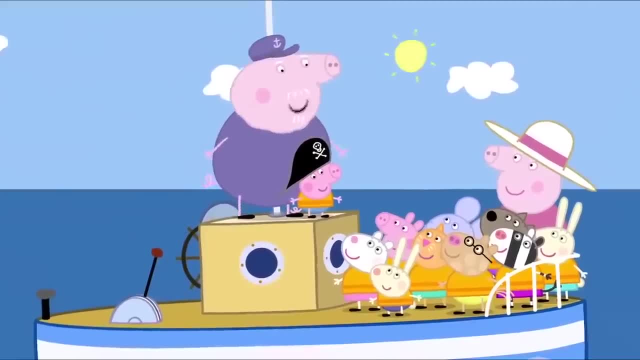 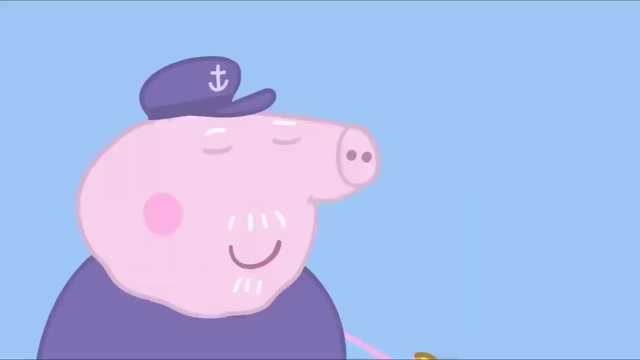 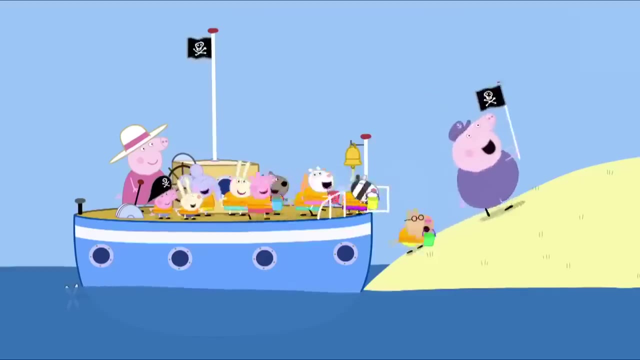 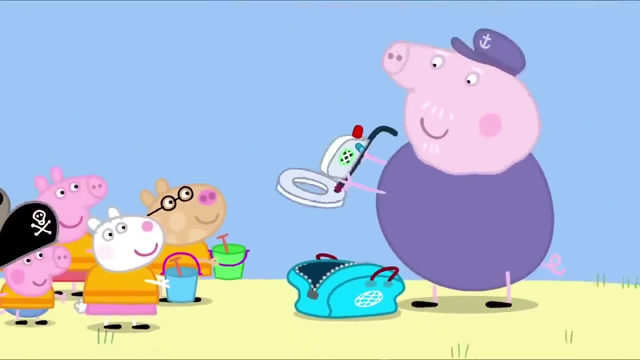 Ooh, If we're lucky, we might find buried treasure. Wow, Pirate Island sounds like a name for a pirate island. It sounds like a great place, Land ahoy, Here we are. Pirate Island, Hooray, What's that? 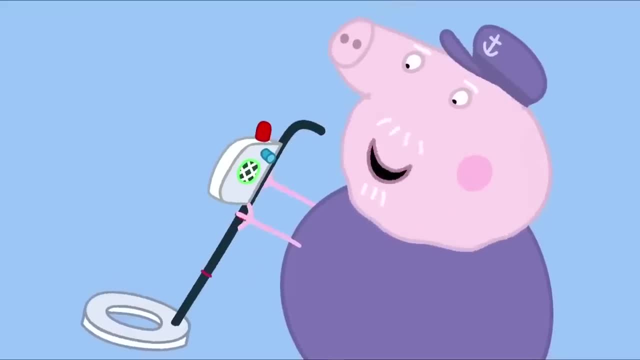 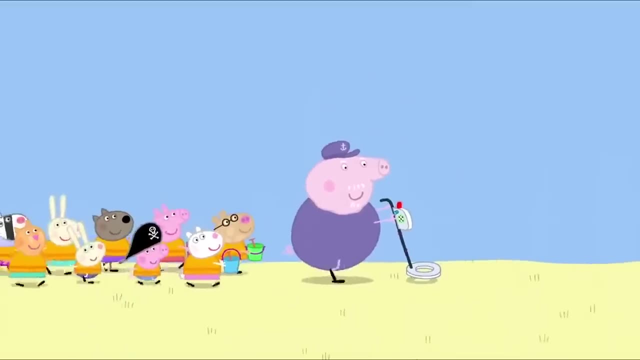 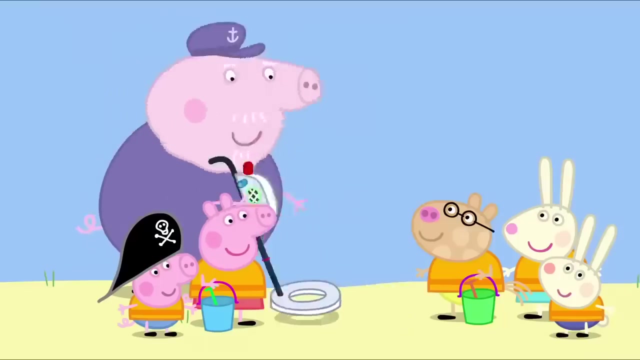 It's a metal detector. It finds buried treasure. Ooh, Grandpa Pig is using the metal detector to find buried treasure. Ah-ha, The metal detector has found something. Let's dig it up. It's a little coin Treasure. 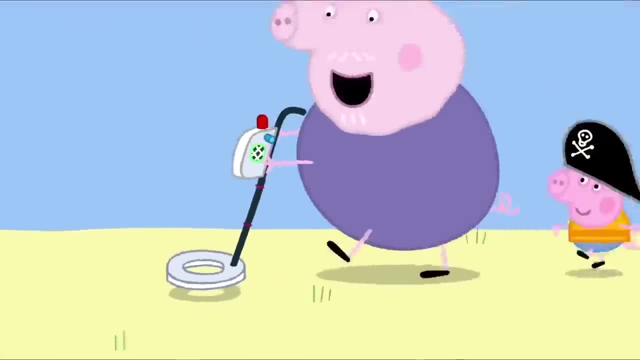 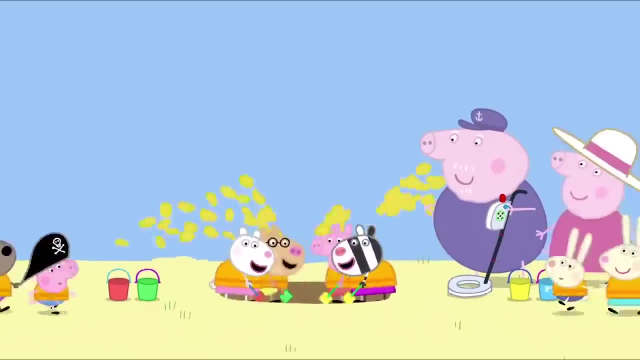 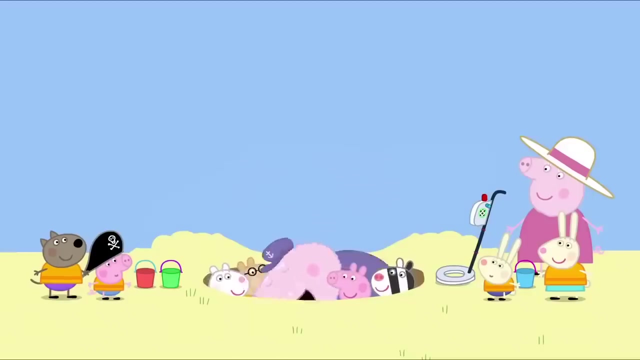 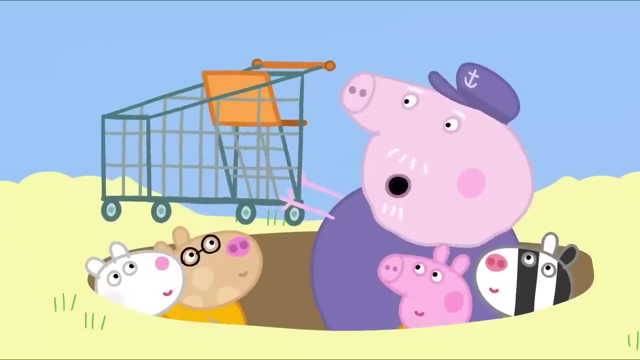 Hooray, Let's find some more. Ah-ha, We've found something else. It sounds big, My goodness. This piece of treasure is quite heavy. Oh dear, That is not buried treasure, That is a rusty old shopping trolley. 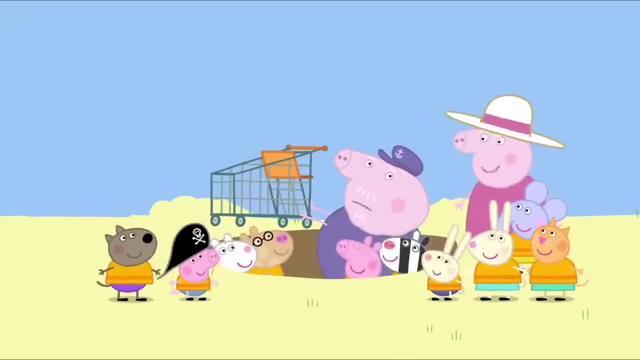 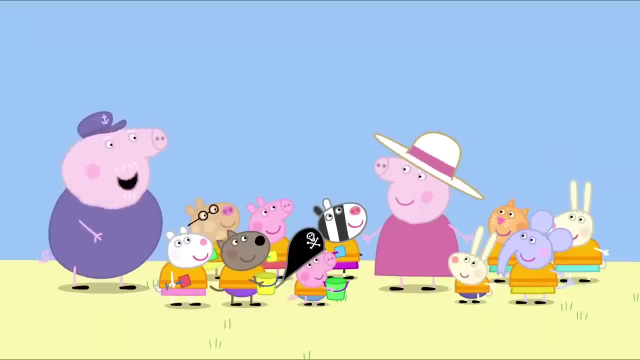 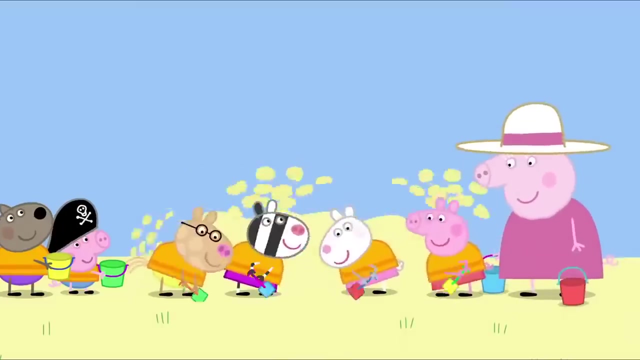 Oh, Maybe that's enough treasure hunting. Who wants to help build a big sandcastle Me? What a good idea, Granny Pig. I'll just check on the boat. Granny Pig is going to help the children build a big sandcastle. 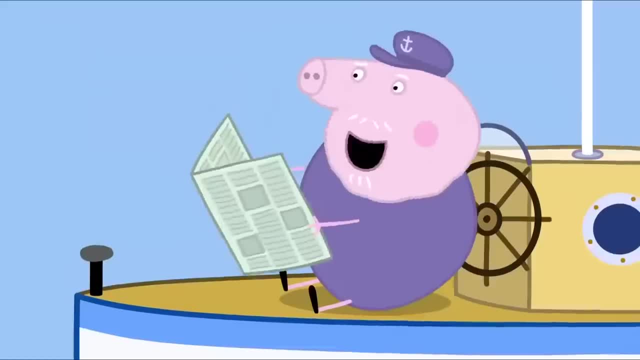 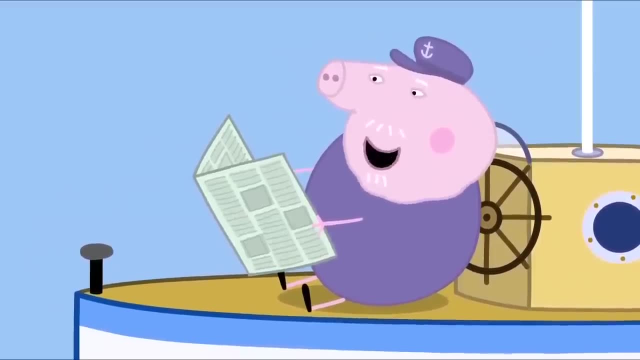 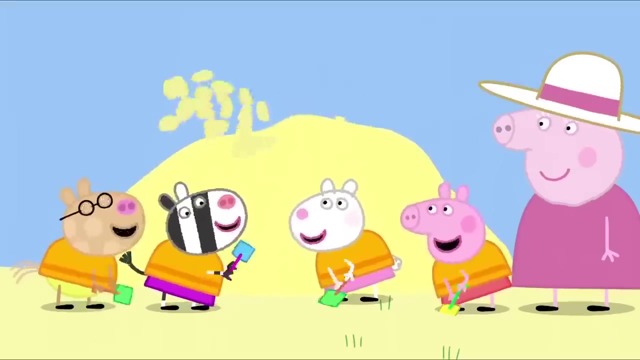 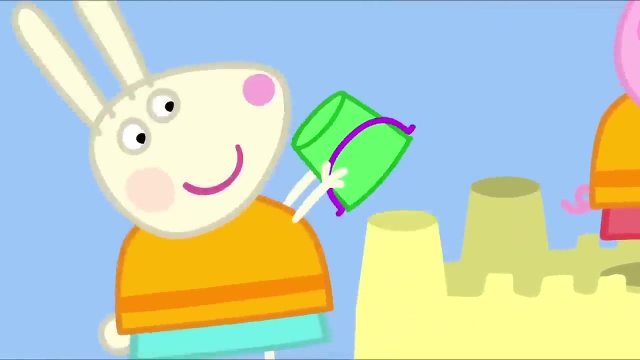 And Grandpa Pig is doing important boat things. Ah, this is nice. Oh, Maybe I'll just close my eyes for a little bit. Granny and the children are making a big sandcastle. They need lots and lots of sand. They use buckets to make the castle's turrets. 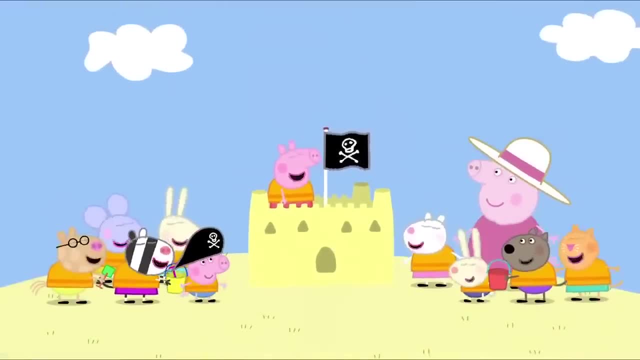 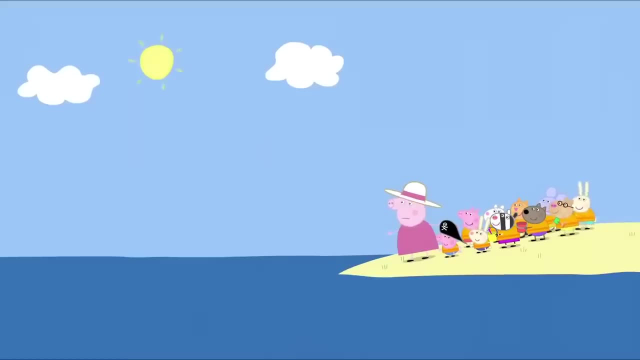 What a splendid castle. Hooray, Hooray, Hooray, It's time to go home. Oh, where's the boat gone? Look, Granny. Oh no, Grandpa Pig is fast asleep and the boat is drifting away. 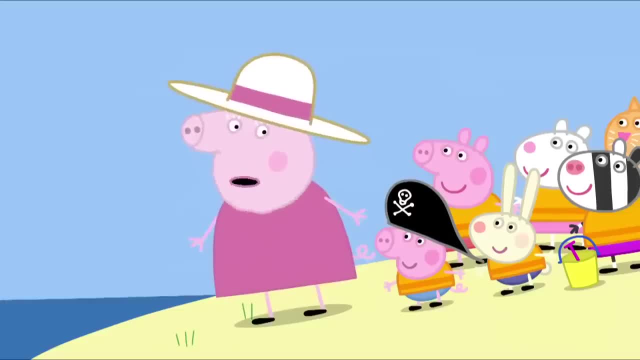 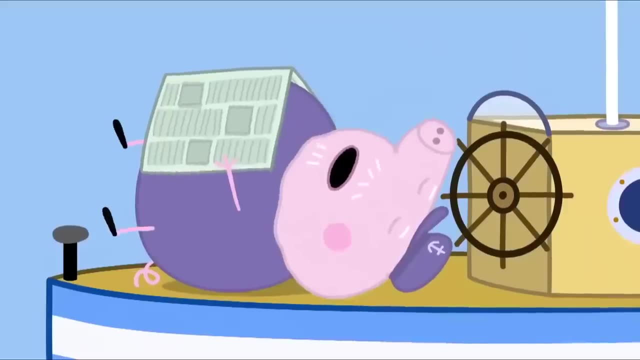 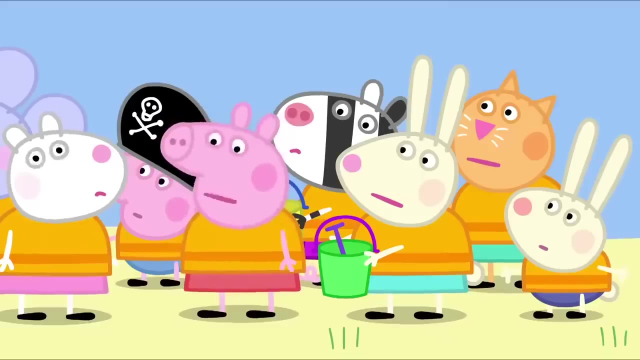 We have to wake Grandpa up. Shout as loudly as you can: Grandpa Pig, Wake up, Wake up. Oh no, Grandpa Pig is still asleep. Grandpa's too far away to hear us. Pfft, We're stuck on Pirate Island. 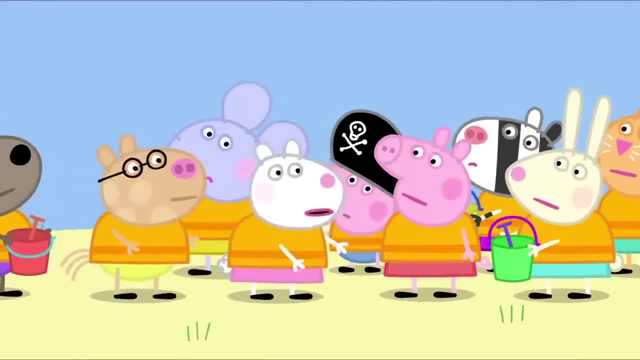 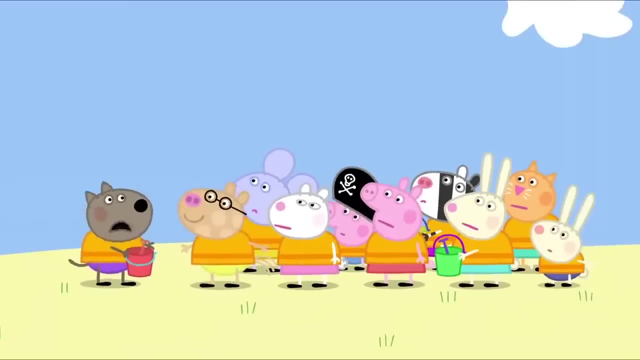 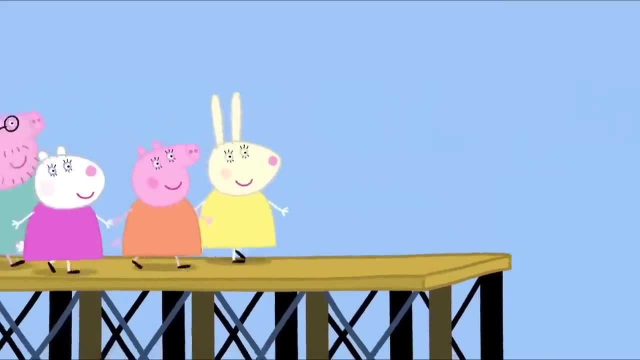 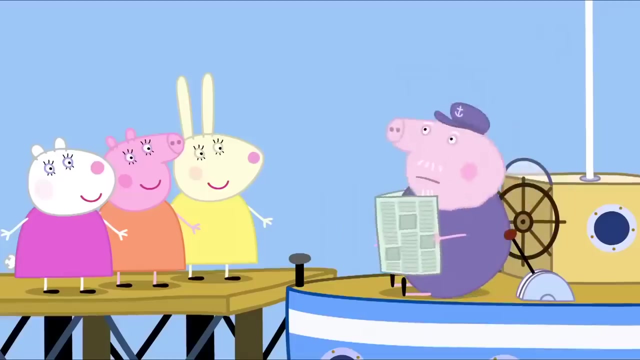 We're cast away. Meh, We'll be here for a hundred years. We'll have to eat wild fruit and berries, And we'll have to eat insects and slugs. Eww, The parents are here to collect the children. Oh, where am I? 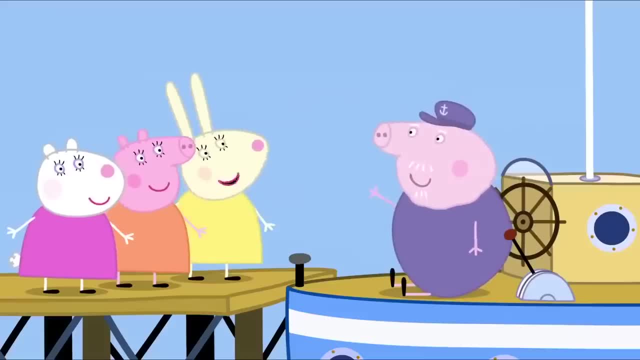 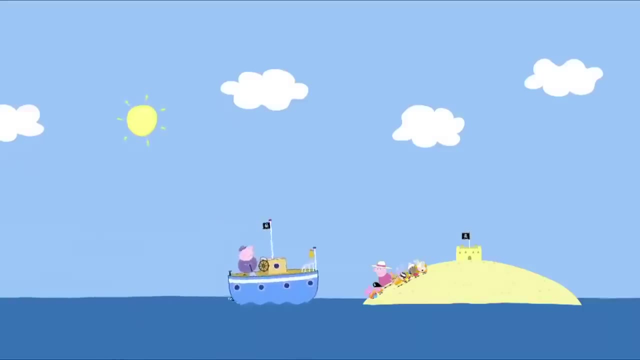 Hello, Uh, hello everyone. Have you had a nice time? Yes, Uh, actually I just left something behind Back in a tick. Look There's Grandpa, We're saved. Hooray, Welcome aboard me hearties. 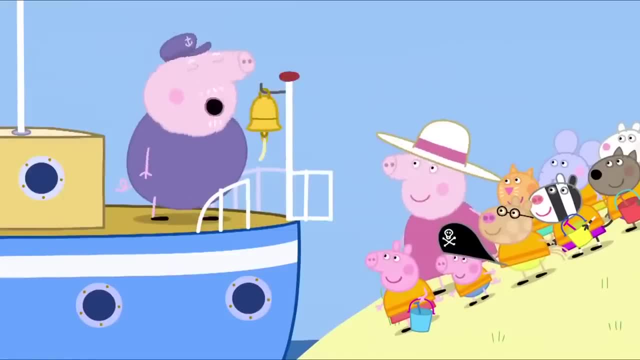 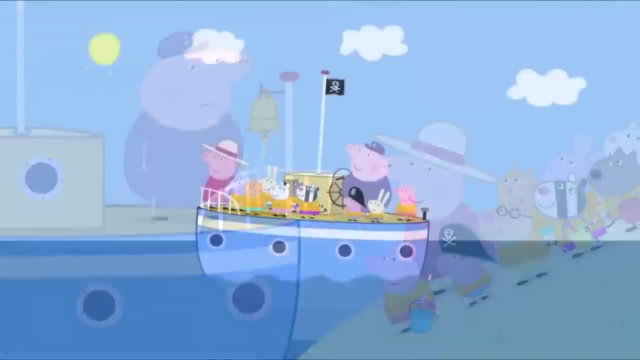 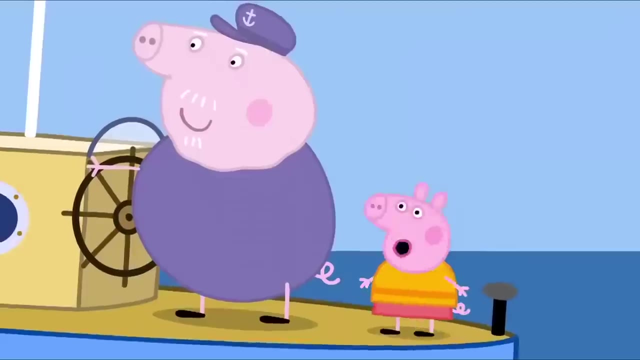 Naughty Grandpa Pig. We thought you'd left us behind. Sorry about that, Granny Pig. Next time I promise not to fall asleep. HE CHUCKLES. Goodbye, Pirate Island. See you again soon. I love Pirate Island. Can we visit it again? 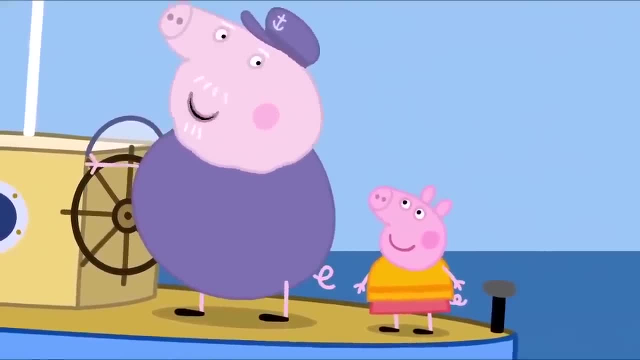 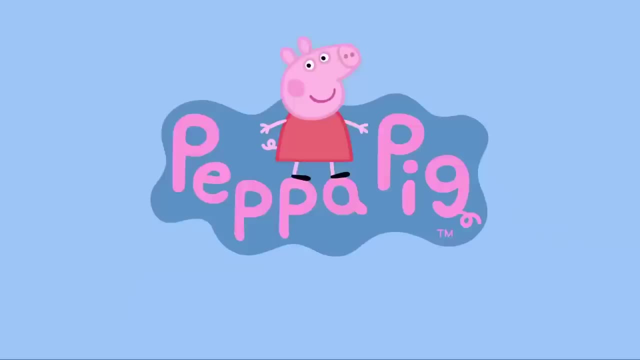 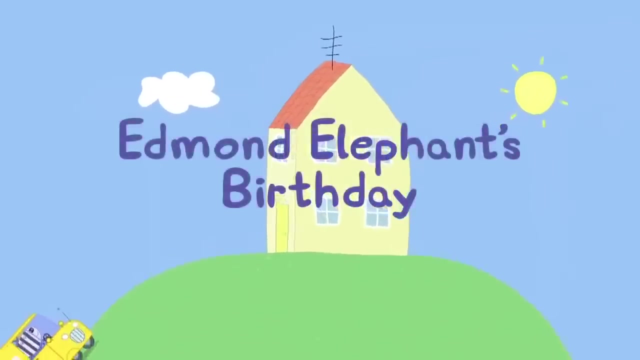 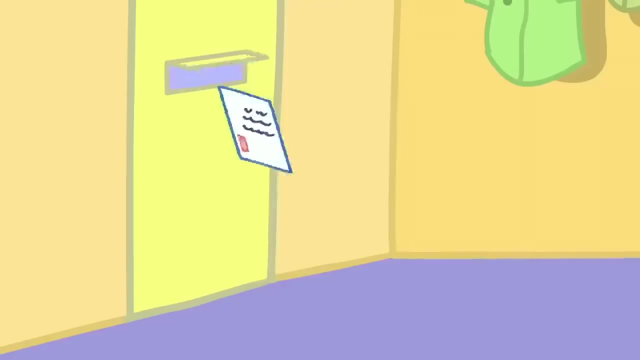 Ho-ho, Of course we can. Peppa, Hooray, HE CHUCKLES Edmund Elephant's birthday. Mr Zebra the Postman's birthday is coming up. Hooray, Peppa the Postman is delivering a letter to Peppa's house. 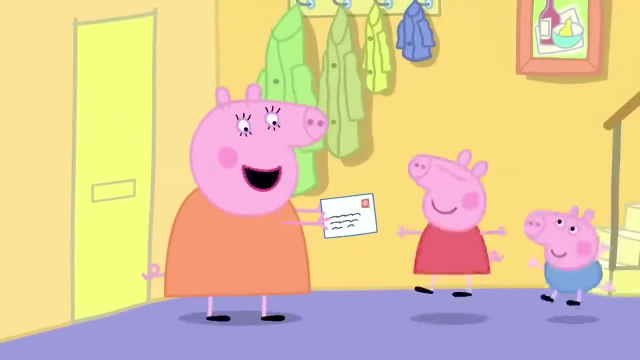 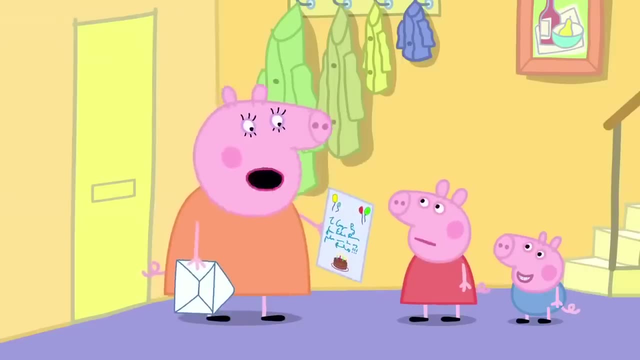 HE CHUCKLES: Oh look, someone's got a party invitation. It must be for me. It says To George Pig from Edmund Elephant, please come to my party, Doesn't it say, George AND Peppa? No, just George. 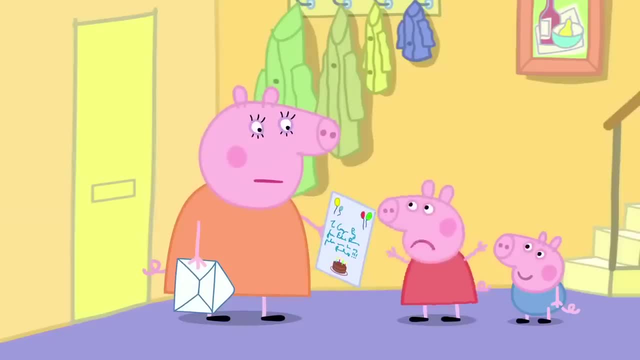 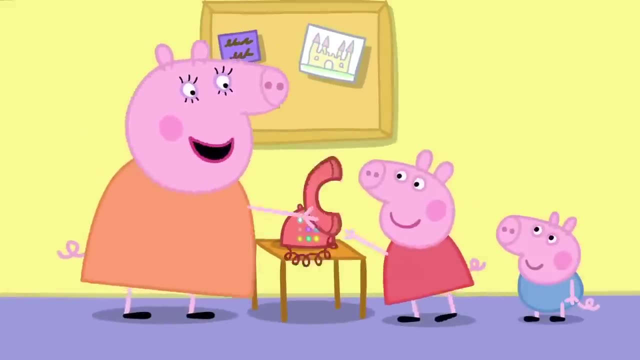 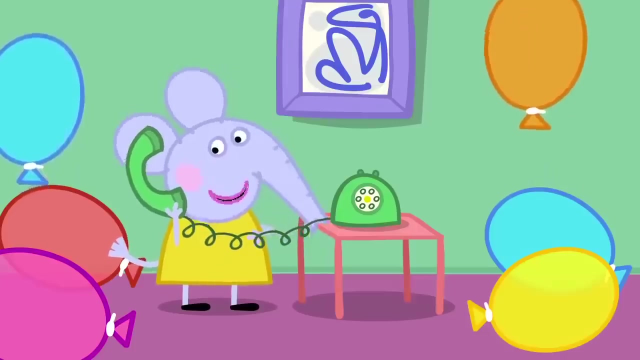 Hm, I didn't want to go to a silly baby party anyway. PHONE RINGS. Hello, Oh, it's for you, Peppa, It's Emily Elephant. Hello. Hello, Peppa, Do you want to come to Edmund's party as my friend? 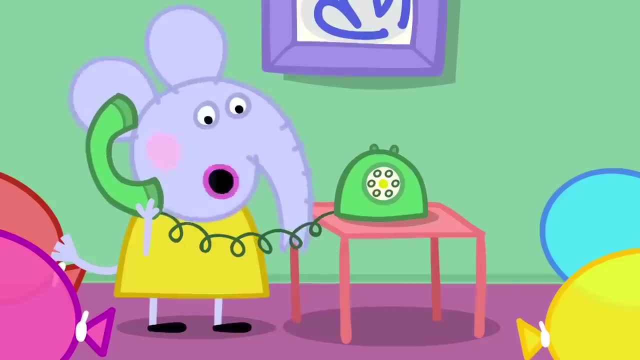 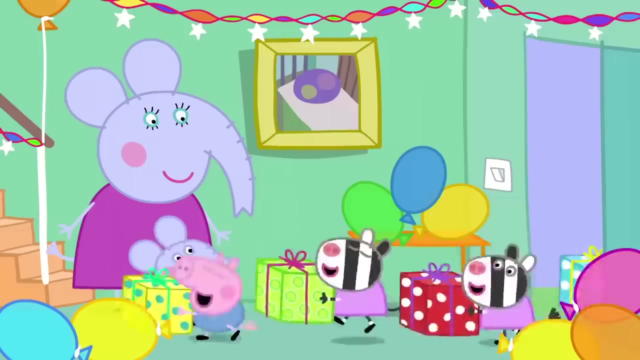 Oh yes, please. My mummy wants to help with the little ones. Help, Yes, I can help. Danny and Suzy are helpers too. Oh goody, HE CHUCKLES, HE CHUCKLES. Everyone is here for Edmund Elephant's party. 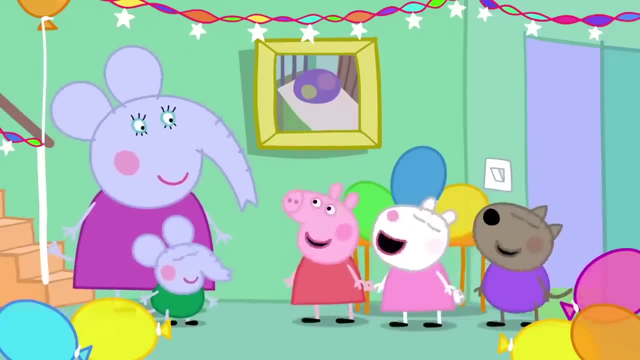 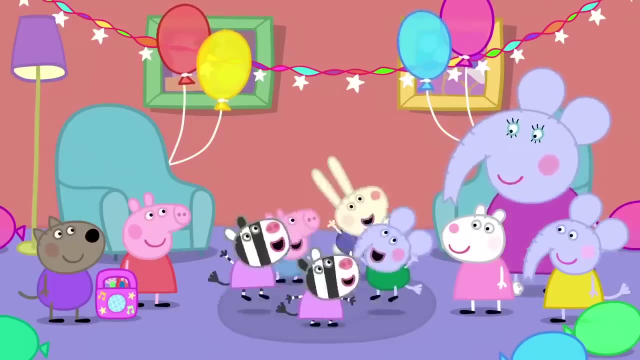 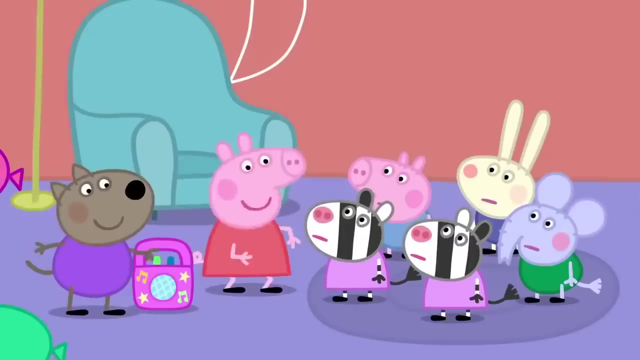 HE CHUCKLES: Ooh, the helpers are here. Hello, Mrs Elephant, Let's get this party started. Who wants to play musical statues? Yay, This is what you do: Dance when the music is playing and when it stops, freeze like a statue. 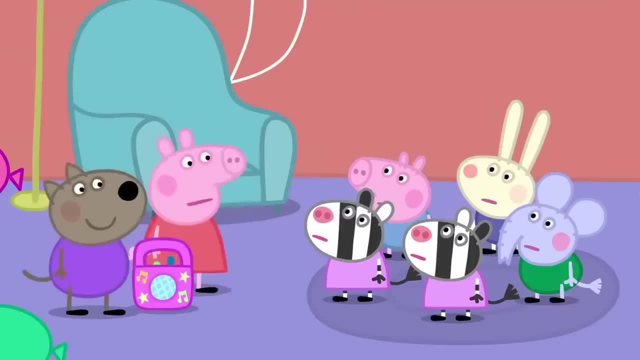 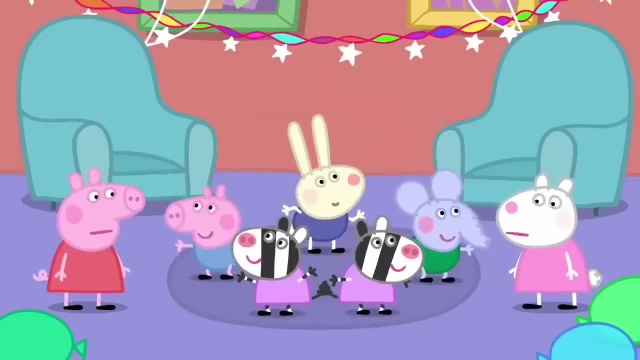 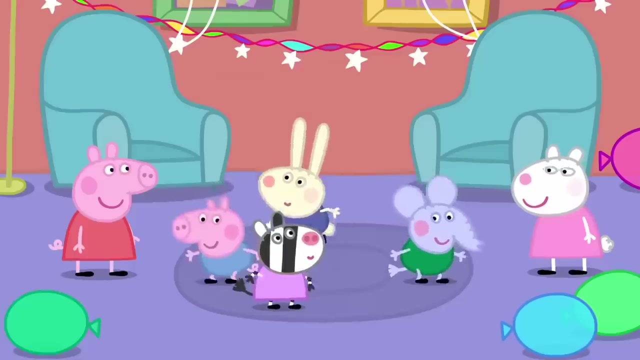 Ready, steady, go. HE CHUCKLES, Just dance already. HE CHUCKLES, HE CHUCKLES, HE CHUCKLES. This one is still blinking, You're out. HE CHUCKLES: RISE AND EARTH AND BACK, You're moving, George. 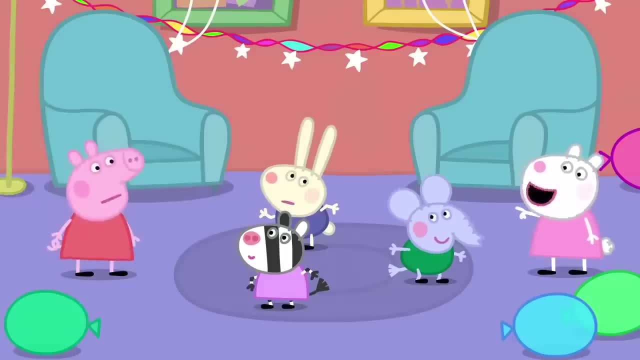 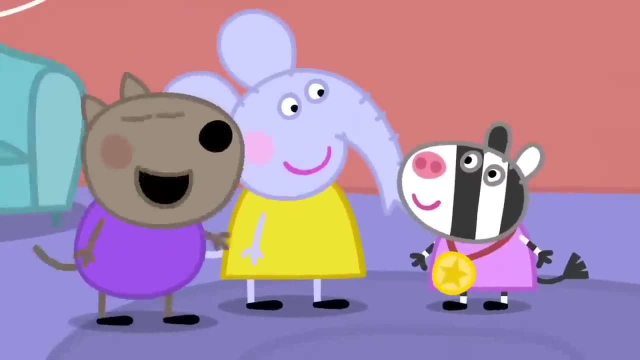 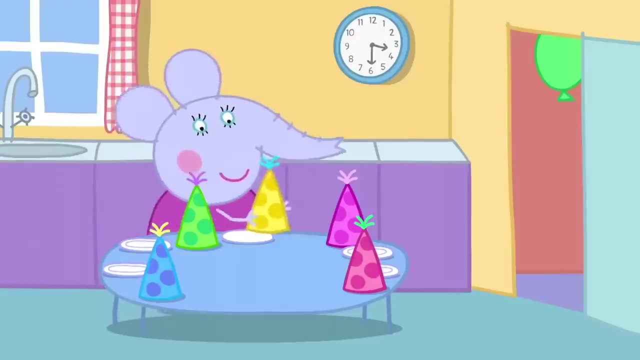 You're out, HE CHUCKLES. Richard and Edmund are out- HE CHUCKLES. So Zaza is the winner. Hooray, You've got a medal. It's made of real plastic gold. HE CHUCKLES, HE CHUCKLES. 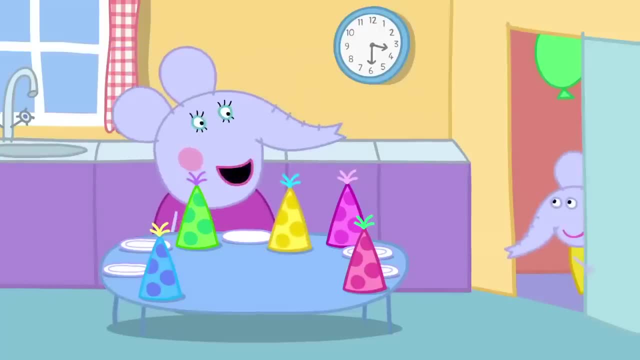 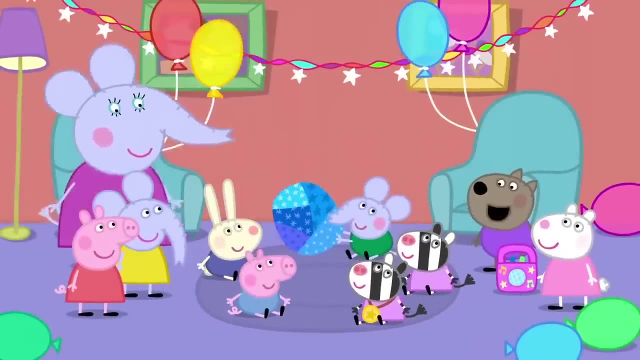 Mummy musical statues is over Lovely, HE CHUCKLES. Now it's time for Pass the Parcel. Yay. When the music plays, pass the parcel round. When the music stops, take some paper off. Ready, steady go. 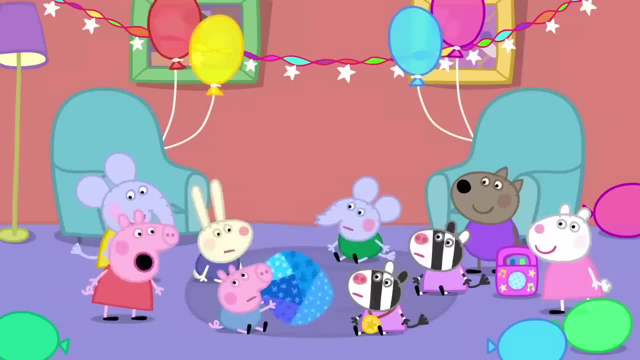 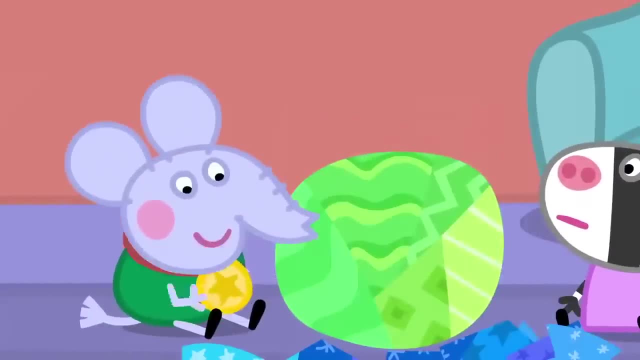 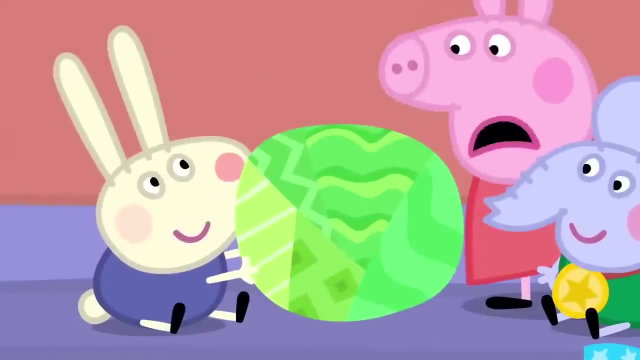 HE CHUCKLES: George, pass the parcel. HE CHUCKLES. HE CHUCKLES: Edmund has got a medal. HE CHUCKLES. HE CHUCKLES: Hurry up Richard, Just take the paper off. HE CHUCKLES: Richard has got a medal. 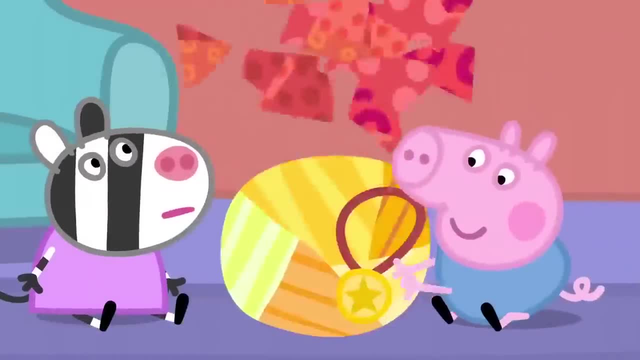 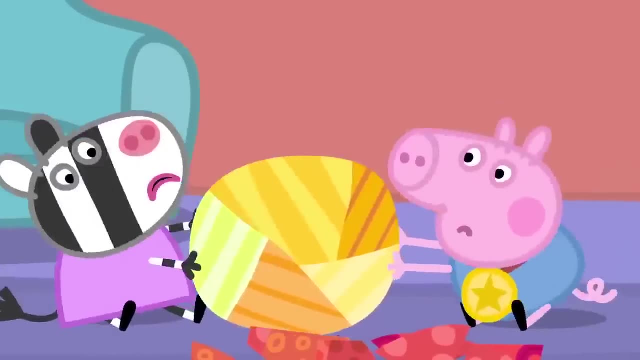 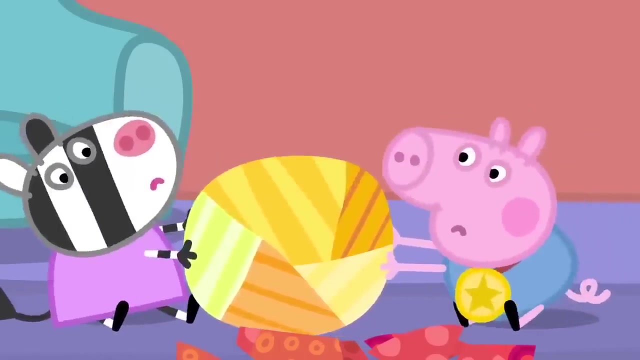 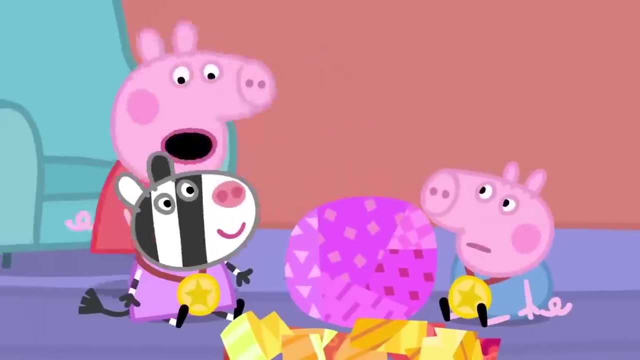 HE CHUCKLES, HE CHUCKLES, George has got a medal. HE CHUCKLES, HE CHUCKLES, Pass the parcel. HE CHUCKLES: Oh dear George isn't passing the parcel. THEY LAUGH: No George, that's Zaza's medal. 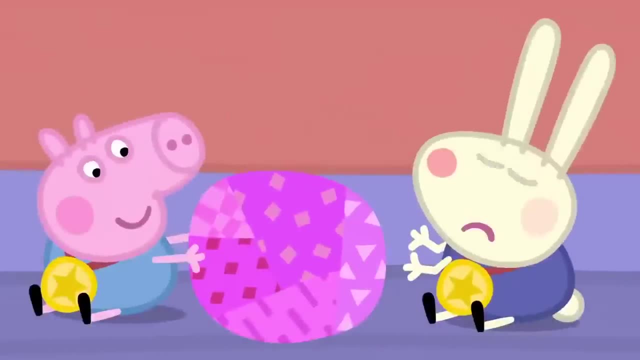 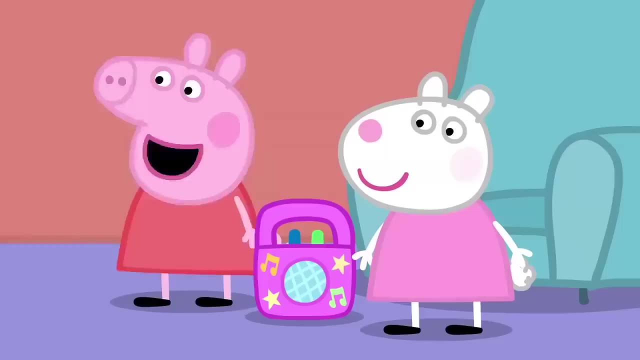 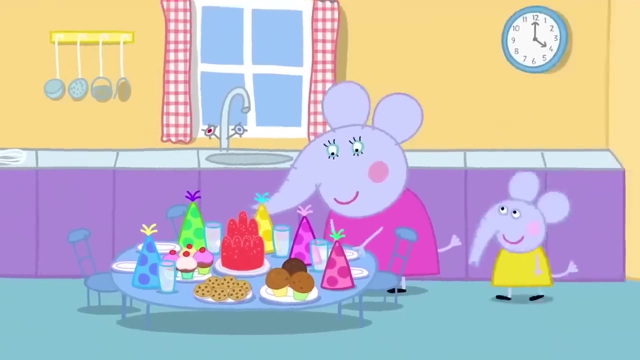 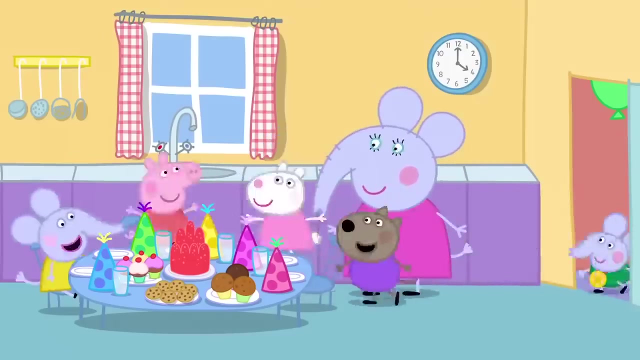 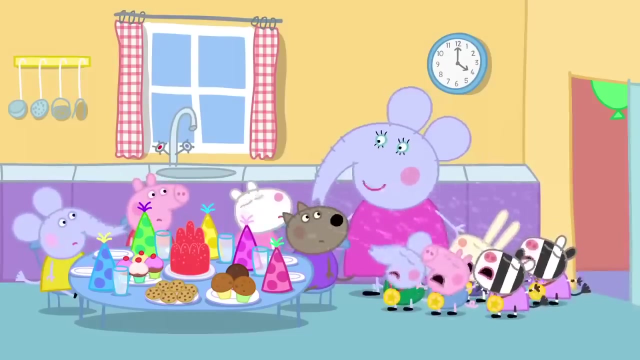 It's a giant teddy. Edmund has won Mummy pass. the parcel is finished. Erm, lovely, Now it's time for food. Hooray, Oh, the helpers have taken all the seats. This is Edmund's party, remember. The helpers can eat after the little ones. 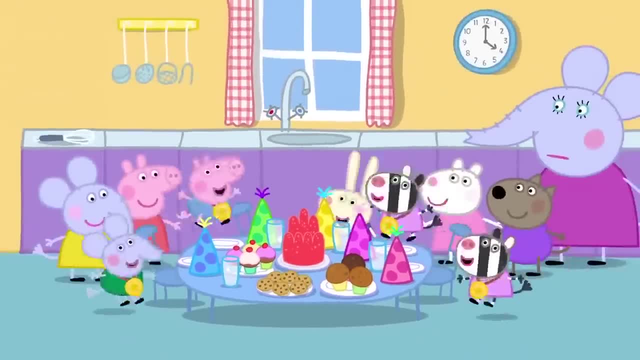 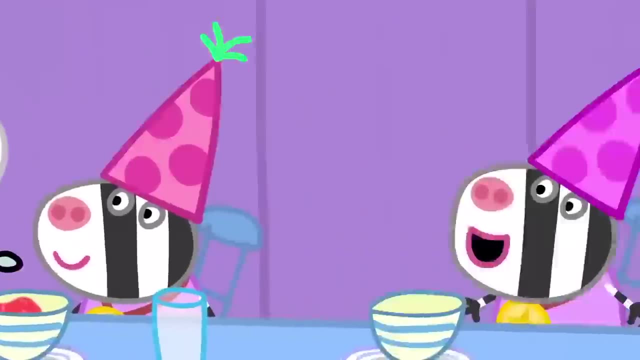 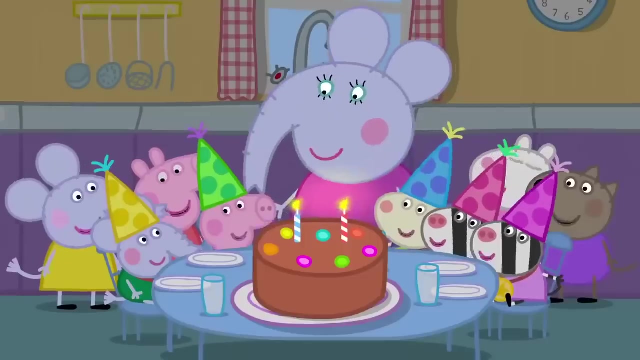 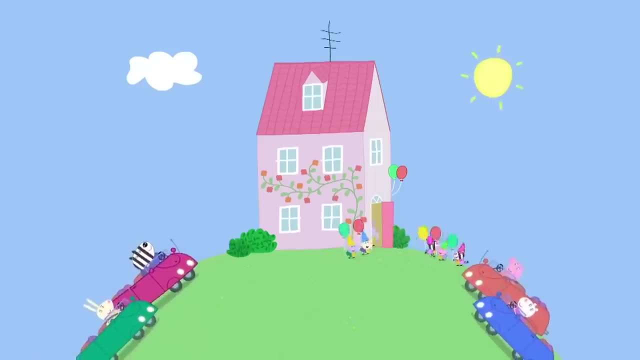 Oh, yes, We're the helpers. Juice please, Juice please, Juice please, Jelly please, Jelly, jelly, More please. Happy birthday, Happy birthday. Happy birthday Edmund. Happy birthday Edmund. It is the end of the party. Thank you to the helpers. You all worked really hard. 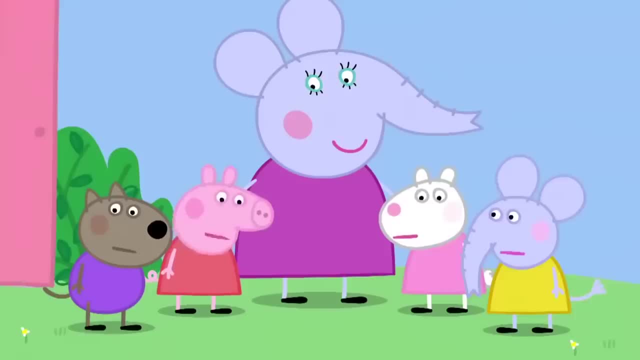 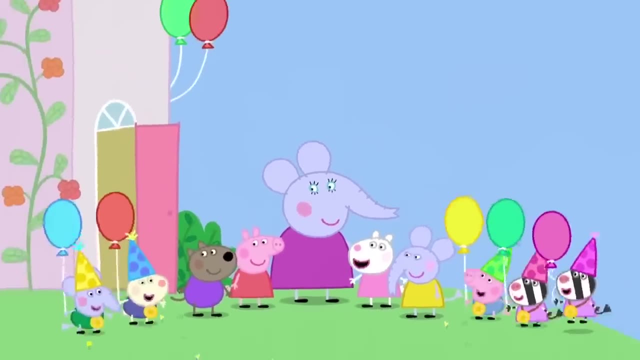 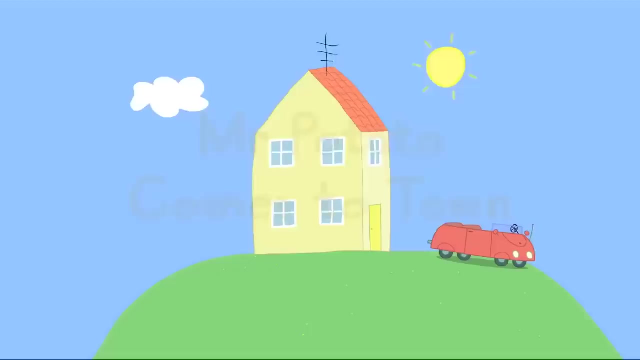 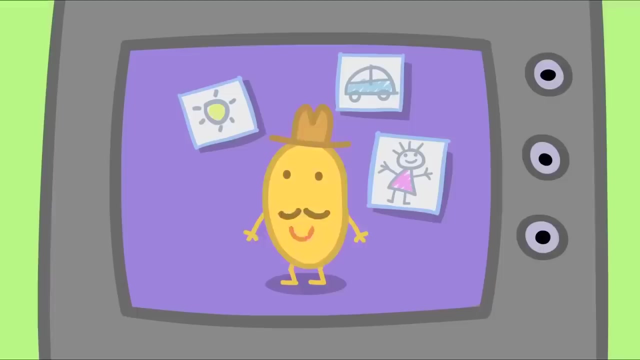 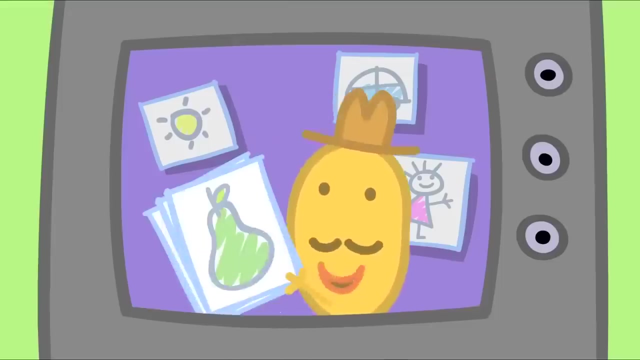 Yes, It's not easy looking after little children. I need to lie down, I need a holiday. Mr Potato comes to town. Peppa and her family are watching Mr Potato on television. I love watching programmes about keeping fit. Now here are some lovely drawings I've been sent. 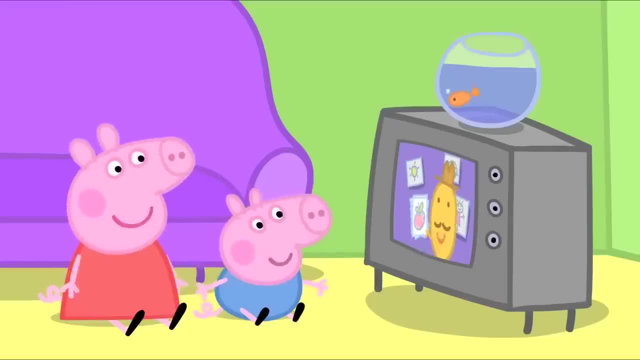 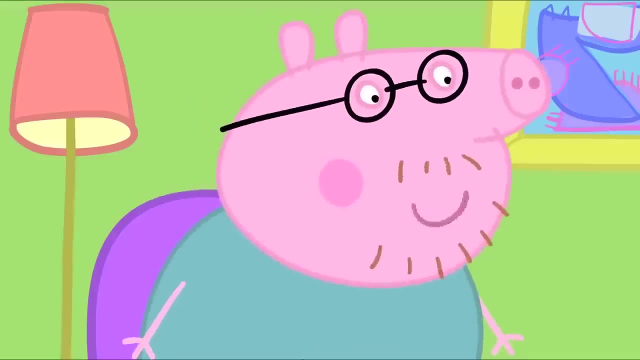 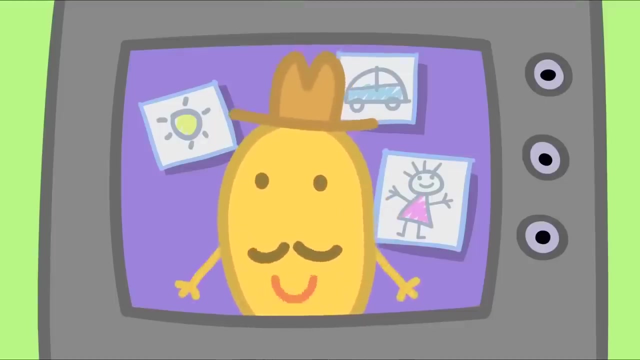 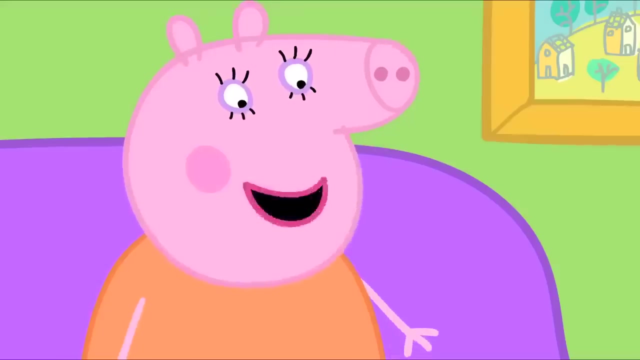 This is an apple. Remember: eating fruit and vegetables helps you stay fit. I'm good at eating fruit and vegetables, And exercise is important. Today you can see me open a new sports centre in town. Mummy, can we go and see Mr Potato? It's a long way to go to see a Potato Peppa. 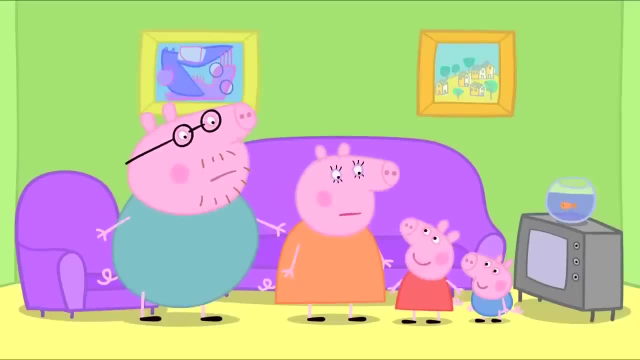 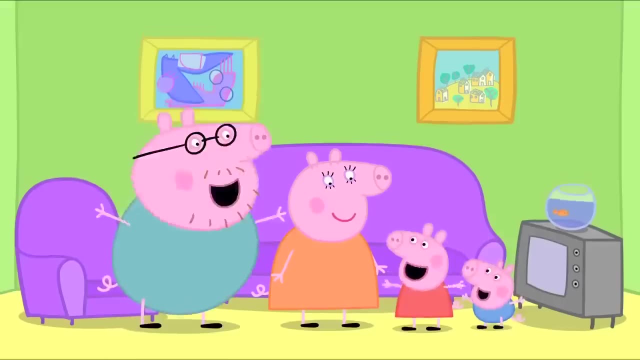 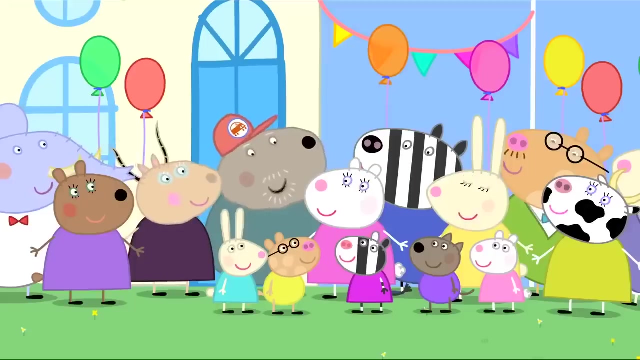 He's not any old Potato. This is Mr Potato. Can we go and see him, Mummy, Please? Oh, all right, Hooray, Everyone has come to see Mr Potato. Everyone has come to see Mr Potato open the new sports centre. Look, it's Mr Potato. 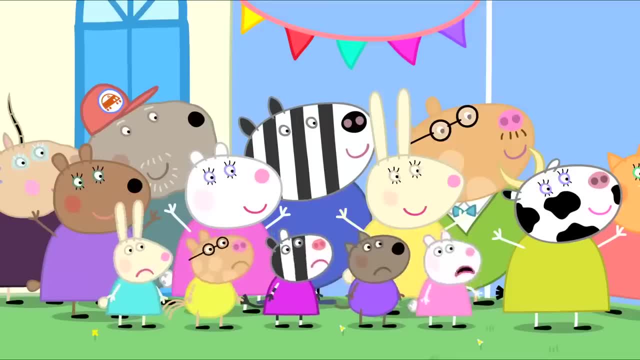 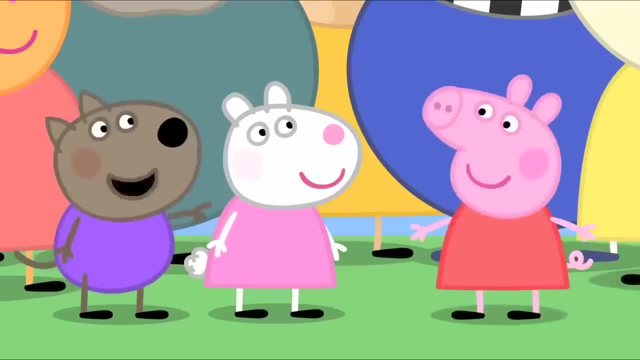 Mr Potato, Oh, it's just Peppa. Hello everyone. Hello Peppa. Susie, thought you were Mr Potato. I don't look like Mr Potato. No, you're much too big. Mr Potato is bigger than me. No, he's not, He's a Potato. 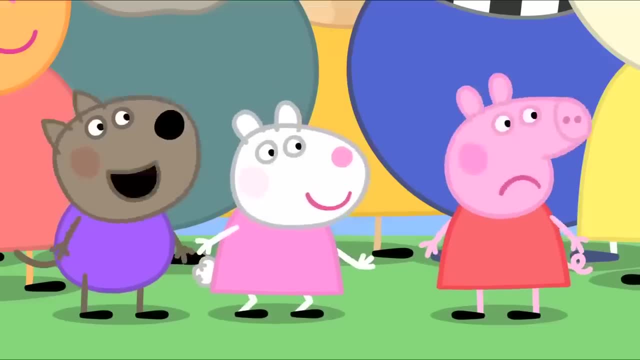 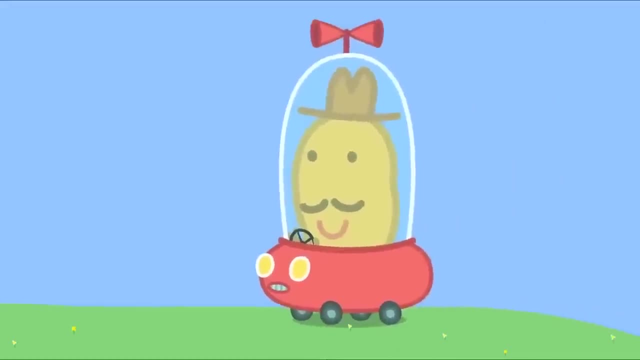 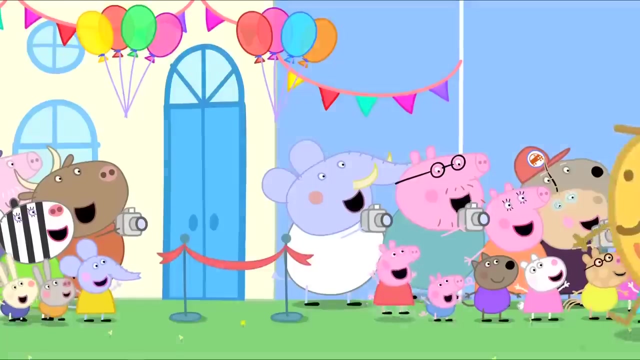 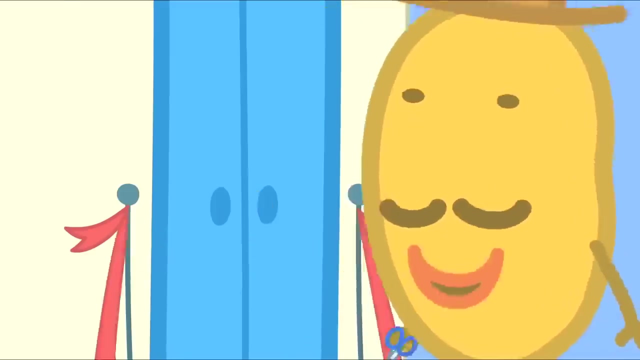 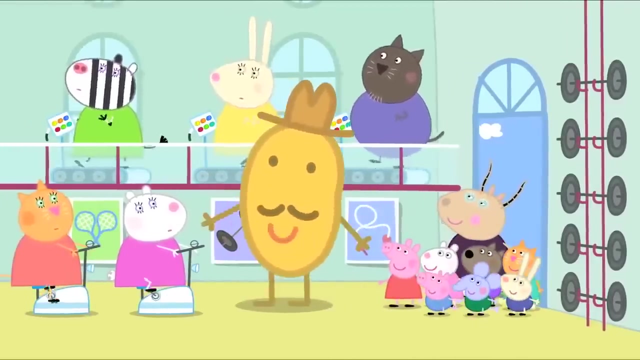 And Potatoes aren't this big. There's, Mr Potato. Mr Potato has come to town. Please welcome your friend and mine, Mr Potato Hooray- Wow, that's a big Potato. I declare this sports centre open. Fantastic. We must all exercise and eat fruit and vegetables. 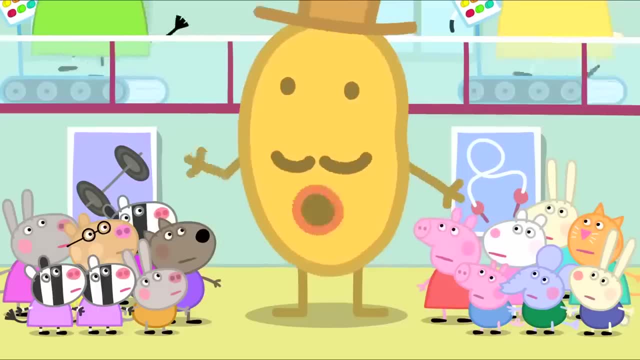 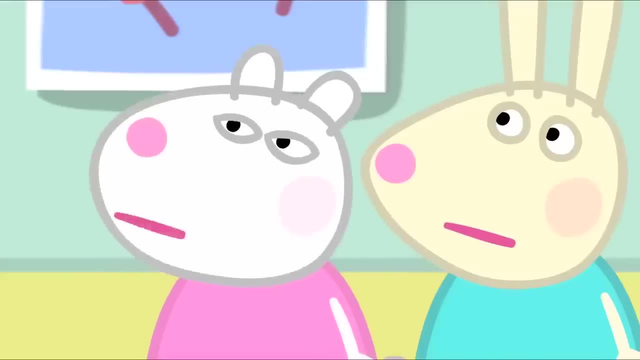 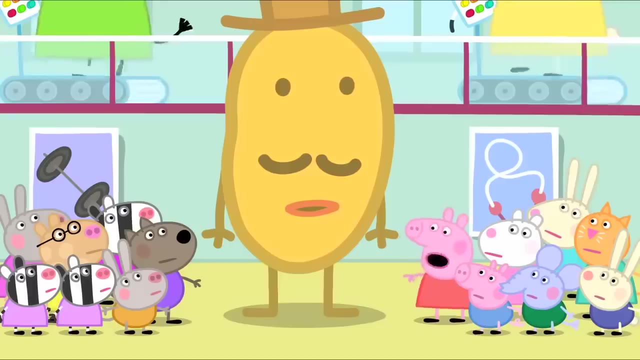 Which one should we eat, Mr Potato, Apples, oranges, carrots, tomatoes, Potatoes, Erm. Why aren't you small like a normal Potato, Erm? Because he's not a normal Potato: He's got legs. Potatoes don't have legs. 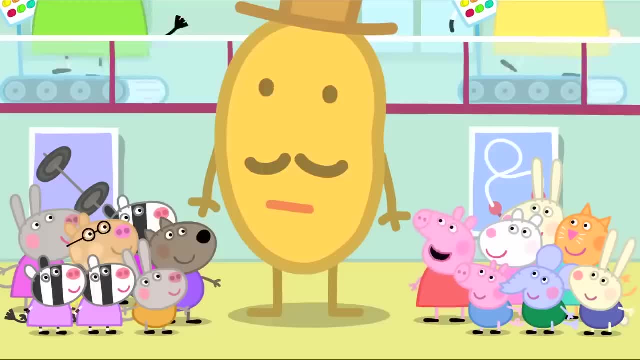 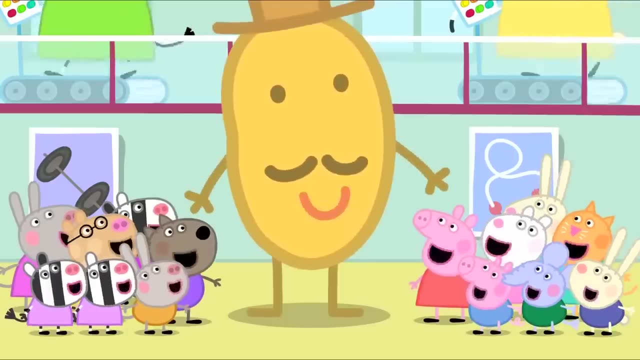 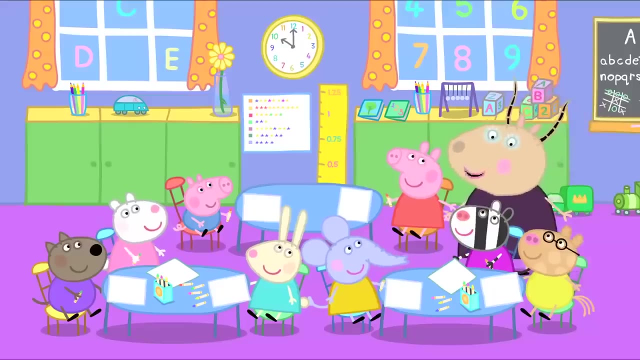 He's a super Potato. We watch your show every morning. Very good, And remember to send me your drawings. We will. Peppa and her friends are at playgroup Children. today we will do drawings for Mr Potato. Hooray, I'm drawing a pineapple. 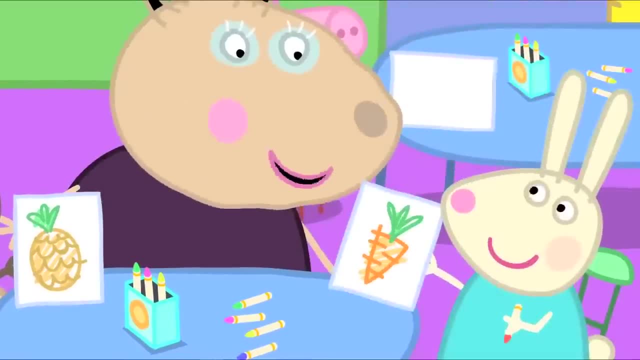 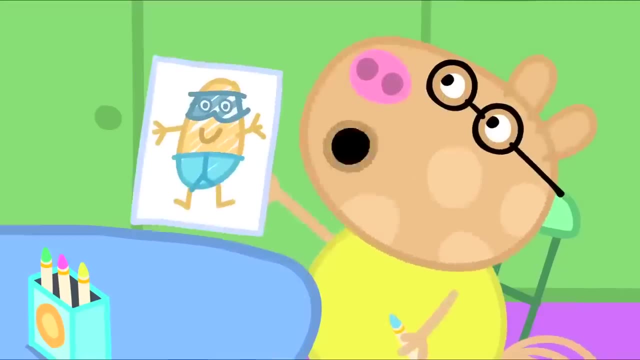 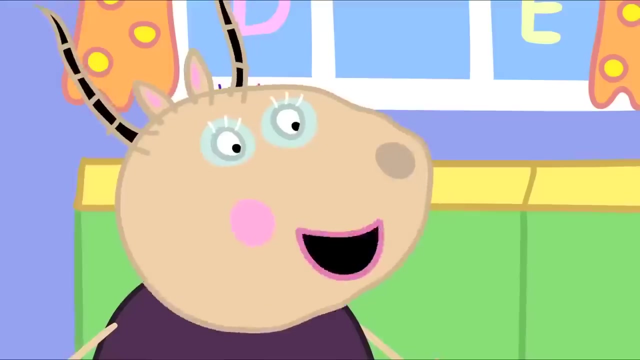 I'm drawing a carrot, Very good, Very good. What are you drawing? Emily, A pea, Lovely. And Pedro, It's a super Potato, Oh, I see. And George has drawn a wonderful tomato. Peppa, what vegetable have you drawn? My Daddy watching television. 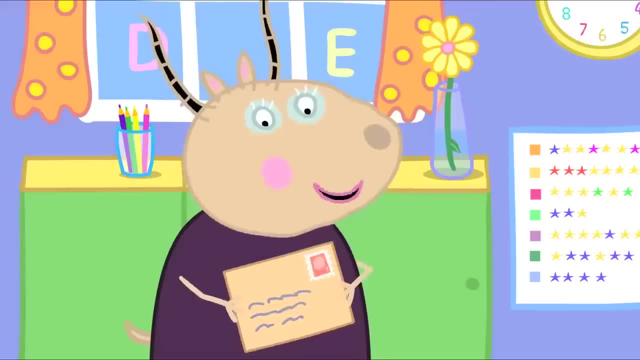 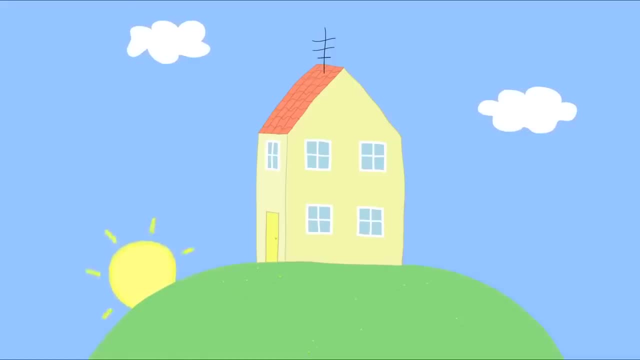 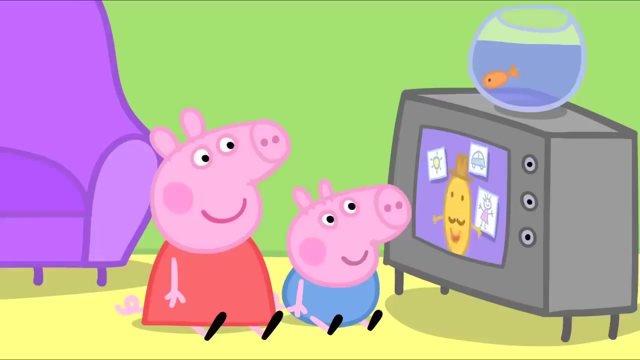 Oh, excellent, Now we put the drawings in an envelope And post them to Mr Potato. It is morning and time for the Mr Potato Show. Please welcome your friend and mine, Mr Potato. We posted some drawings to Mr Potato in an envelope. Did you get the envelope? 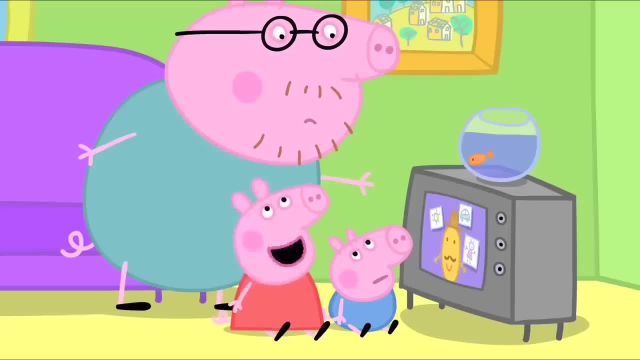 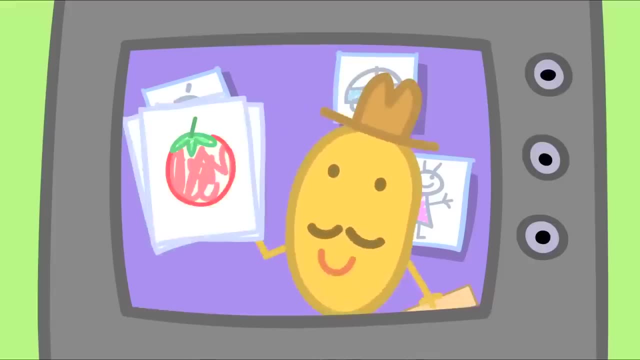 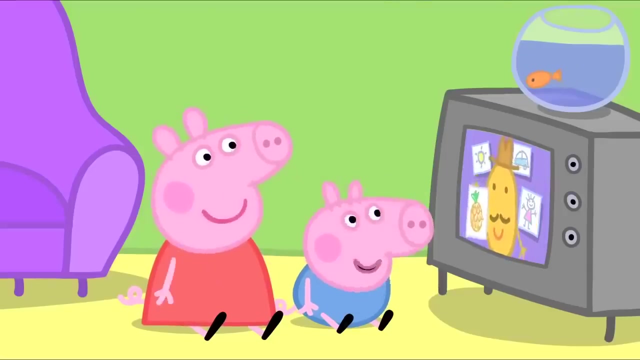 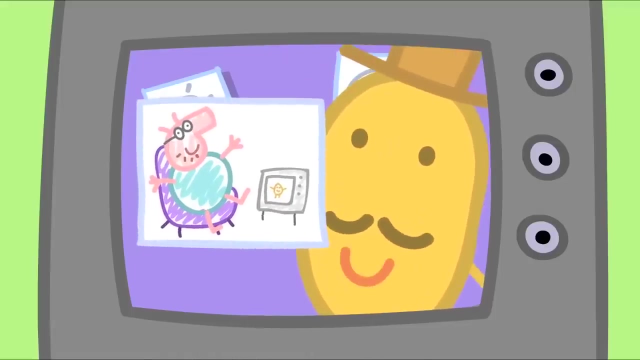 He can't hear you, Daddy. He's on television. Oh yes, of course, I've received an envelope full of drawings. This tomato looks very juicy. That's George's picture. Well done, George, But this picture from Peppa Pig is my favourite. Wow, that's my picture. 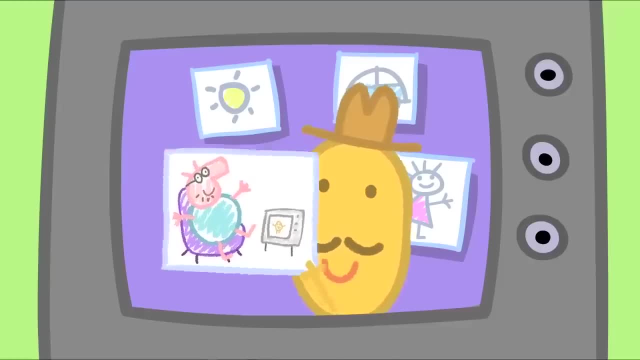 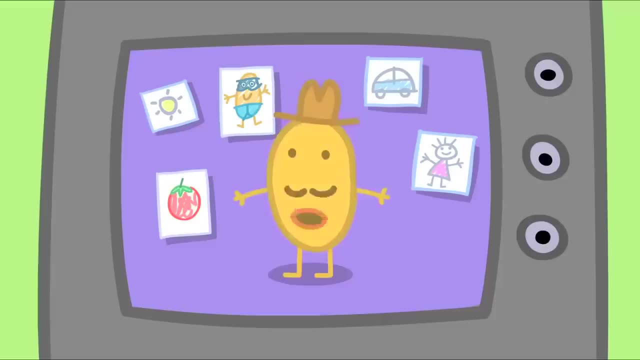 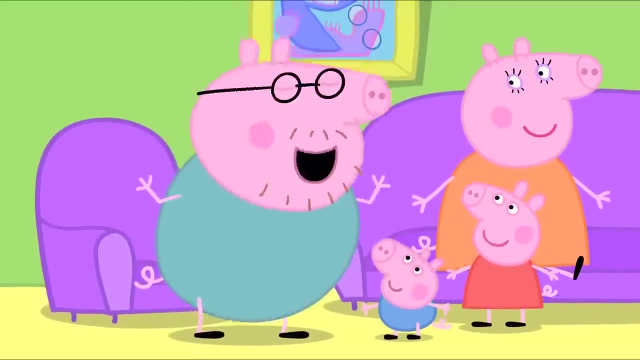 It shows Daddy Pig watching TV. Mmm, looks like Daddy Pig needs some exercise. Eh what? Come on, Daddy Pig, Let's do some jumping up and down. Oh alright, Up and down. Daddy Pig likes jumping up and down, Everyone likes jumping up and down. 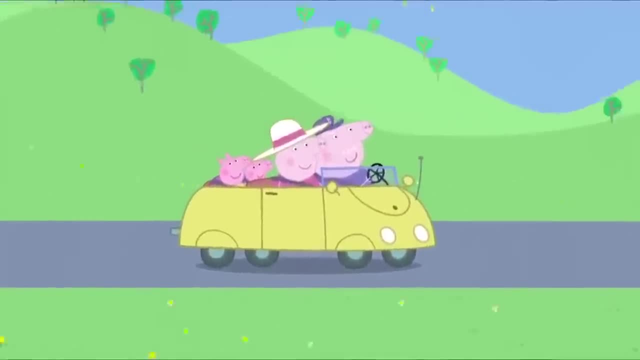 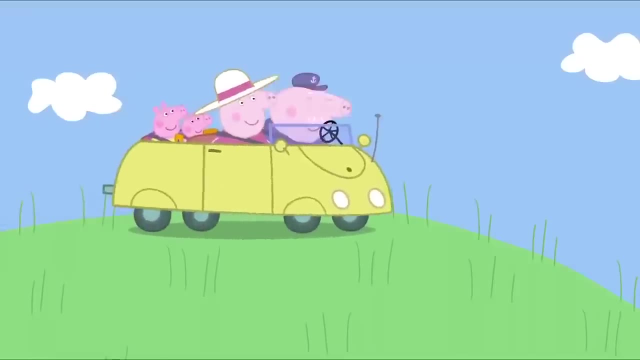 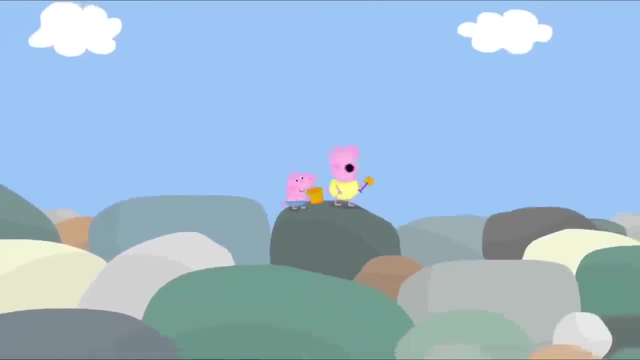 Rock pools. Peppa and George are going to the seaside with Granny and Grandpa Pig. Peppa and George love the seaside. Peppa and George love the seaside. Oh, where's the sand gone? There isn't any sand on this beach, Peppa. 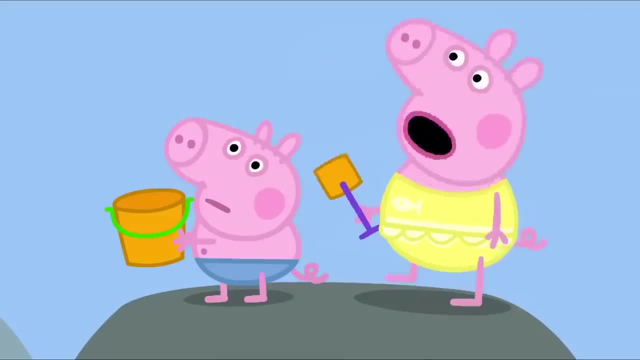 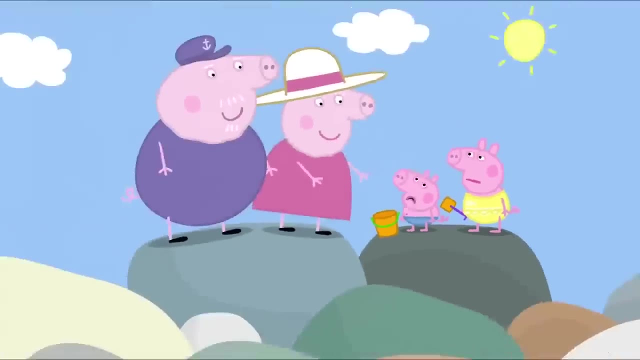 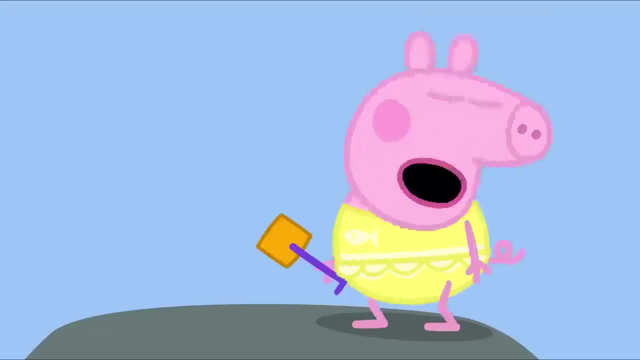 No sand, But we wanted to make sand castles. Peppa and George love making sand castles. Now, now, George, don't be upset. There are lots of exciting things to do on this rocky beach. Like what? When the sea goes out, it leaves little pools of water in amongst the rocks. 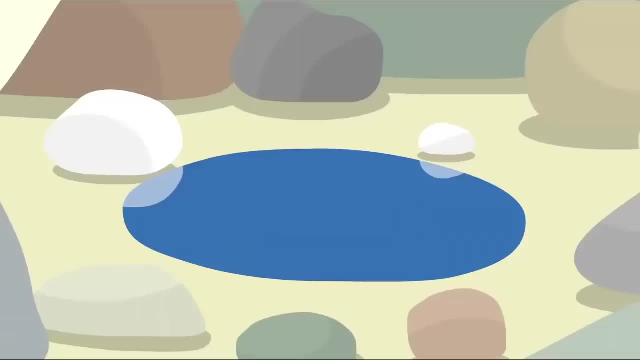 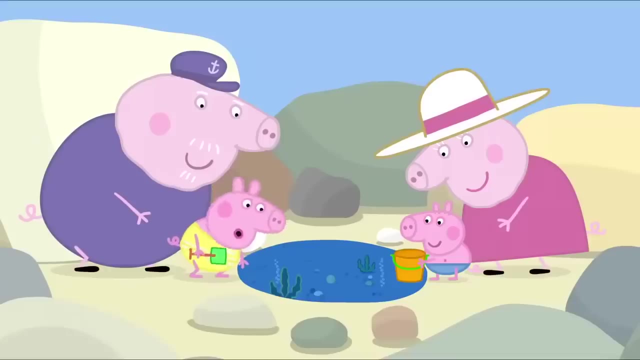 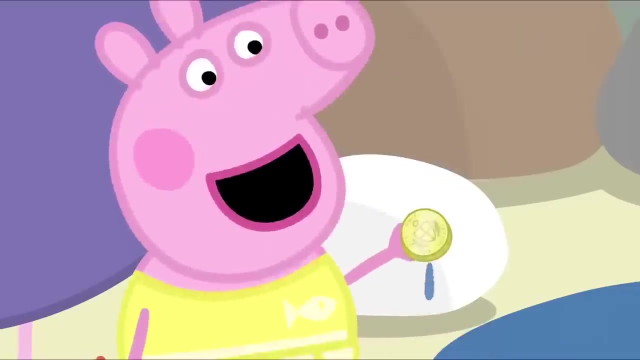 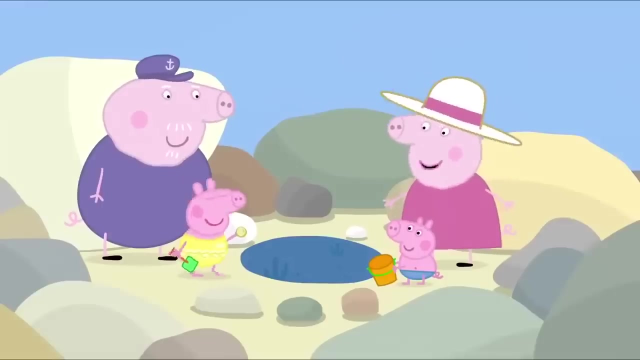 They're called rock pools, And in every rock pool there's something special that the sea has left behind. Ooh, I can see something glittering. It's a coin. Wow, Maybe it's a pirate's treasure. Ooh, Let's make a collection of all the things we find. 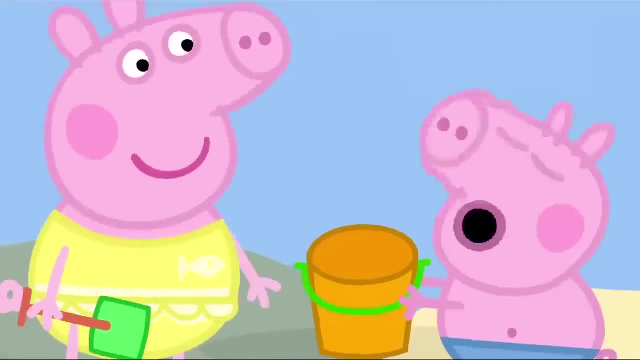 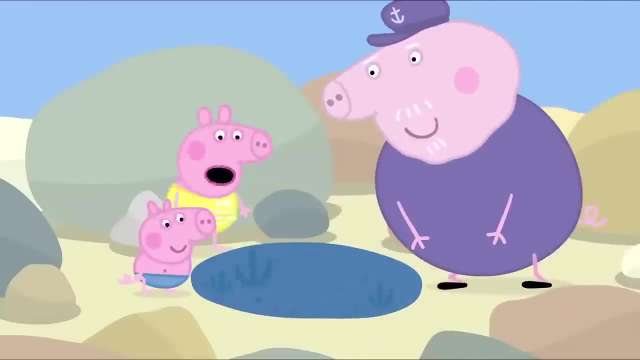 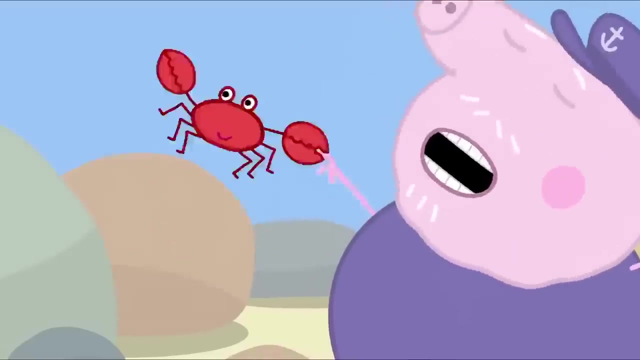 Yes, We'll put them in George's bucket. What surprise is waiting in this pool? There's nothing special in this one. There's always something. Peppa, Look closer. Ooh, there is something. Yes, it's a crab. Ahhhh, The crab is pinching Grandpa Pig's finger. 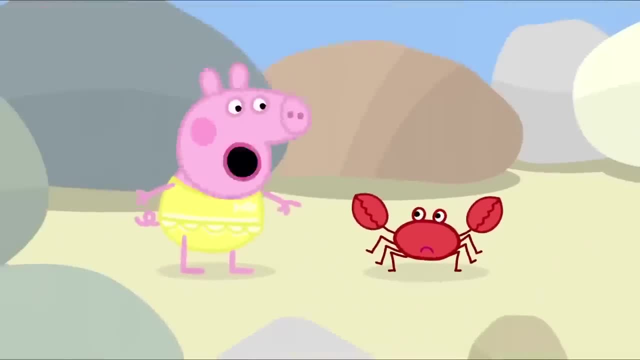 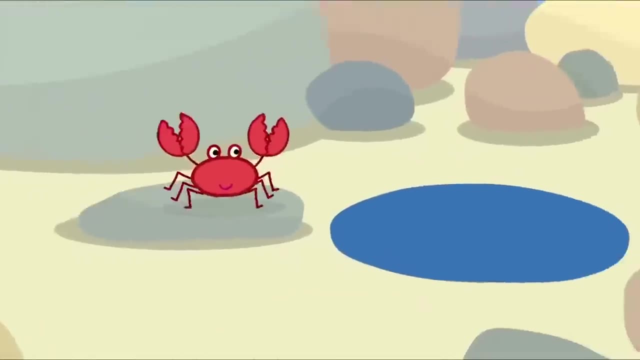 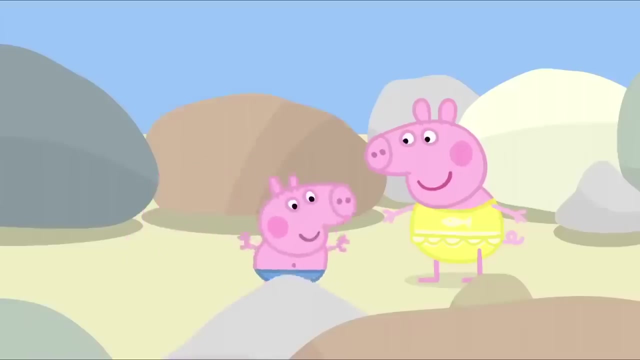 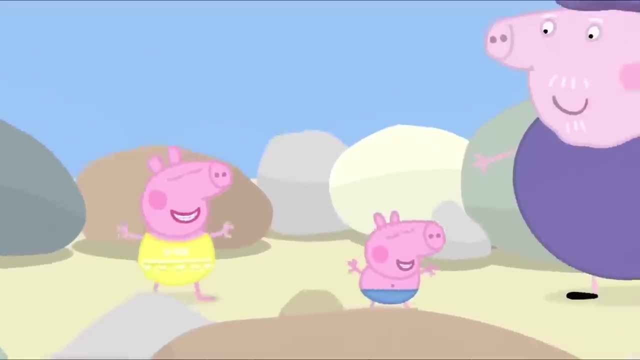 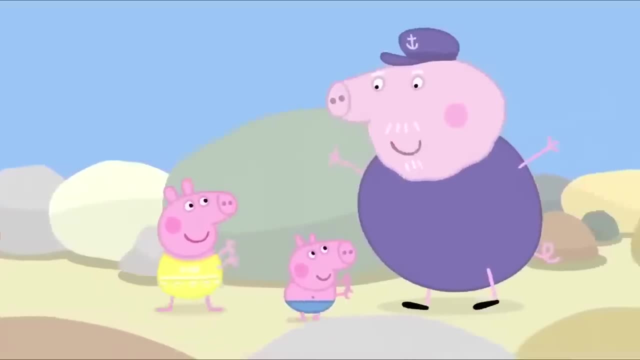 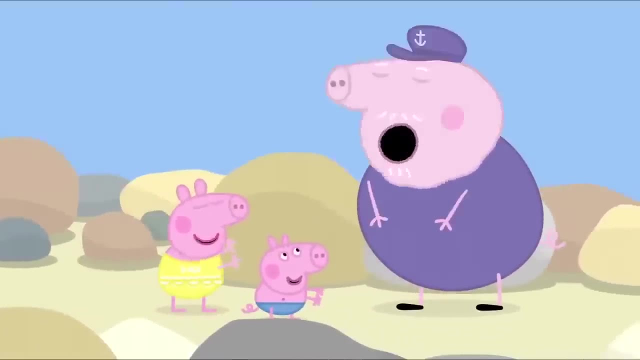 Help. There are two naughty crabs trying to pinch me. Pinch, pinch, pinch. We're naughty crabs. Pinch, pinch, pinch, Shoo, shoo, shoo. you naughty crabs, Go back to your little rock pools. Yes, Let's look in more rock pools. 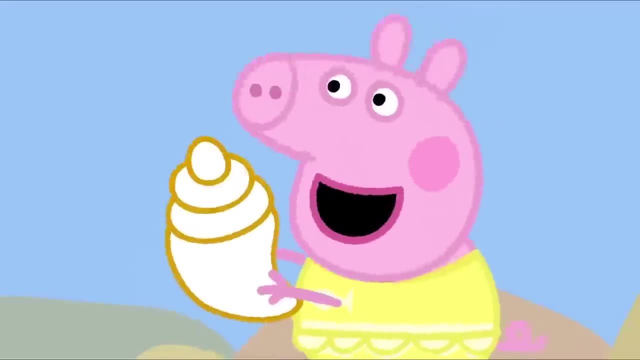 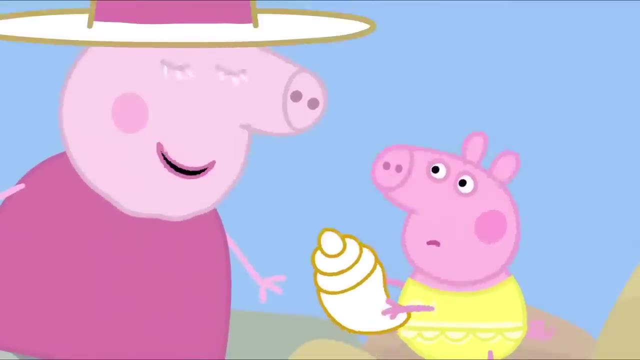 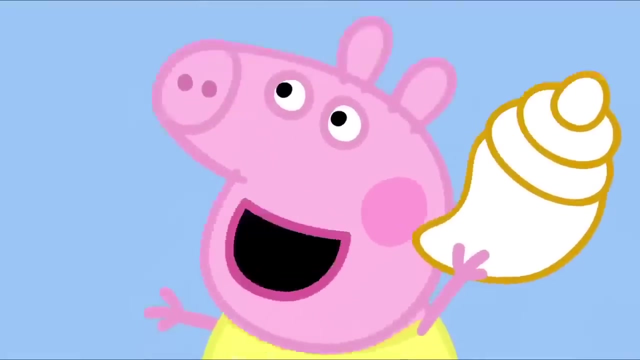 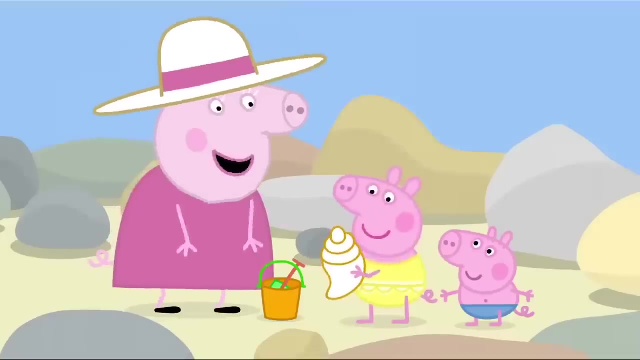 What can you see? A sea shell. Can you hear the sea in it? What do you mean? If you put a shell to your ear, you can hear the sea. Wow, I can hear the sea. I love my sea shell. George, can you find a sea shell too? 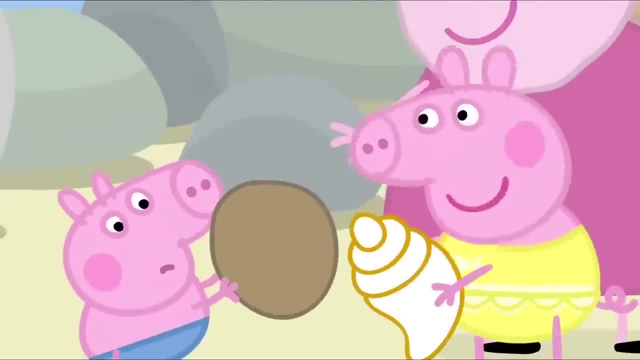 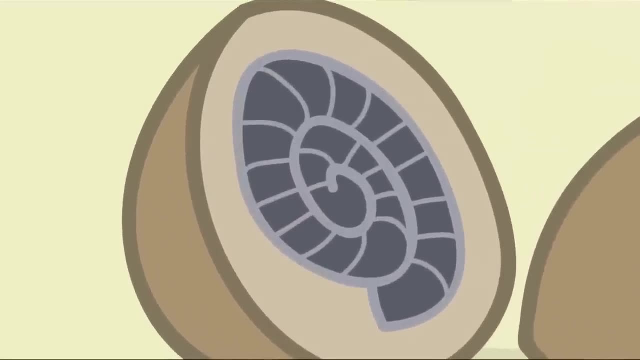 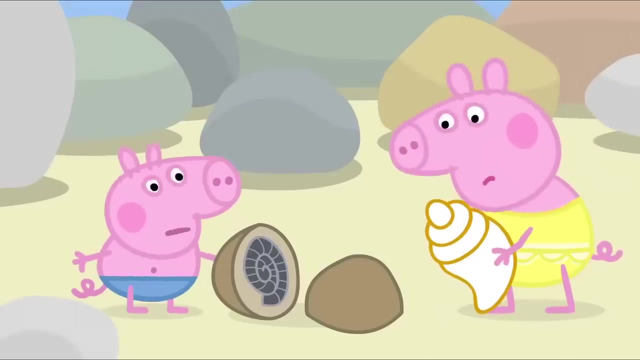 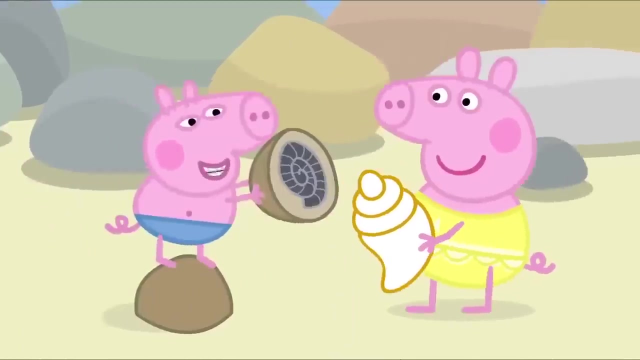 Shell, That's not a shell. Oh, Peppa's right, that's not a shell. George has found a fossil. What's a fossil? A fossil is the remains of an animal that lived long ago, when there were dinosaurs. Dinosaur Rock pools are such fun. 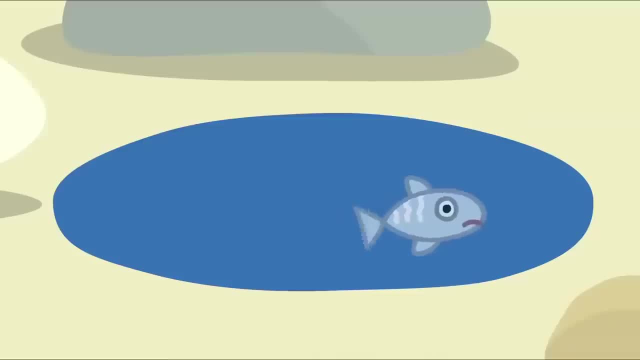 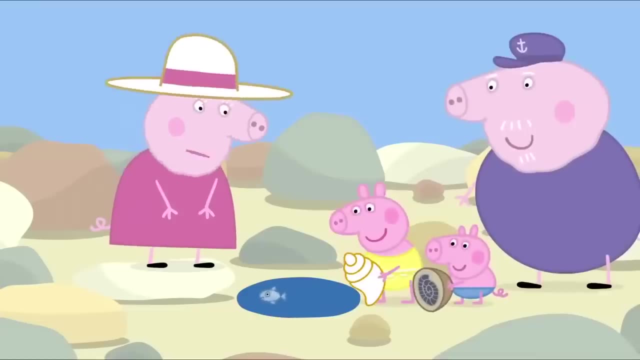 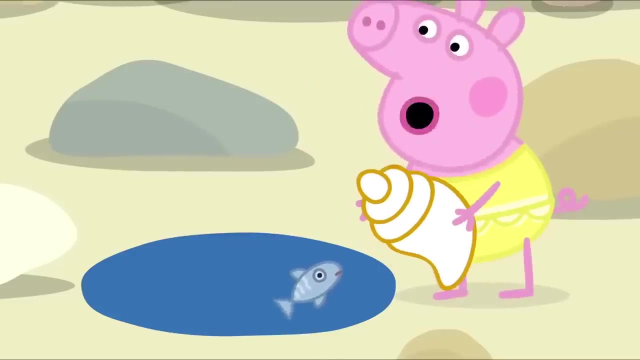 Yes, they're fun for us, But not for this little fish. A fish Where Poor little fish she's trapped. Oh, oh, The little fish says she wants to go back to the sea. Maybe you could use your bucket to rescue her. Yes, 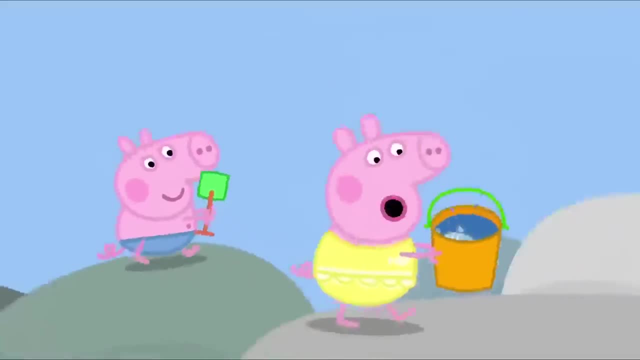 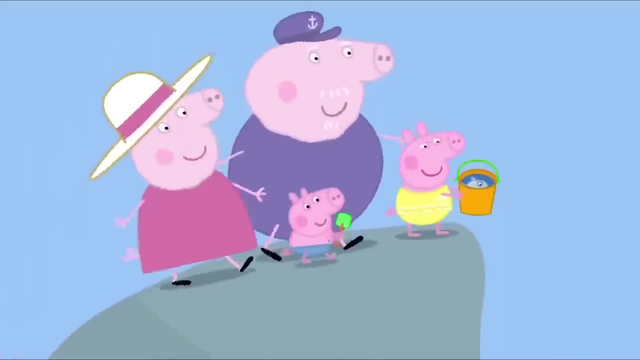 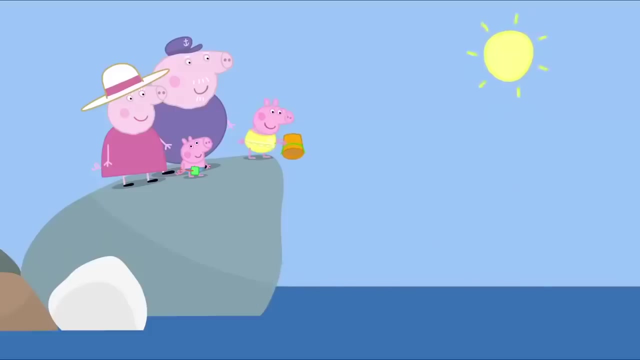 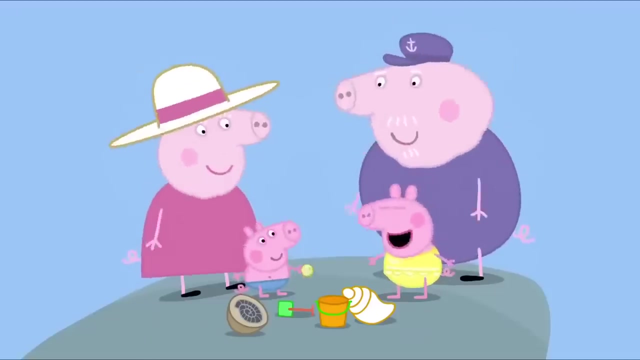 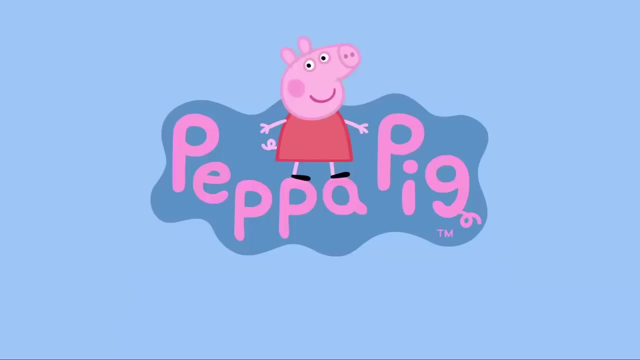 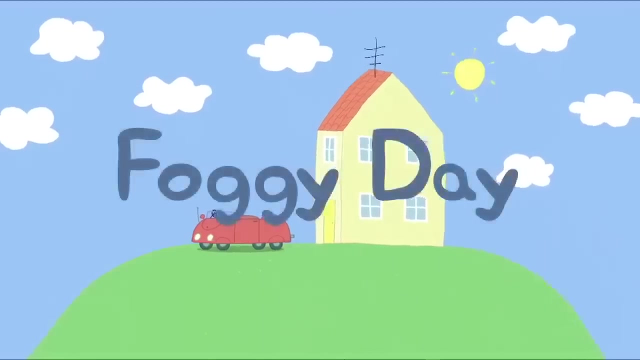 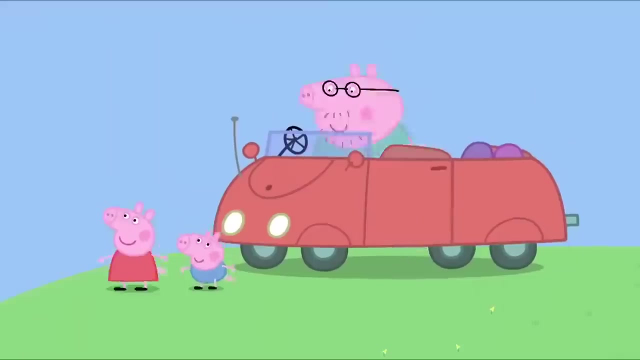 Peppa is rescuing the little fish in her bucket. Don't worry, Mrs Fish, You'll soon be back with your friends. Bye-bye, Mrs Fish, Bye-bye. I love rock pools. Foggy day. Peppa and George are going to the playground today. 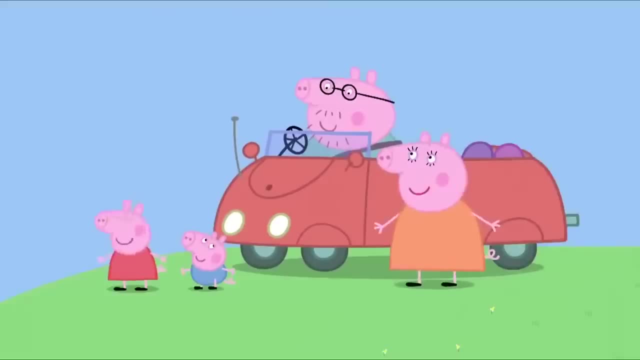 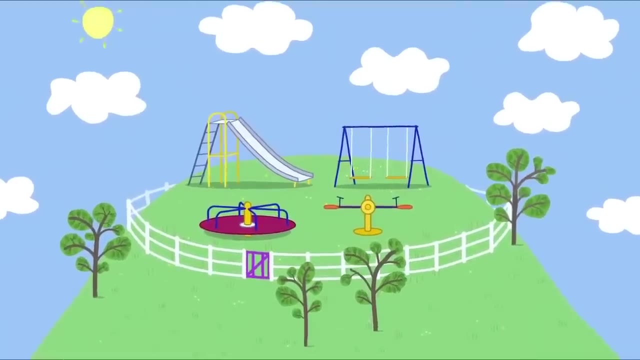 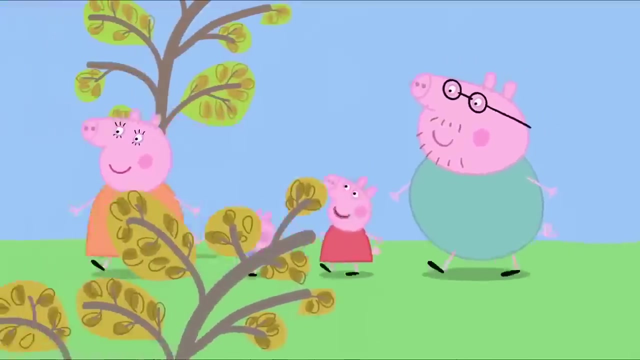 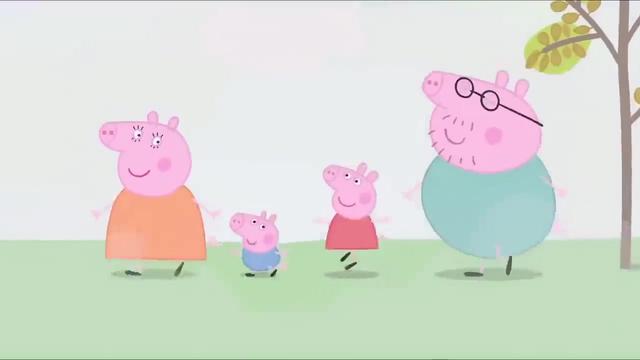 Should we drive to the playground? No, let's walk. Look, it's just over there. The playground is quite close. OK, let's walk This way, everyone, Thanks, We're going to the playground. We're going to the playground. Oh, Where has the sky gone? 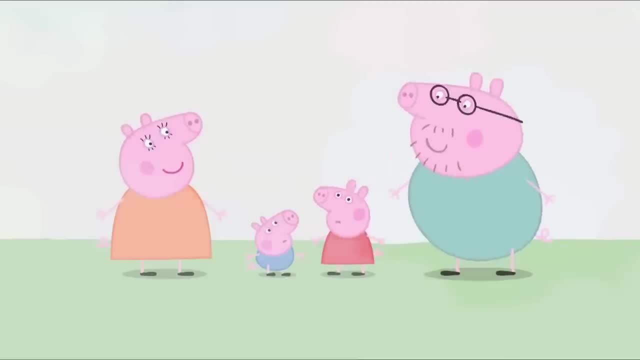 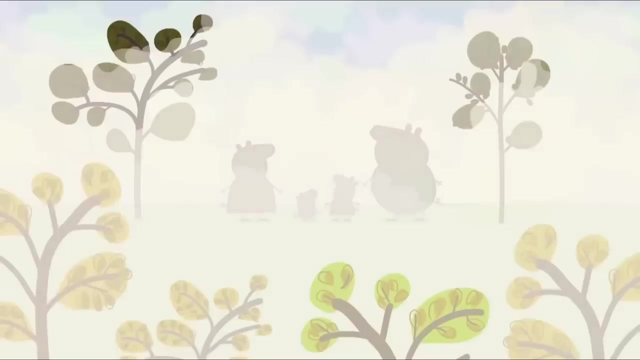 Don't worry, Peppa, It's just fog. What's fog? Fog is a cloud that is on the ground instead of in the sky. Oooh, It's very thick fog. I can't see a thing. Hmmm, Maybe we should go back home. 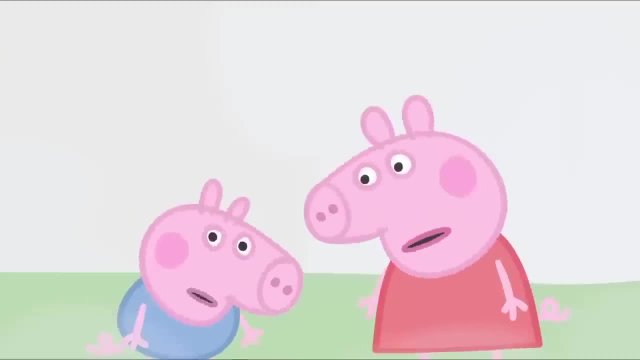 Yes, We'll go to the playground another day. Aww, It is too foggy to find the playground, So Peppa and George have to go back home. Now, which way is home? Are we lost? Daddy Pig, Don't worry, I know exactly where we are. 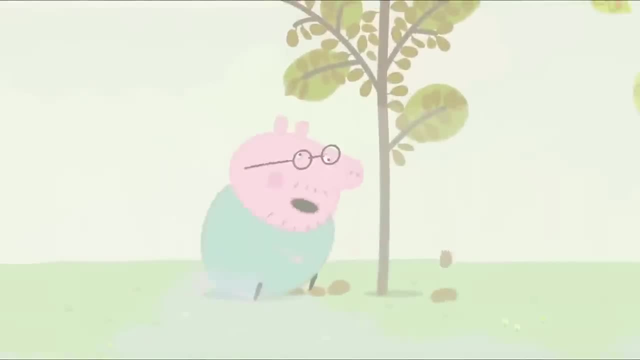 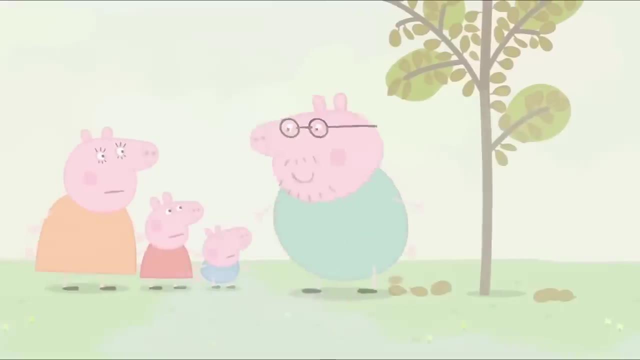 This way? Who put that tree there? Daddy Pig has walked into a tree. Are you OK, Daddy Pig? Yes, I'm fine This way. Daddy Pig, do you know where you're going? Yes, of course I do. I don't think we'll ever find our house again. 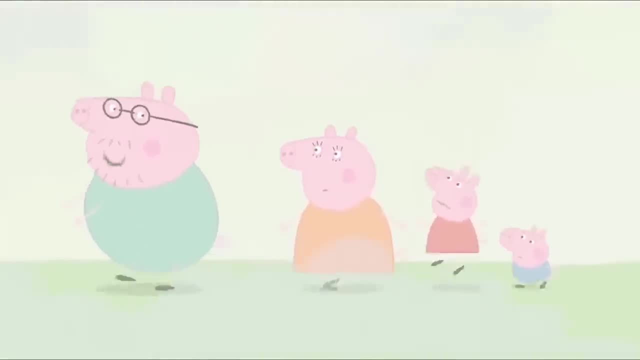 I'm sure we will, Peppa. We're only in our garden. Oh, it's the ducks. Hello, Mrs Duck. Have you lost your pond? We're lost too. We are not lost. I know exactly where we are. See you later, ducks, Good luck finding your pond. 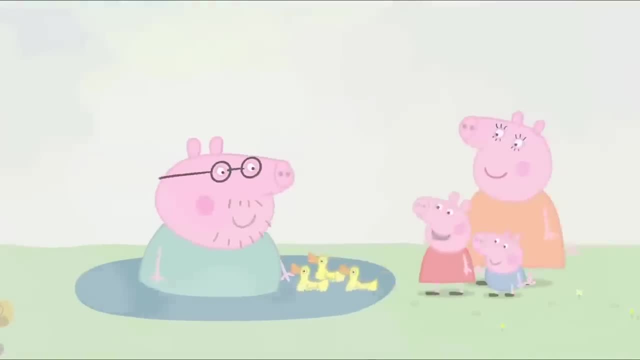 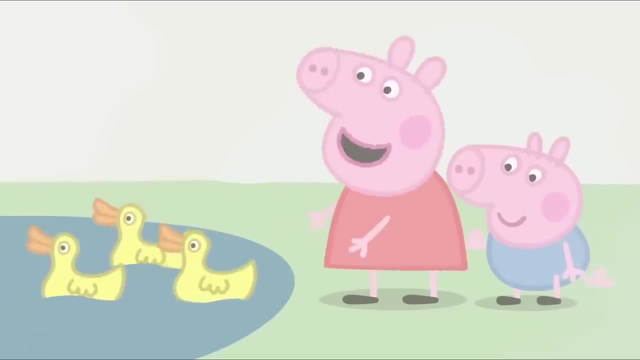 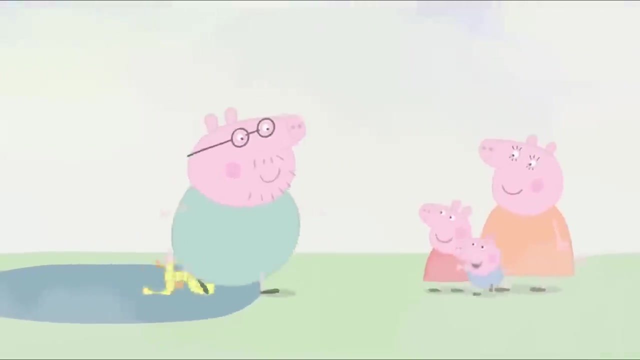 Daddy Pig has found the duck pond. That's lucky. Yes, What a stroke of luck. Daddy The duck says: thank you, You're most welcome, Mrs Duck. Now let's find our house. I'm sure it's this way. Hello, Did you hear something? Yes, I thought I heard someone say: 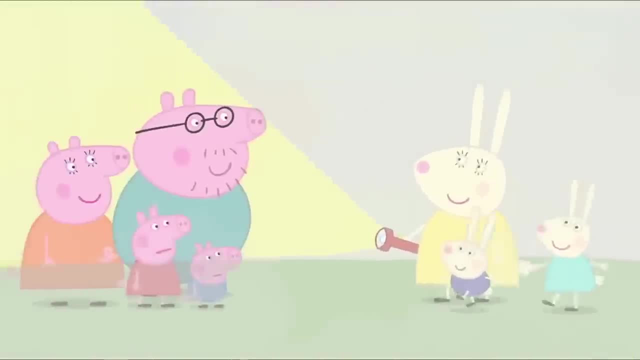 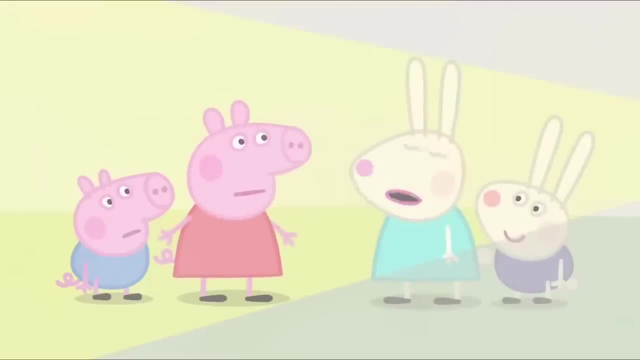 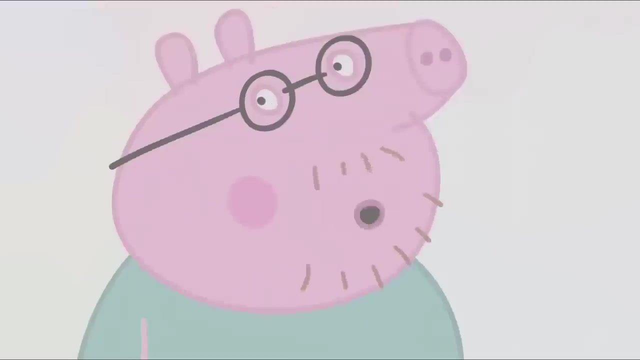 Hello, It's Mummy Rabbit with Rebecca and Richard. Hello, Peppa, We're lost. Hello, Rebecca, We're lost too. We wanted to go to the playground, So did we, But it's too foggy to get there. Come on, everyone, Back to our house until the fog clears. 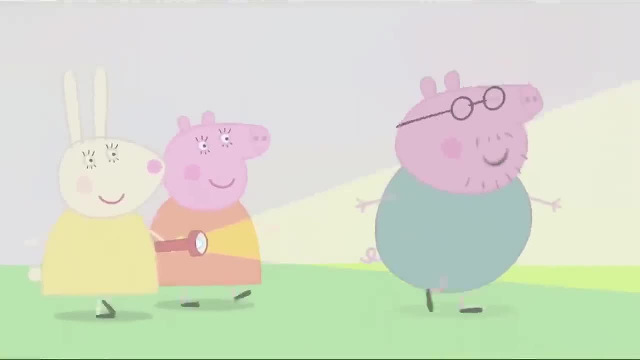 Daddy Pig, do you know where you're going? Yes, of course I do This way. Yes, Daddy Pig. Aha, I've found our little hill. We'll soon be home. Hooray, Our house should be just about here. Oh, Daddy Pig has found a ladder. 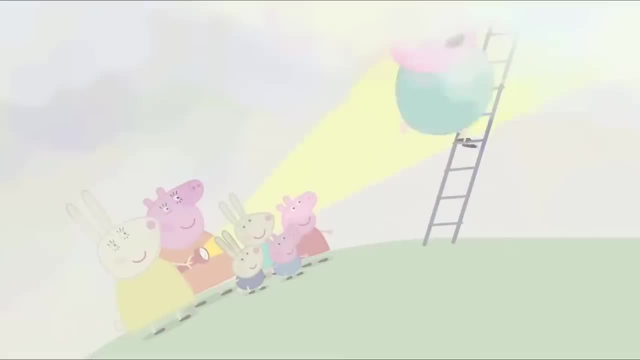 That's strange. We don't have a ladder in our garden. Goodness me, Can you see where we are, Daddy Pig? Yes, I can, Daddy, where are we? Why don't you have a look? Okay, Let's go. Wow, Wow, I can see everything again. 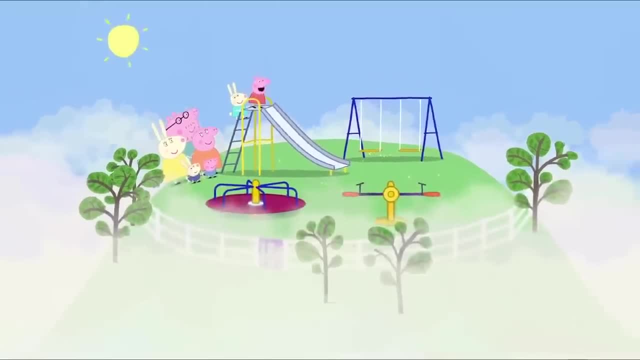 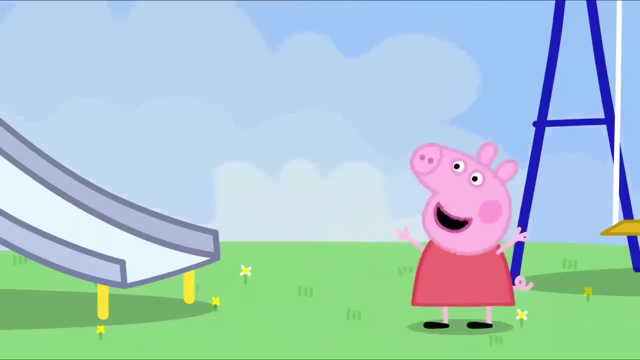 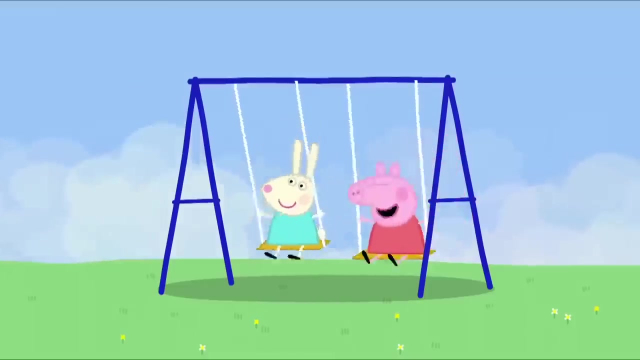 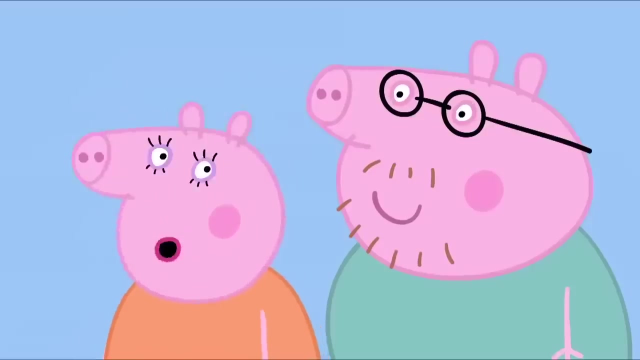 The fog is going away. We're at the playground. Hooray, Whee, We're at the playground. We're at the playground. Whee, See-saw, See-saw. Daddy Mummy, We're at the playground. Well, that's lucky, But I thought we were trying to get home. 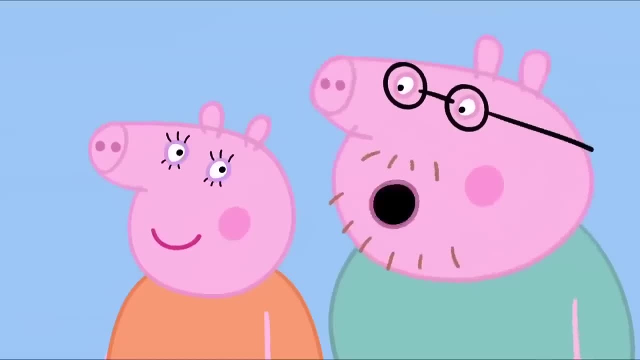 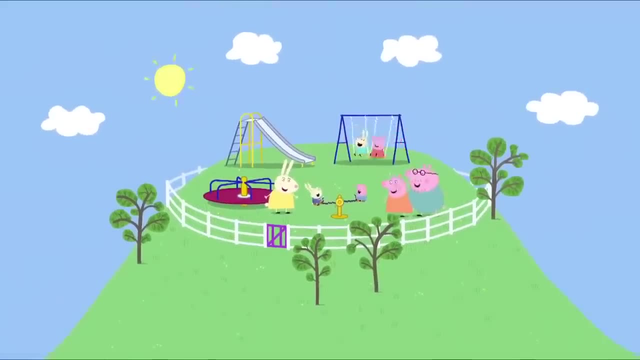 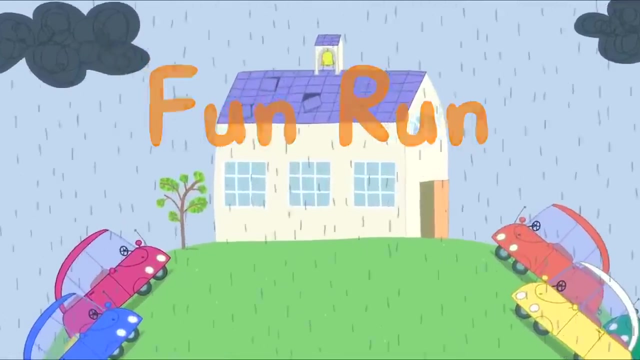 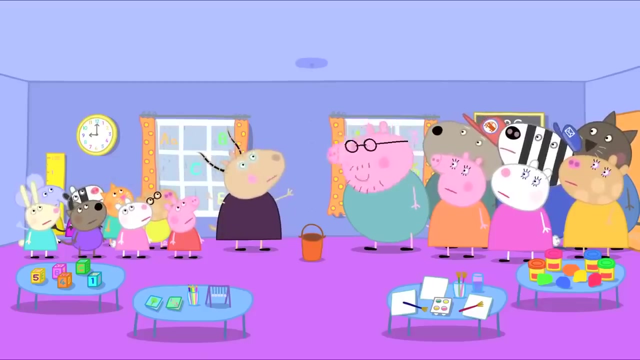 So did I. Maybe we did get a bit lost after all Fun run. It has been very stormy weather and the school roof is leaking. How can we raise the money to fix the school roof? We could have a fun run. What's a funny run. 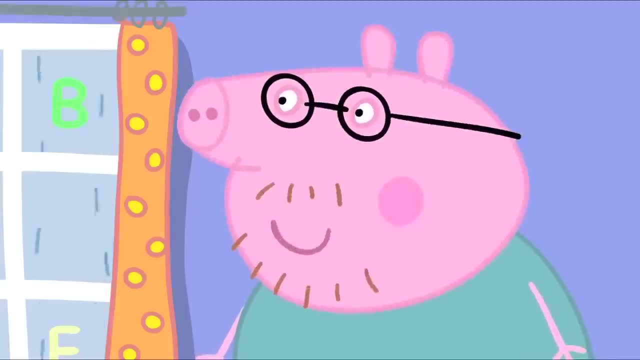 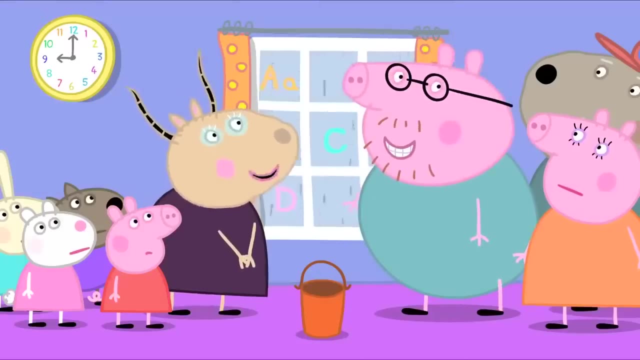 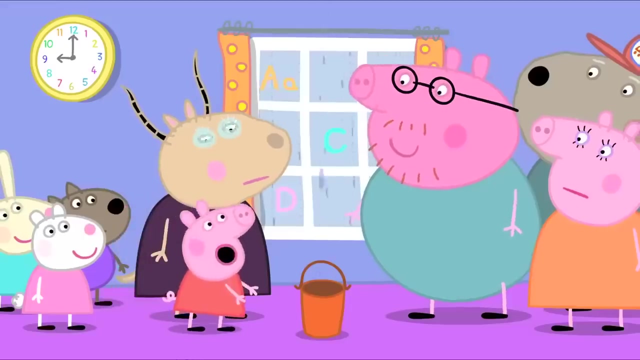 It's a day for picnics and giving money to see people run, And the more money you give, the further they run. Good idea, Daddy Pig. How far can you run? What? Well, I can run as far as you like, But, Daddy, you can hardly run at all. 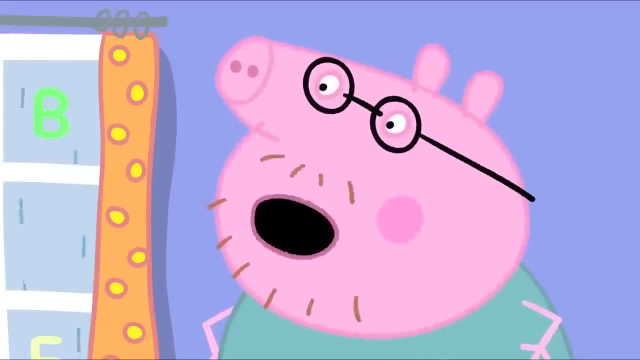 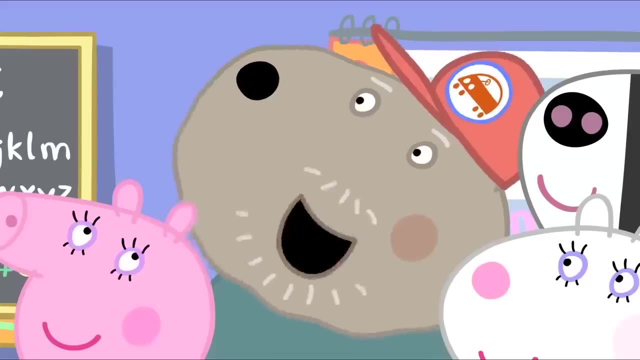 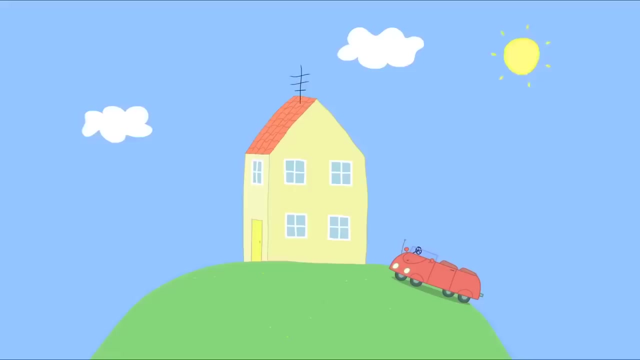 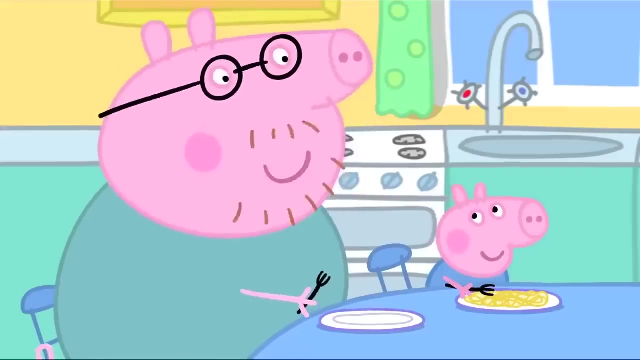 Nonsense. I'm an expert at running Good, Does anyone else want to run? No, thank you, But I'll give money to see Daddy Pig run Me too, And me- Excellent, Thank you, Daddy Pig. Peppa and her family are eating spaghetti- Delicious. Is there any more spaghetti? 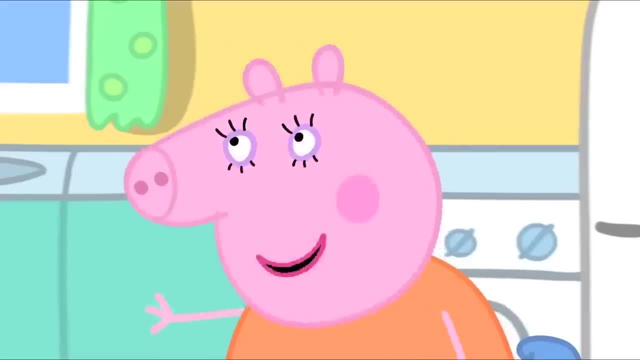 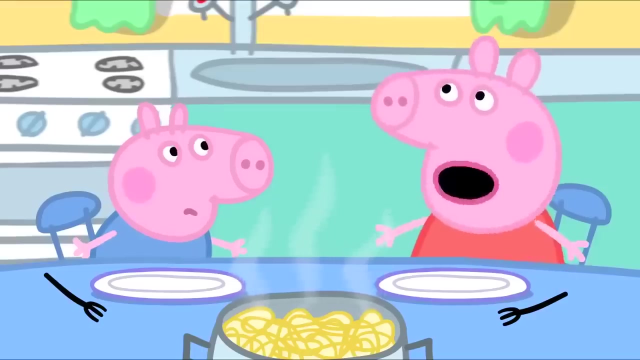 Daddy Pig, you've already had three helpings. Eating gives me energy And I need energy for my fun run. You also need to practice running. What if I practice eating today, then practice running tomorrow? No, Daddy, You need to practice running now. Oh, Come on, Daddy. 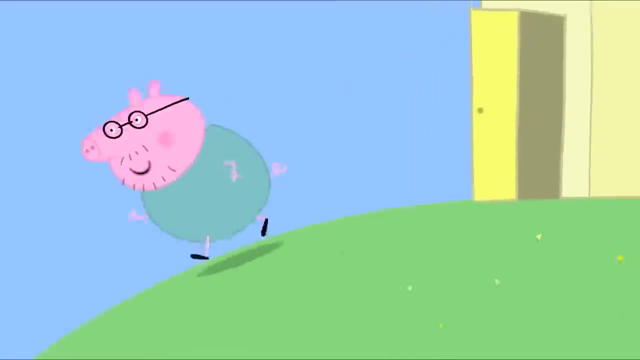 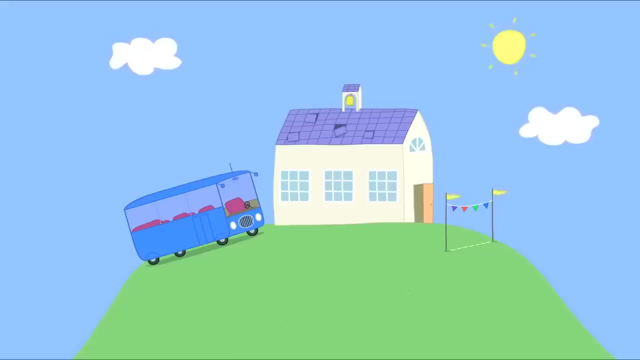 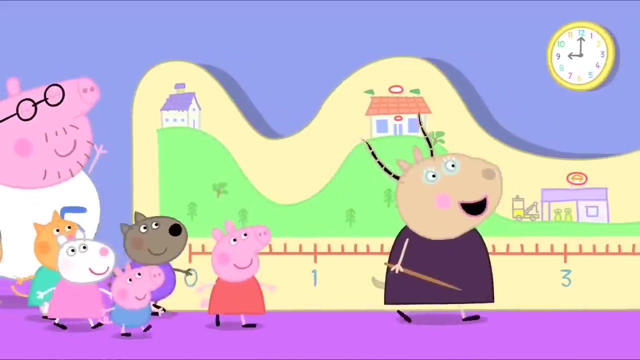 Race you. This is easy. It is easy to run downhill. It is hard to run uphill. I don't think I should have eaten so much spaghetti. It is the day of the fun run. Madame Gazelle has a chart to show how far Daddy Pig must run. If Daddy Pig can run to here. 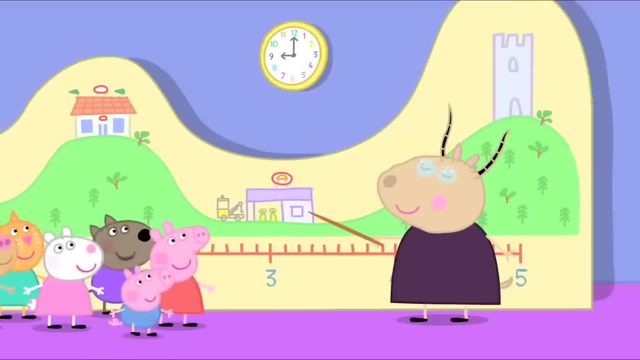 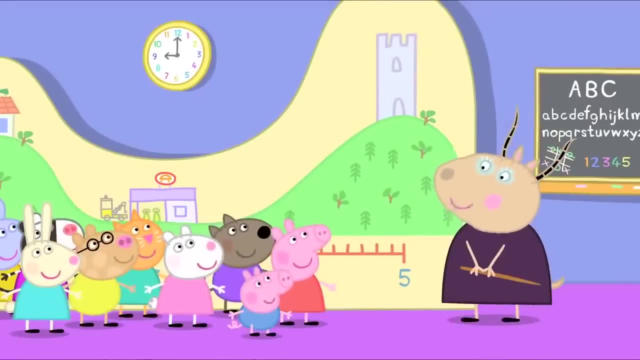 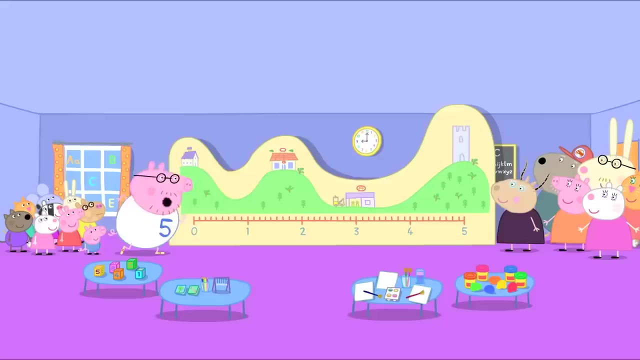 The supermarket, Then to here My Grandad's garage And all the way to here Windy Castle. Then we'll have enough money to fix the school roof. I'll do it now. Ready, steady go. I did it. Now we can have the picnic, Silly Daddy. 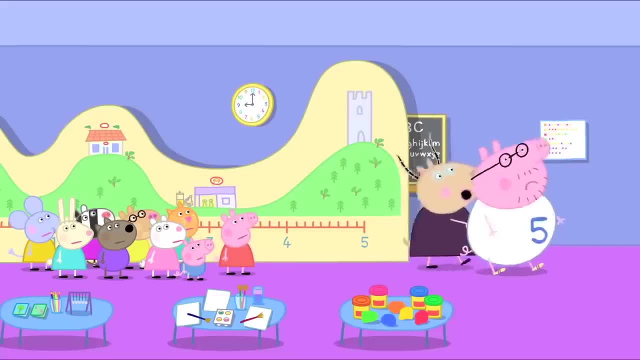 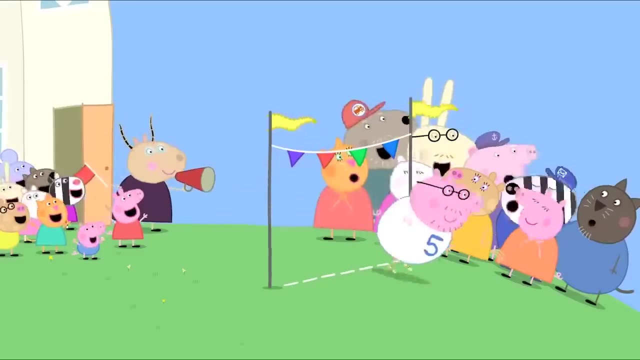 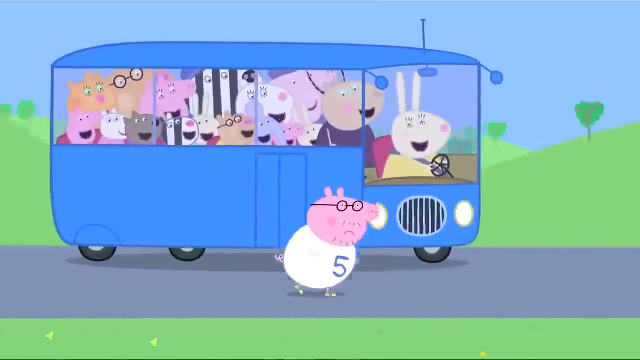 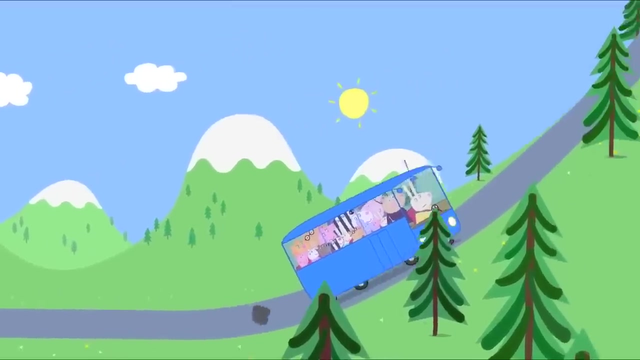 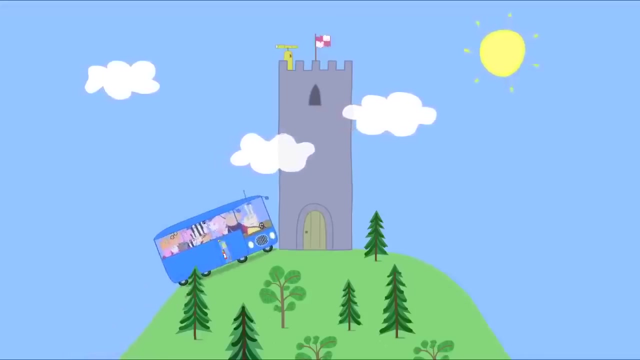 That's just a drawing. Yes, Now you must run to the real Windy Castle. Ready, steady, go Hurray. Come on, Daddy Pig, You can make it. Come on Pop, You can make it, You can make it. The school bus has made it to Windy Castle. 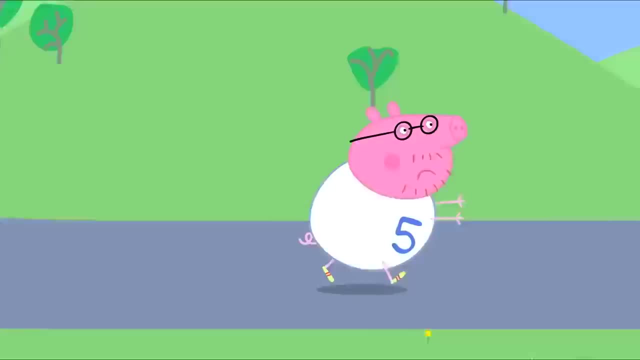 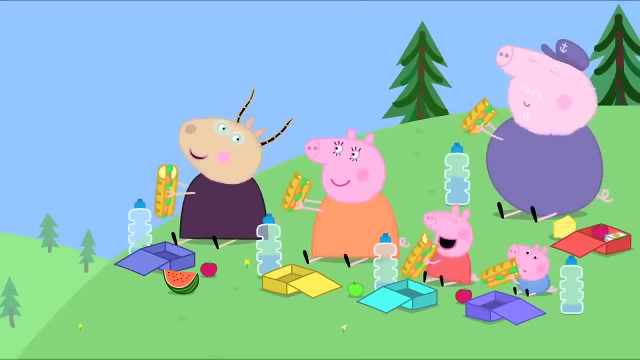 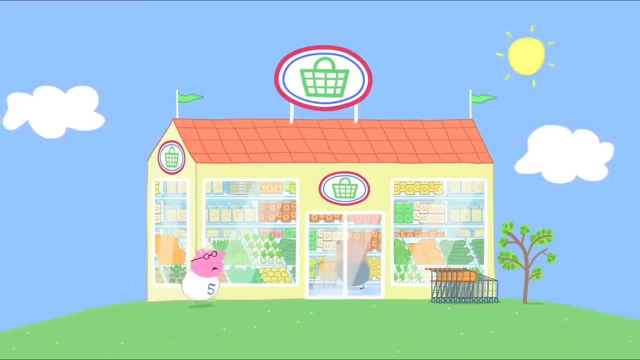 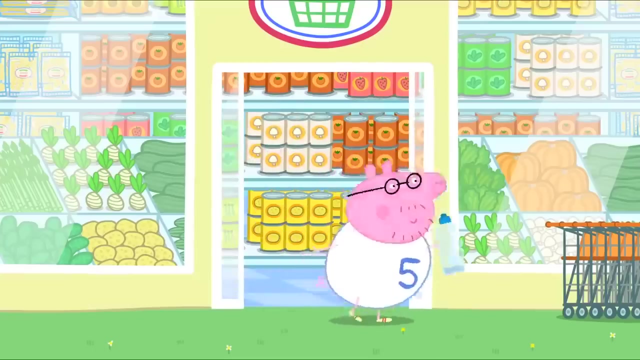 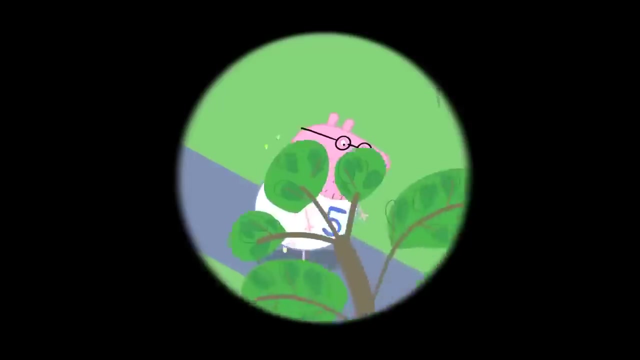 Now everyone can enjoy the picnic. Water water. What a lovely hot day And such a relaxing way to raise money too. Water water. Daddy Pig has reached the supermarket. All the running has made him very thirsty. Let's look through the telescope. I can see Daddy. The telescope makes everything look closer. 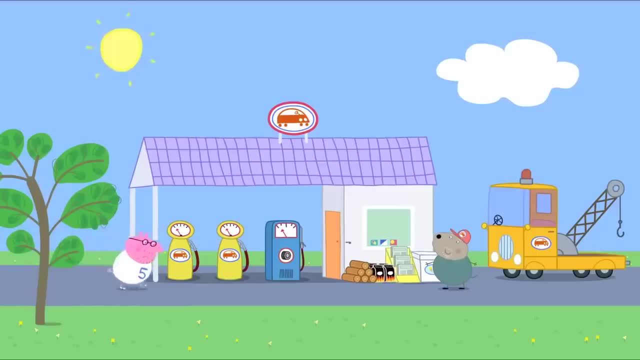 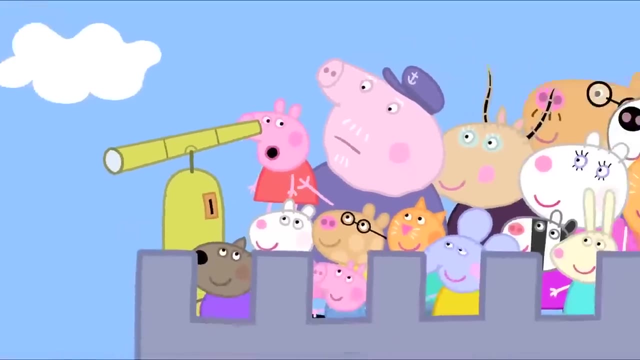 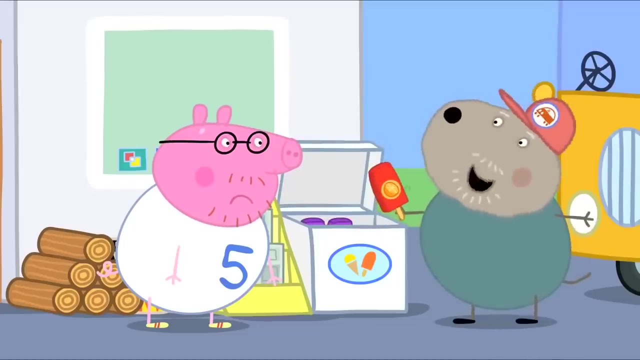 Oh, he's not going very fast. Daddy Pig has arrived at Grandad Dog's garage. That's it. I can't go on. Daddy has stopped. You look rather hot. You need something to cool you down and give you energy. Have an ice lolly. Thank you, Grandad Dog. 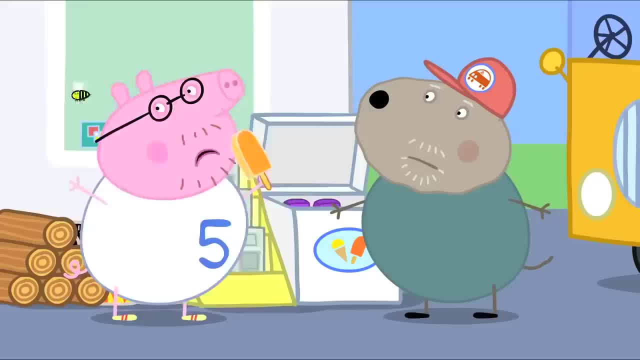 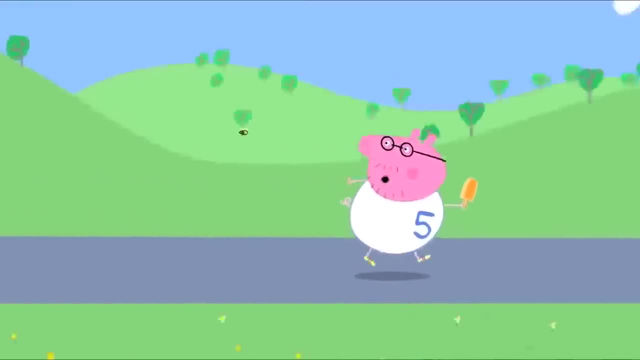 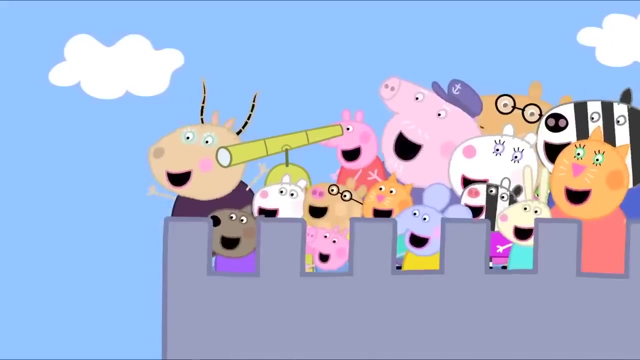 That's nice. Huh, a wasp Shoo shoo. Get away, you, little pest. The wasp wants to share Daddy Pig's ice lolly. No, this is my lolly. Daddy started running again Really fast. Hurray, Get off, get off. 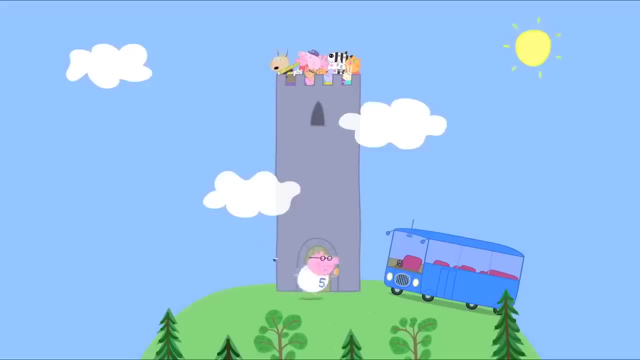 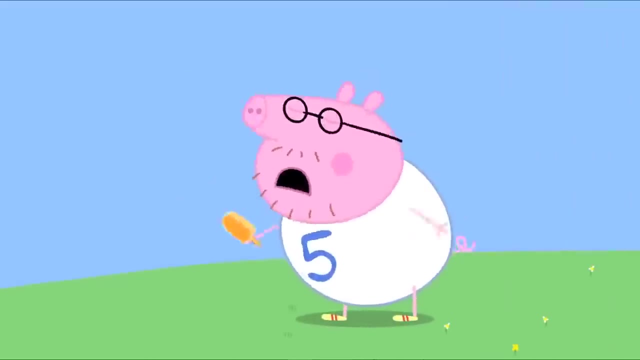 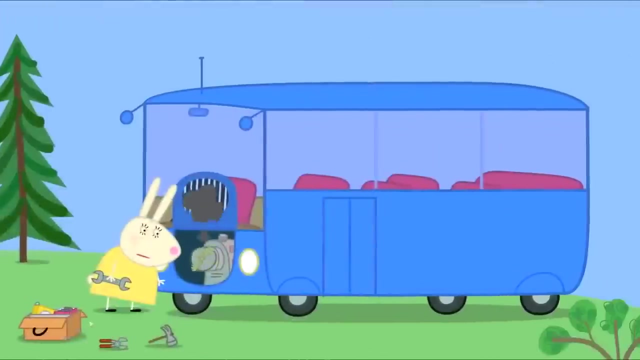 You can stop now, Daddy Pig. We have enough money to fix the school roof. Daddy Pig has lost the wasp. Well done, Daddy Pig. All that extra running means we've got enough money for a new school bus too. Thank you, Daddy Pig, You're most welcome. 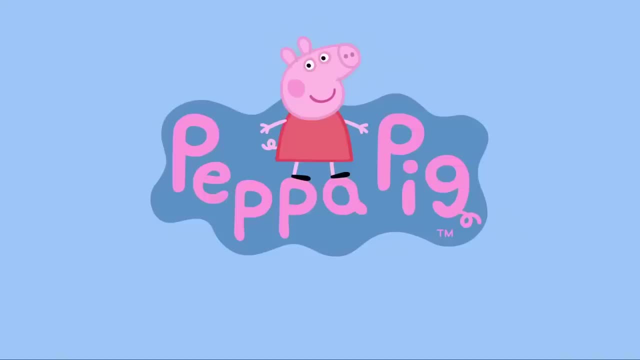 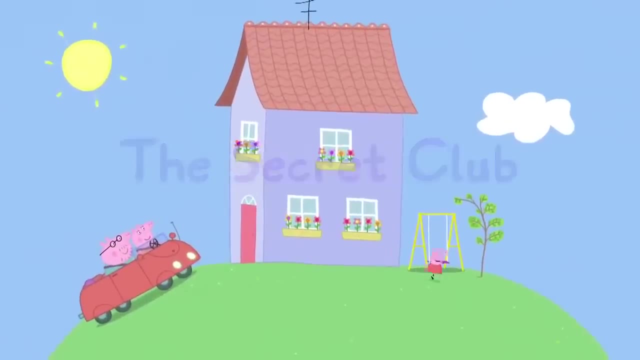 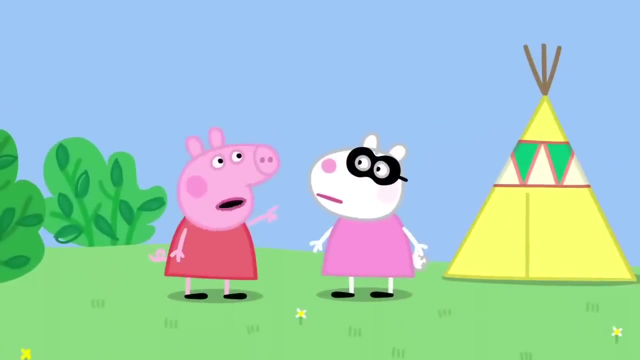 You're most welcome. The Secret Club Peppa has come to play with Suzy Sheep. Hello Suzy, Hello Peppa. Why have you got that mask on your face? So people don't know it's me? I'm in a secret club. 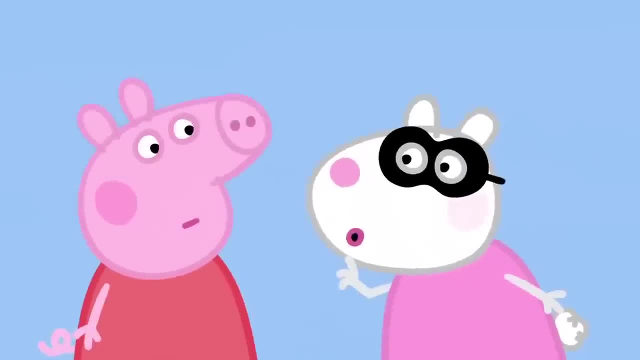 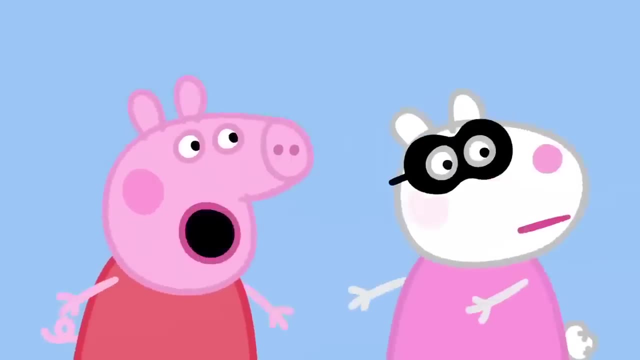 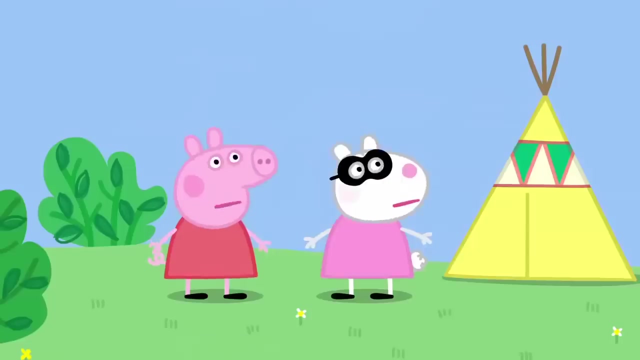 Can I be in your secret club? Shh, It's not easy to get into. You have to say the secret word. What word? Flubberdobble, Flubberdobble. Right, you're in. Danny Dog has come to play. Hello Peppa. 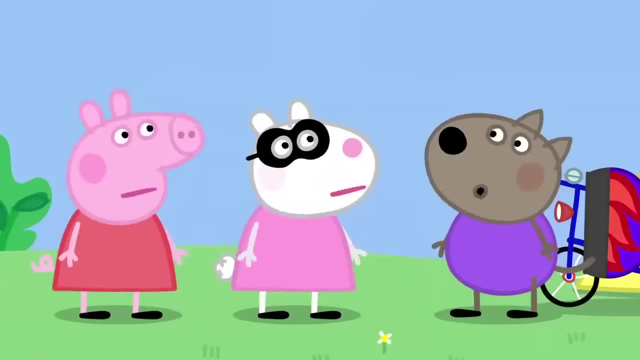 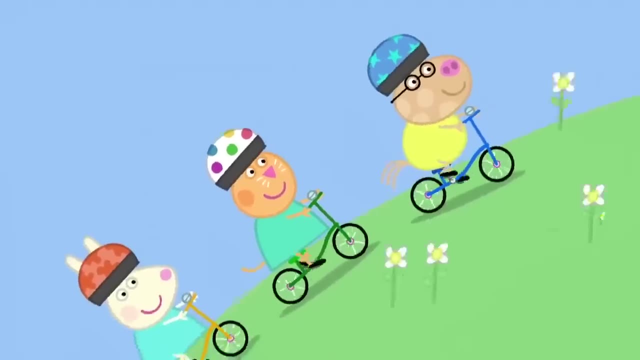 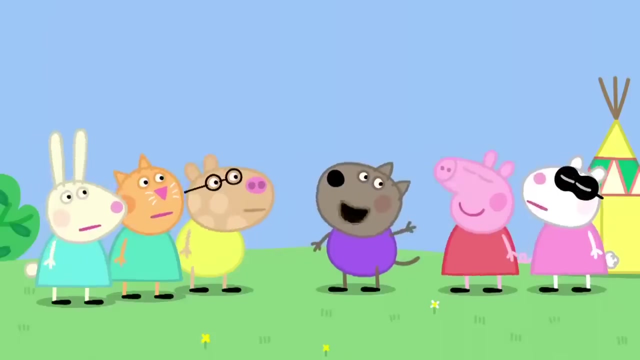 Hello, Suzy, Shh What. I'm in a secret club, I'm in it too. Ooh. Pedro Pony, Candy Cat Suzy Sheep and Rebecca Rabbit have come to play. Hello, Shh. Suzy and Peppa are in a secret club. 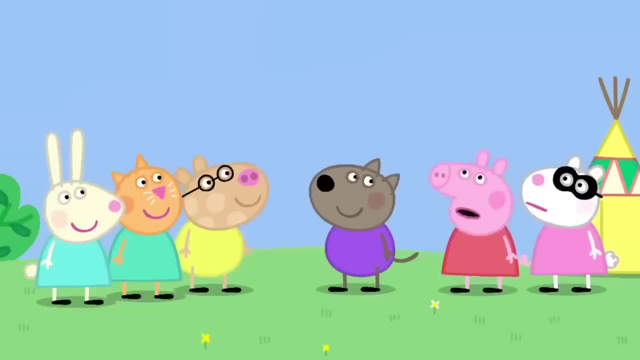 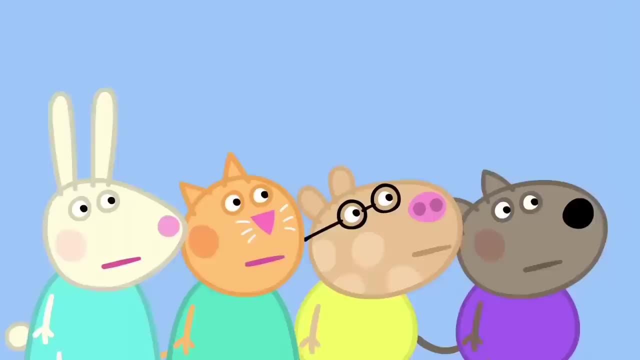 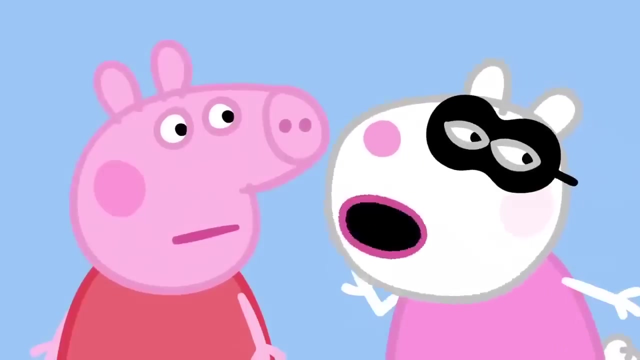 Can we join your secret club? It's very hard to get into. You have to say the secret word: Shalamakookie, Shalamakookie. That's not the word I said. It changes all the time to keep it secret. Oh, Are we in the secret club now? 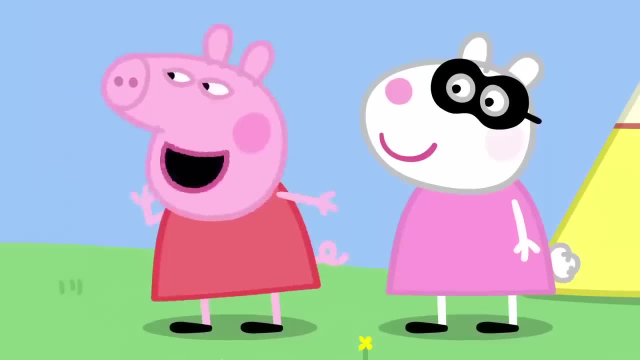 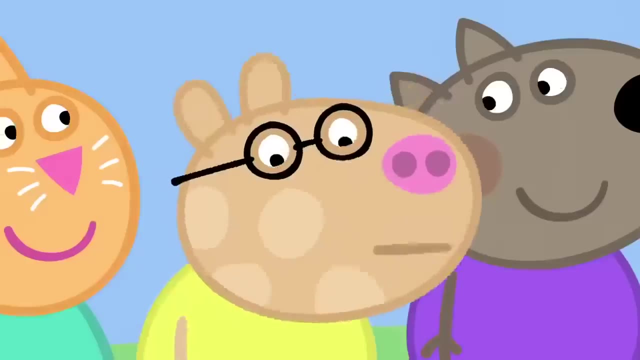 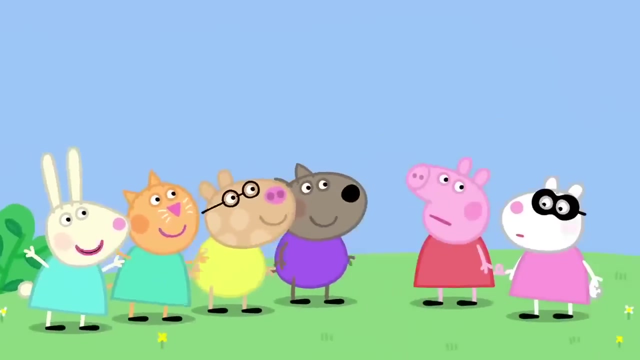 We are in. What do we do? We do secret things in secret And secretly go on secret missions. I don't know what you're talking about. Show us how you do a secret mission. Yes, show us, Er Peppa can do it. You've got the mask on, Suzy. 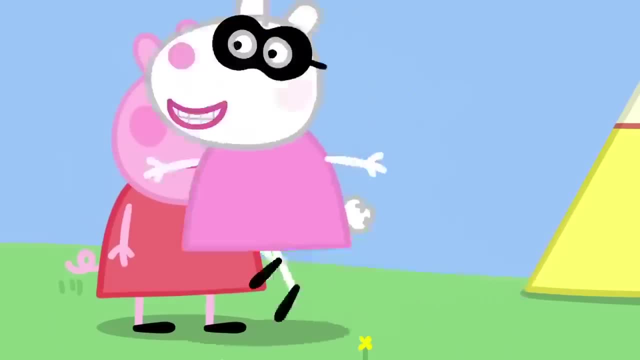 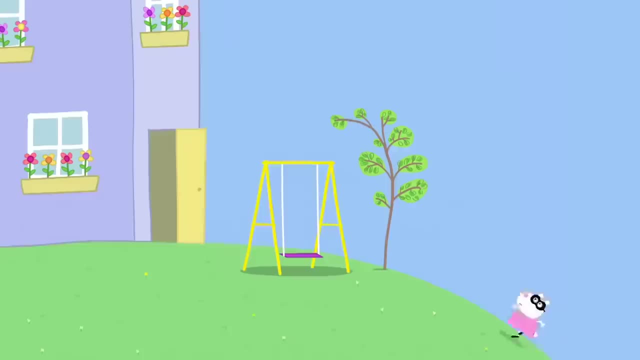 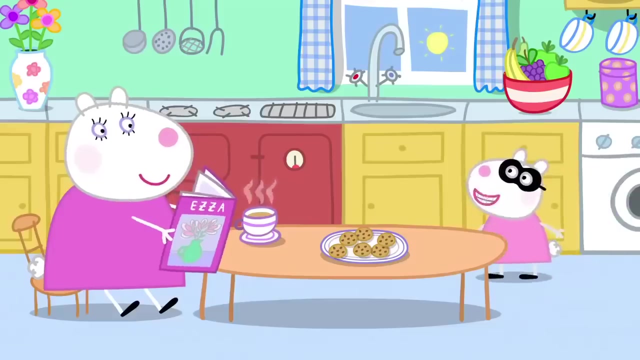 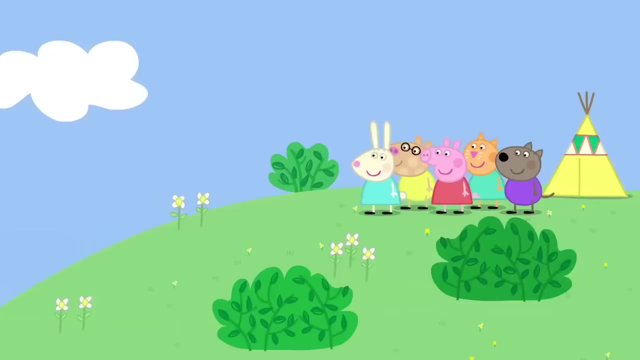 OK, my secret mission is to get biscuits. Watch, this Suzy Sheep is trying not to be seen. Mummy, can I have some biscuits for my friends please? Of course, here you are. Thank you, Mummy. Suzy Sheep has returned with the biscuits. 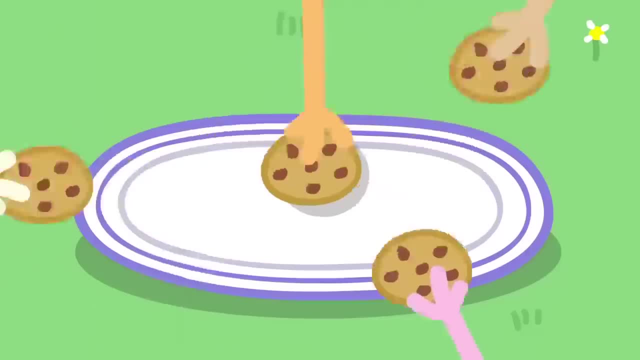 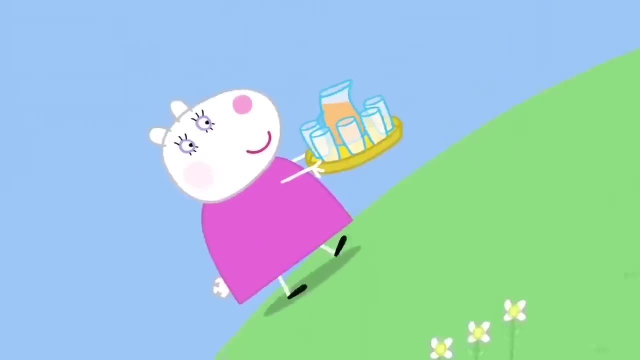 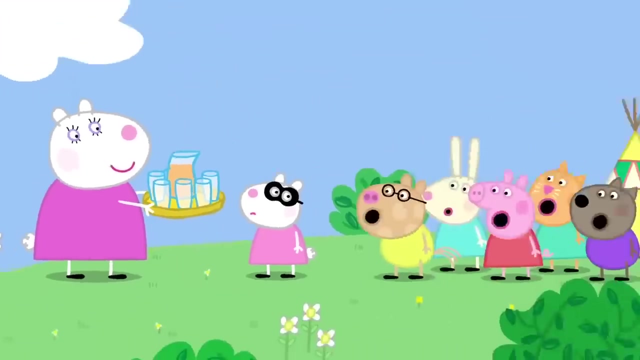 Hooray Shh Hooray. Did anyone see you? No, Well, only a grown-up. Look out. Would you like some juice to go with your biscuits? What biscuits? The biscuits I just gave you for your friends? Oh, Suzy. 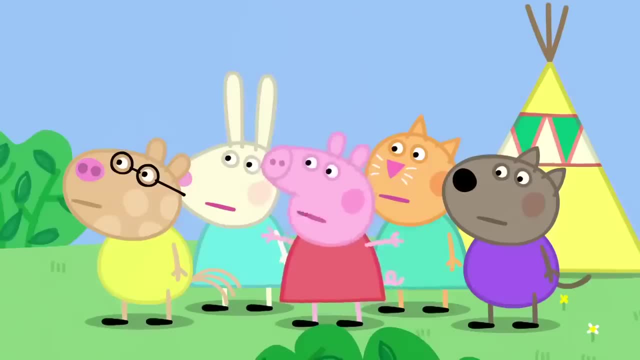 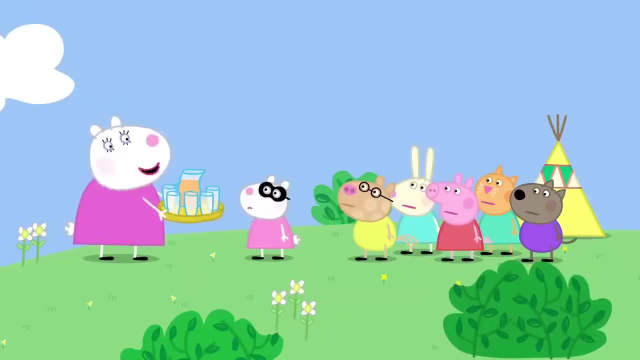 What's the matter? We're in a secret club doing secret things And Suzy's told everyone: Oh, can I be in your secret club please, Please. I've always wanted to be in a secret club. It's very hard to get into. 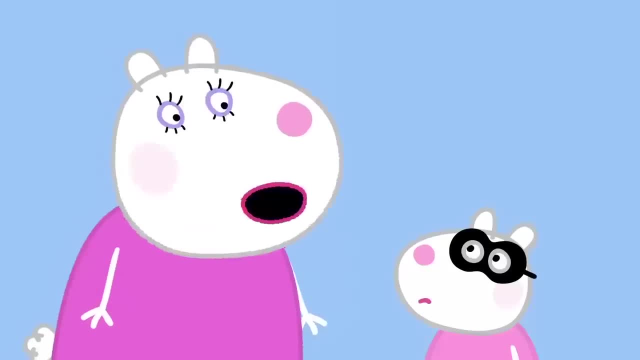 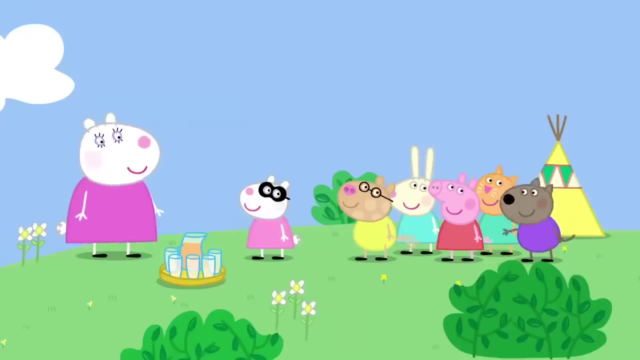 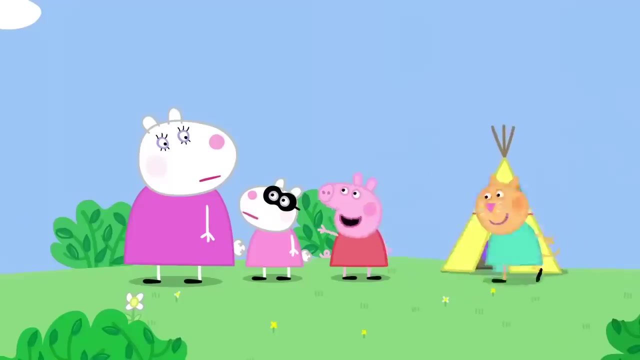 You must say the secret word, Which is: Pick a needle noodle. Pick a needle noodle, That's it. You're in What happens now? Look out, It's Daddy Pig. You talk to my daddy, But don't say anything about our secret club. 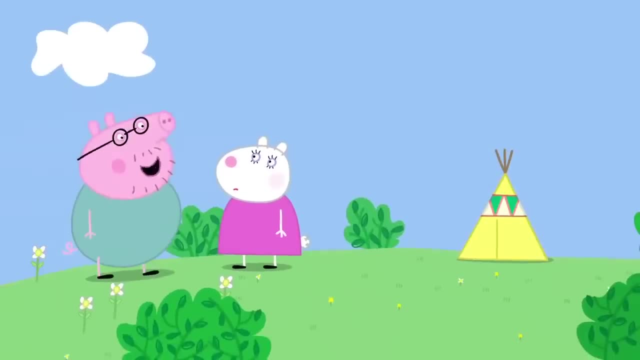 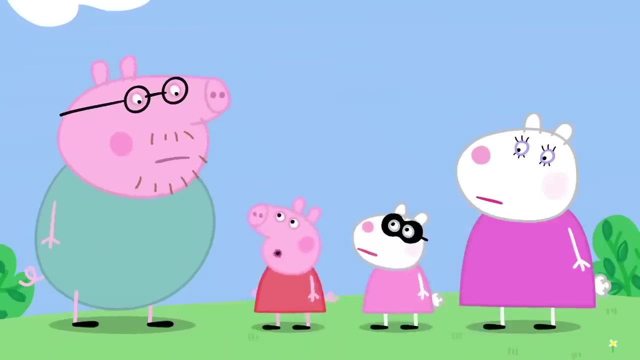 Hello, Ah, there you are, Mummy Sheep. What's new? Er erm er er. Secret club. Oh no, Oh, I always wanted to be in a secret club. Can I join, please? You can't join, Daddy, Because you are grown-up. 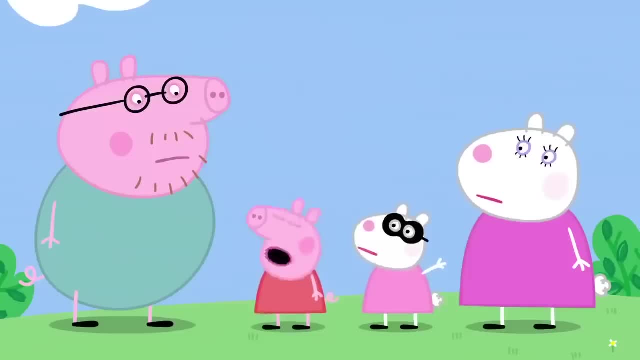 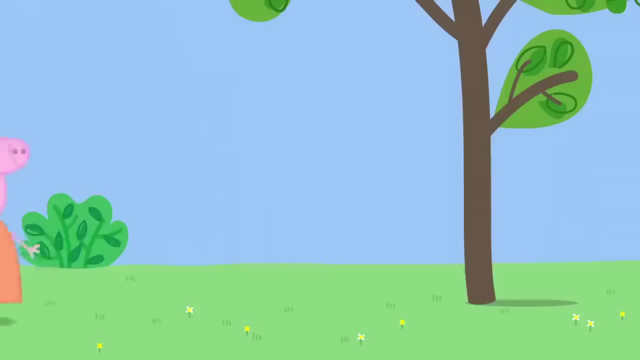 Er, my mummy is grown-up. Well, you have to know the magic word, Which is Papa-deedle-doodle-dum. Papa-deedle-doodle-dum, You're in. What do I do now? Look out, It's Mummy Pig. 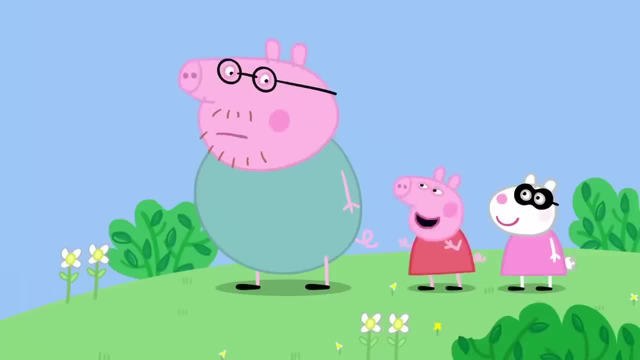 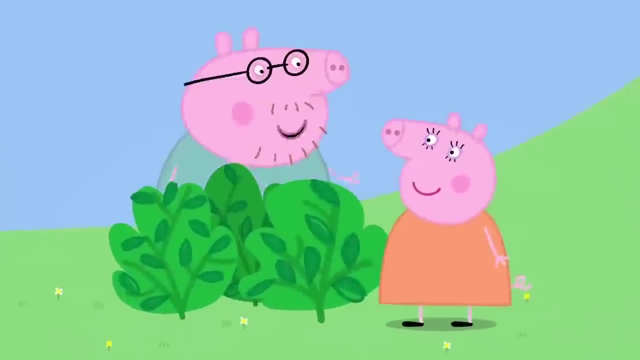 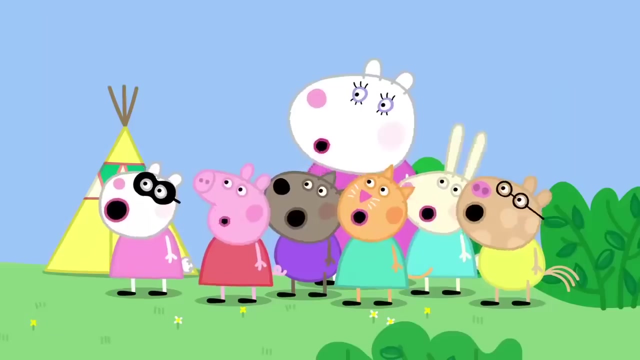 It's Mummy Pig. Follow Mummy in secret. Daddy Pig. Ah, hello, Mummy Pig. What are you doing in that bush Erm er secret club? Oh, I've always wanted to be in a secret club. We can't have everyone in the secret club. 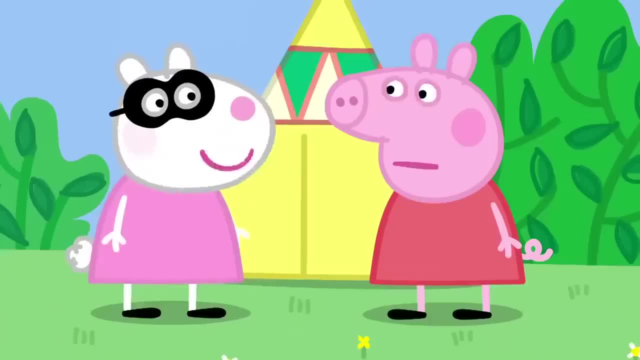 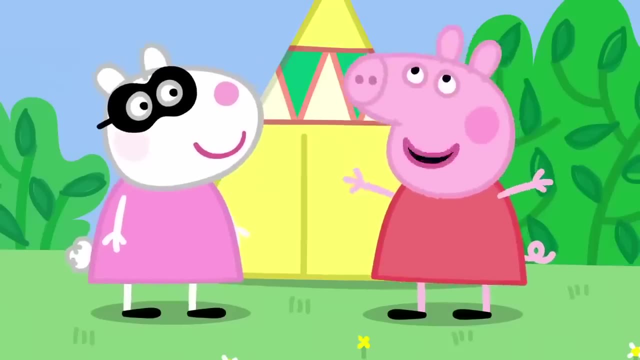 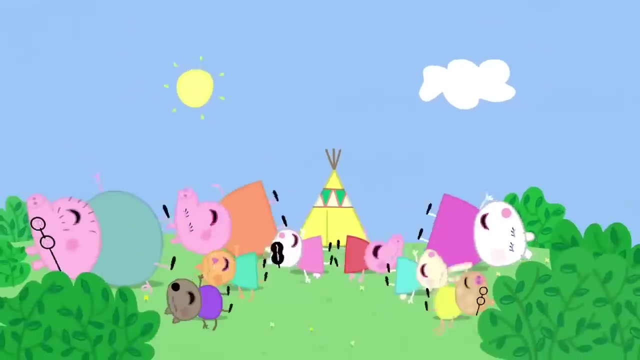 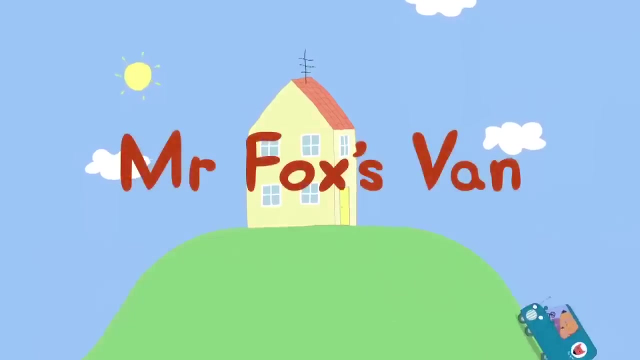 It wouldn't be a secret. Oh, I suppose it doesn't have to be a secret club. It can be the everybody secret club And everybody can be in it. Oh goody, Mr Fox's van. It is a lovely sunny day. Peppa is playing with her friends. 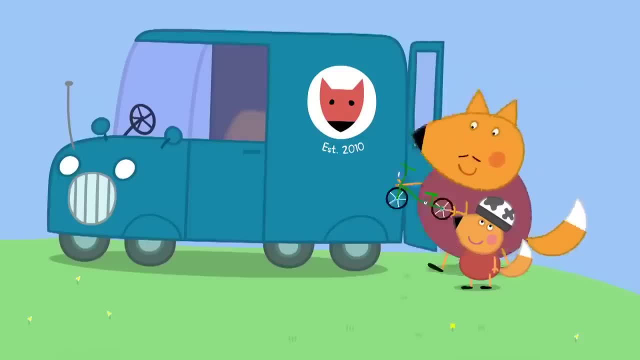 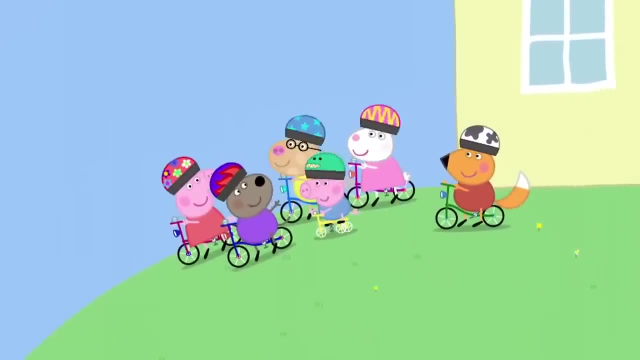 It's Freddy Fox. Hello everyone. Hello Freddy, Come on, Let's cycle through the big hill. Yay, Good morning, Mr Fox. It's afternoon, Mr Pig, Afternoon. Already, My watch must have stopped. My shop sells watches and clocks. Let me see what I've got in the van. 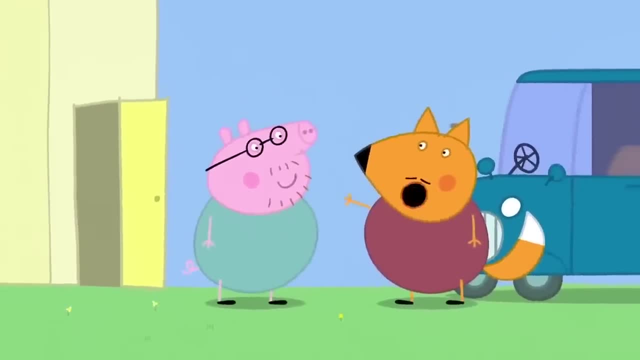 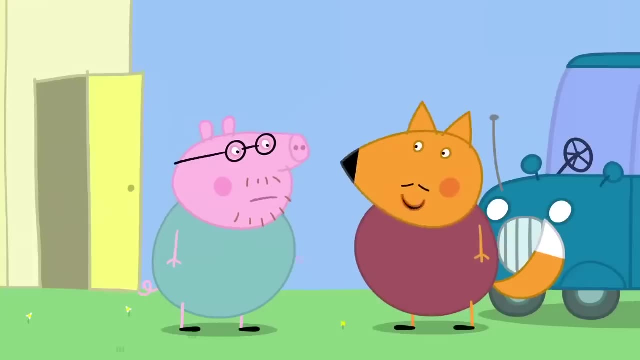 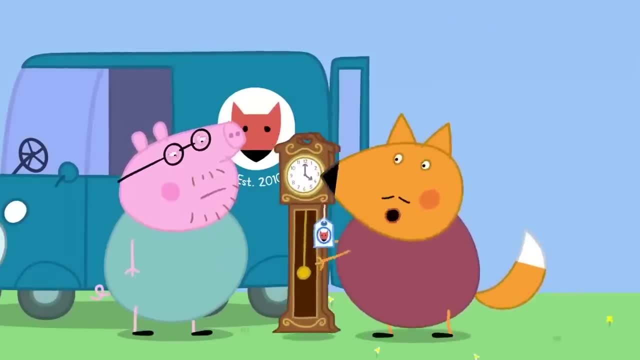 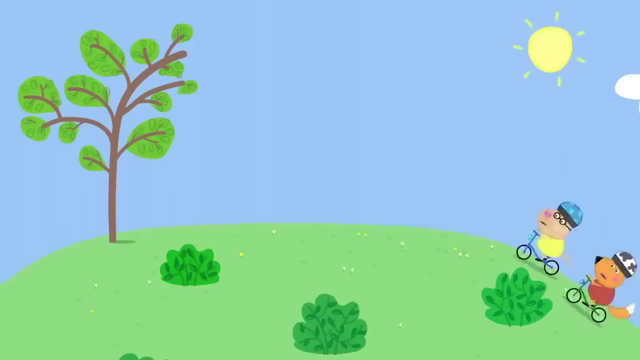 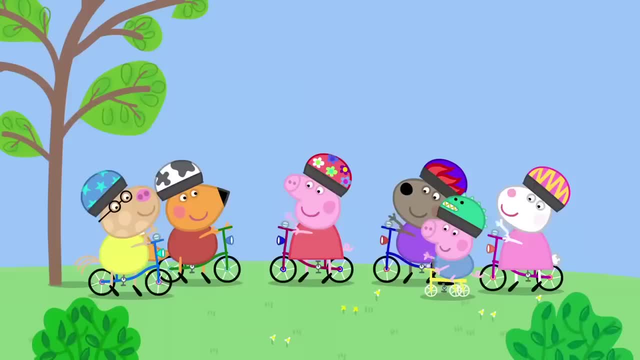 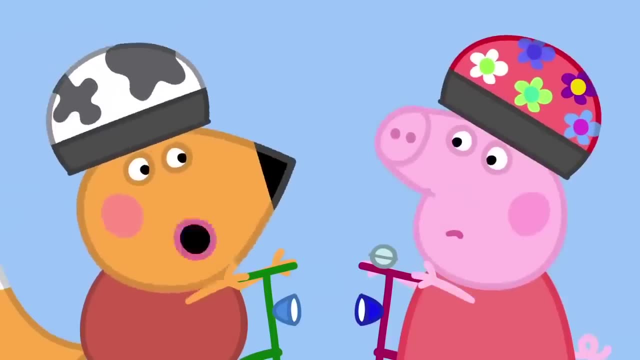 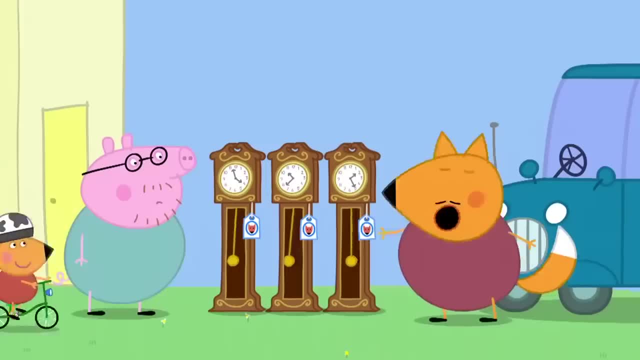 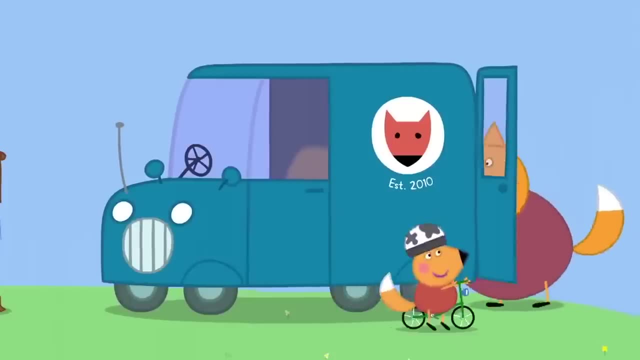 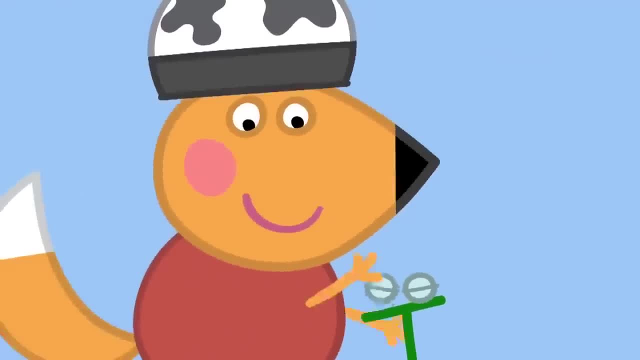 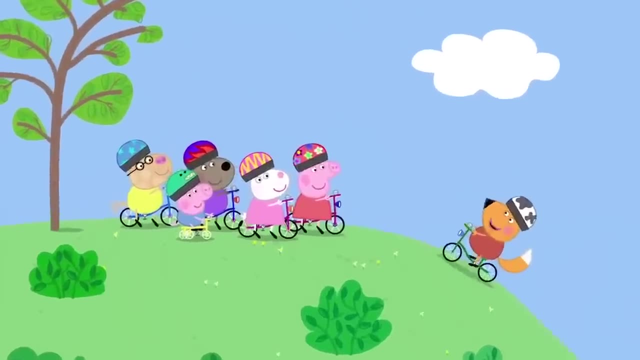 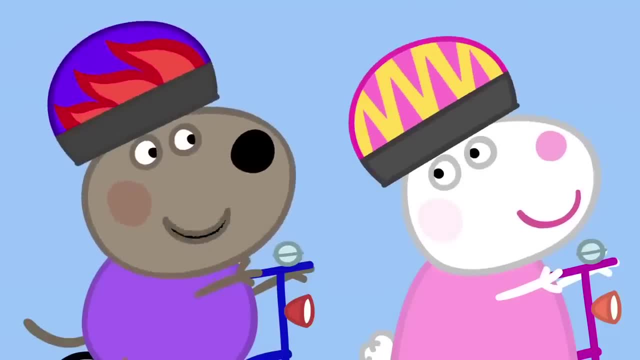 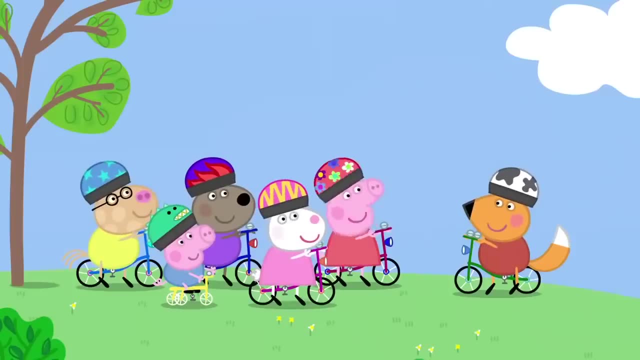 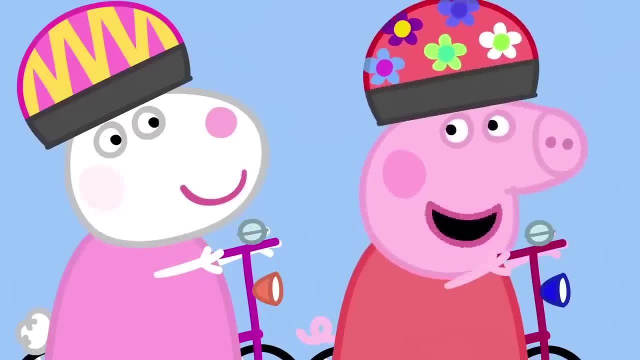 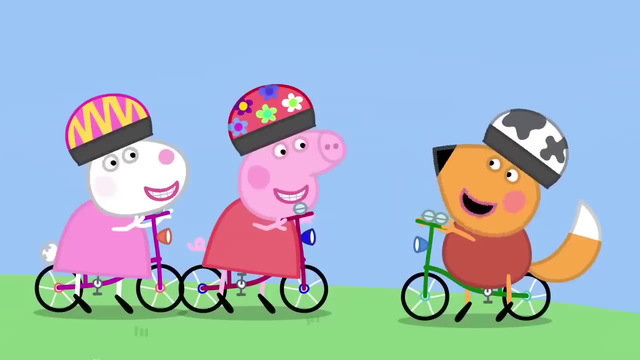 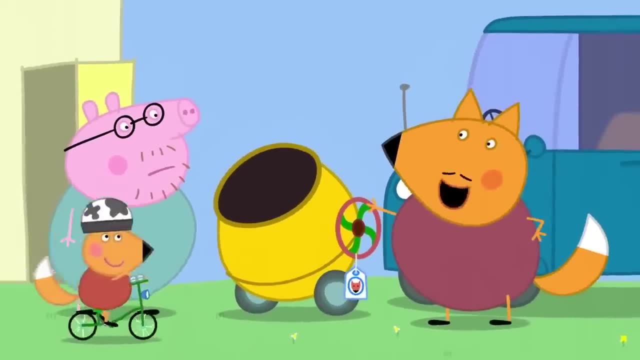 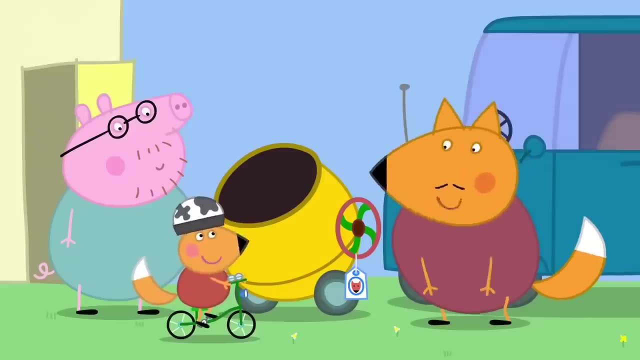 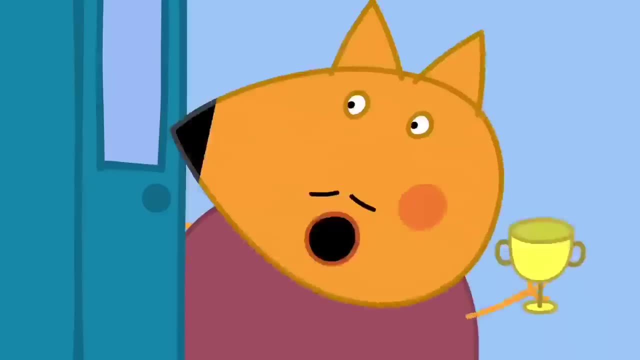 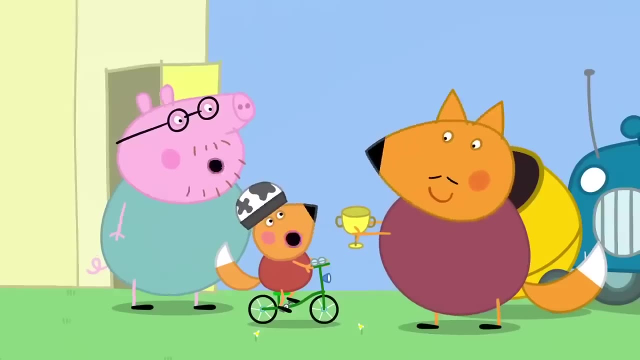 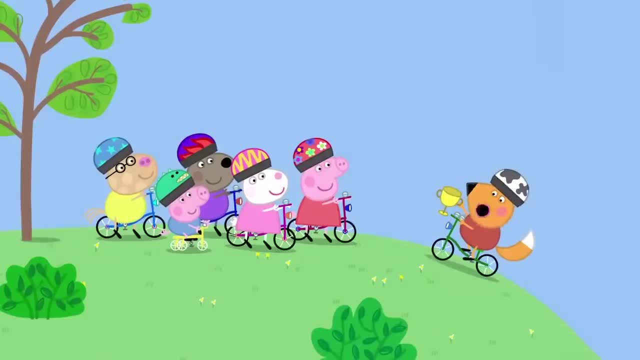 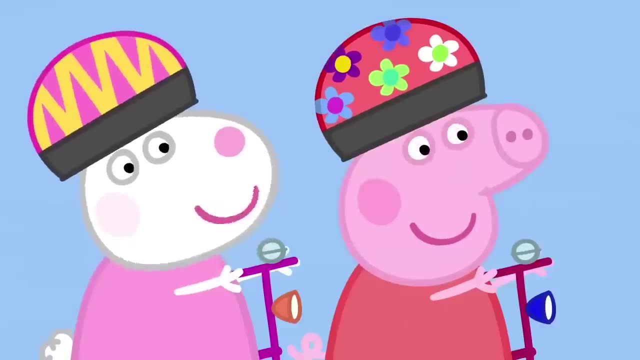 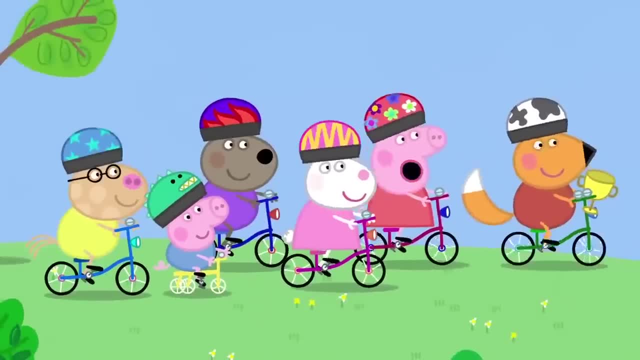 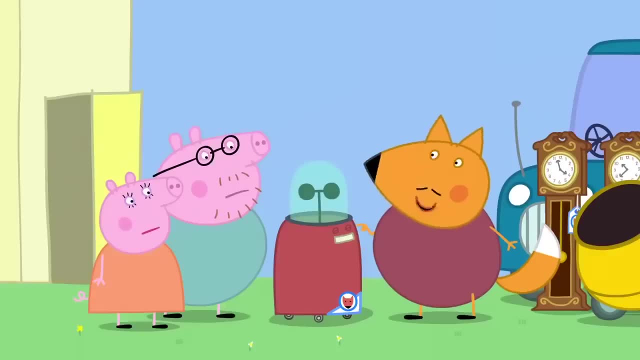 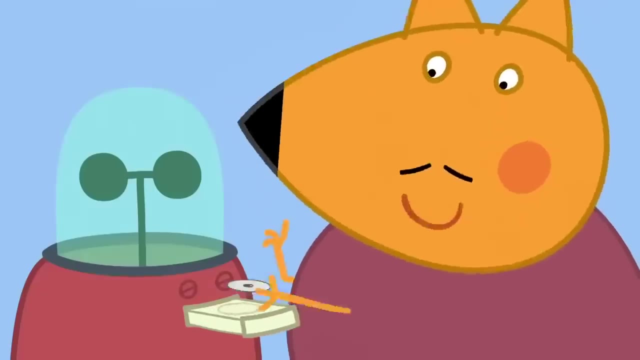 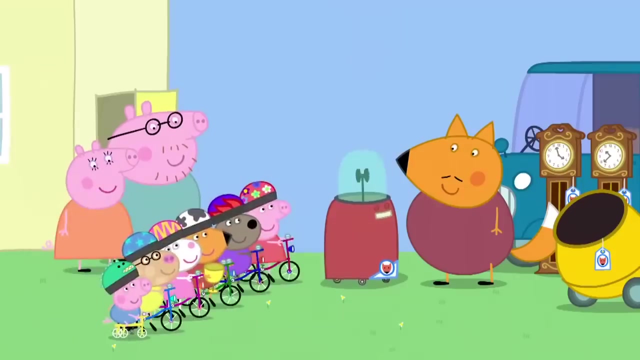 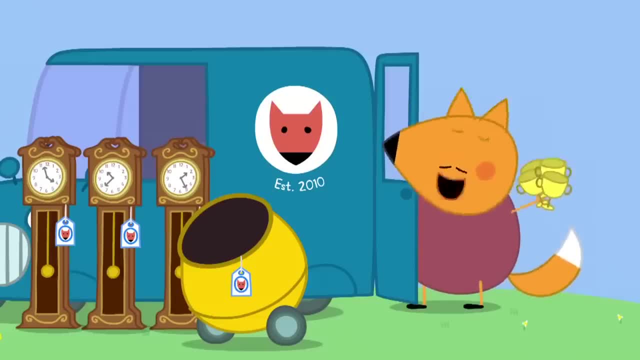 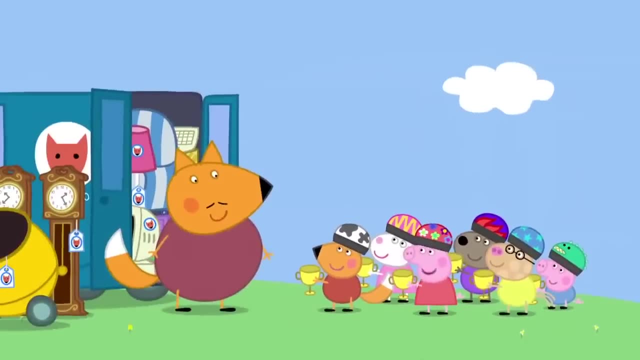 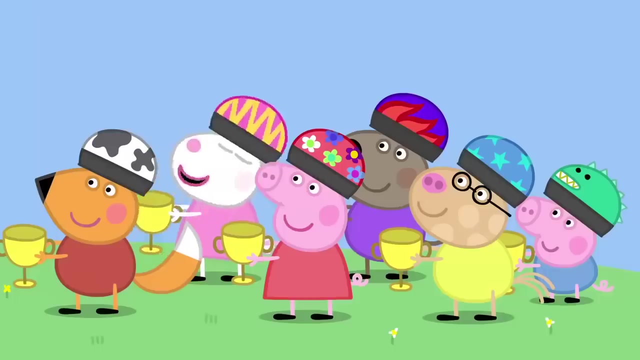 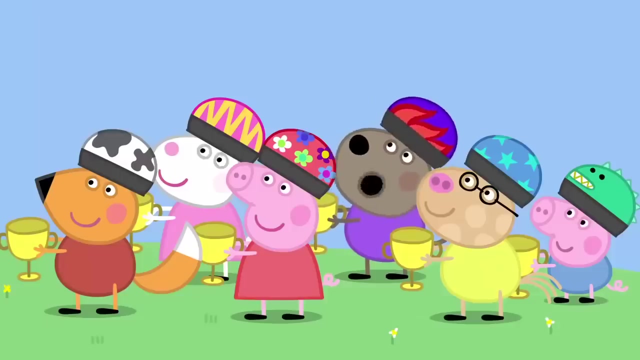 My van has a winner's cup for everyone. Mr Fox, is there anything you don't have in your van? Try me, Have you got a banjo Four or five string? You won't have a tree in your van, Apple or pear. I bet you haven't got a rocket in there. 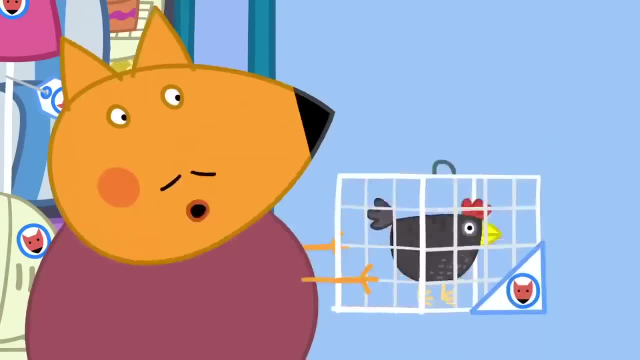 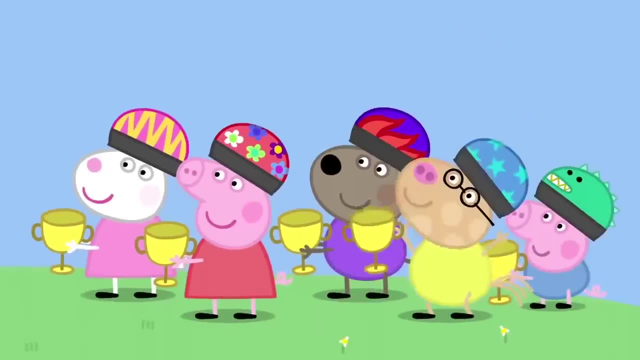 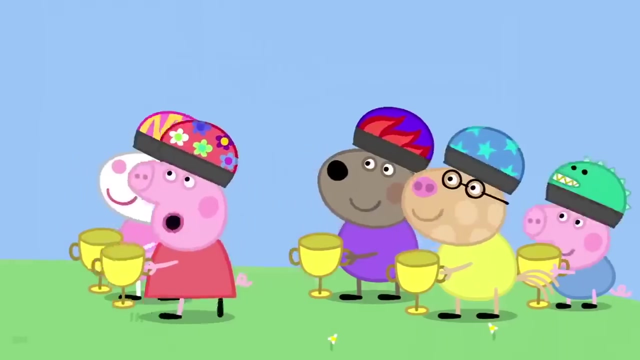 Boxes of five. What about a chicken? One chicken. Mr Fox's van is magic, It's a super van. Yes, it is. Come on, Freddy, we'd better get home Bye. Have you got a bouncy castle? Yep. A garden shed? Yep, I've got everything. 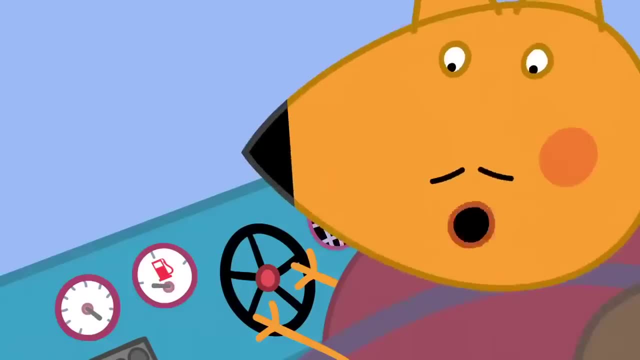 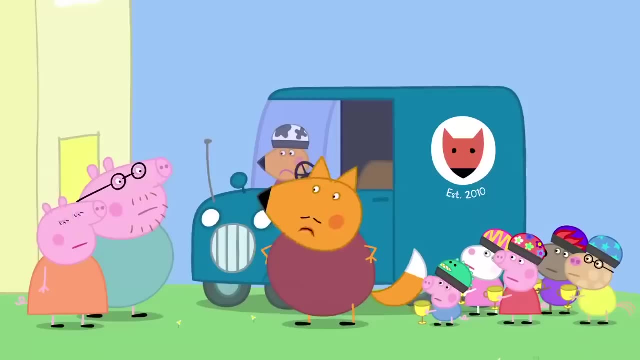 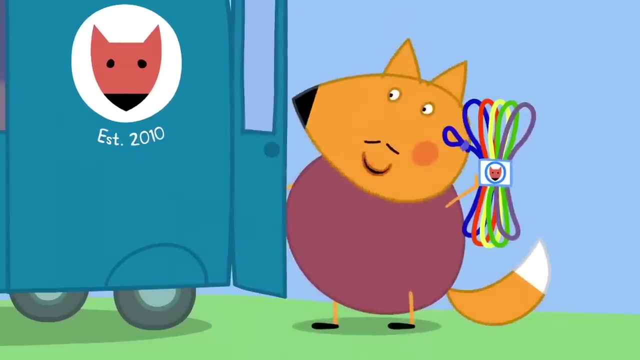 Oh, I've got no petrol. Mr Fox has everything in his van Except petrol. Hmm, I need to get to the petrol station. I would tow you, but I haven't got a tow rope. Oh, I've got plenty of them. I do them in packs of five. 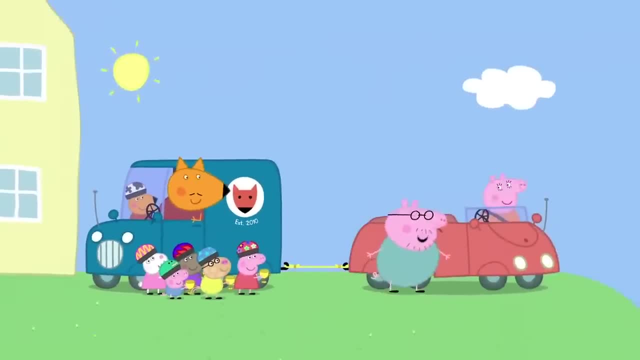 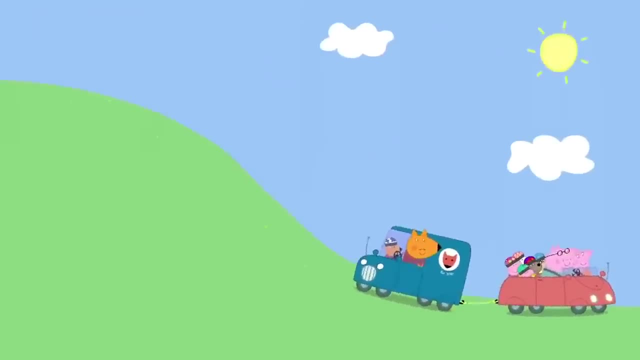 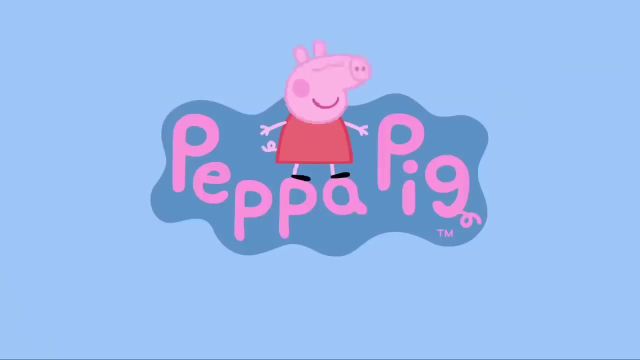 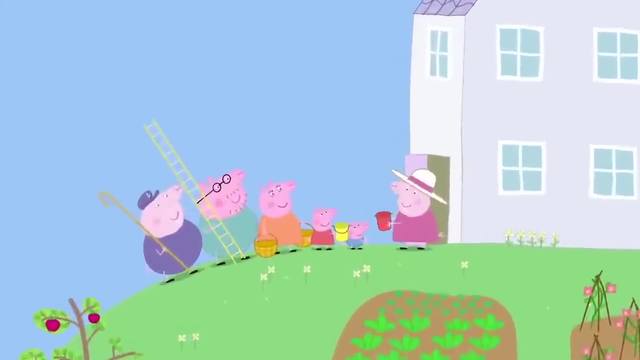 Can we come along too? Haha, why not? Daddy Pig is towing Mr Fox's van to the petrol station. Hahaha, Yep, Yes, Heheh, Phew. The Blackberry Bush, Peppa and her family are at Granny and Grandpa Pig's house. 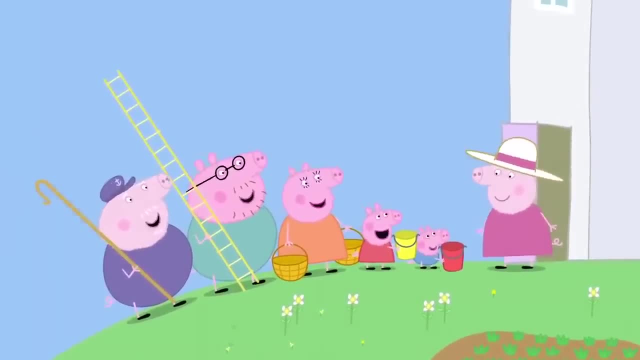 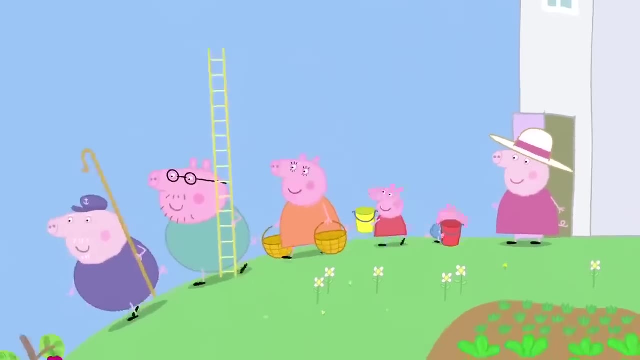 Today I'm going to make apple and blackberry crumble. Yummy. I need you brave explorers to go and get the fruit. Aye, aye, Granny Pig, We've got baskets for the apples And buckets for the blackberries. 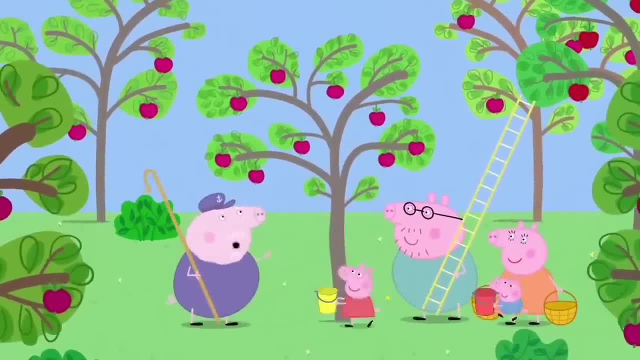 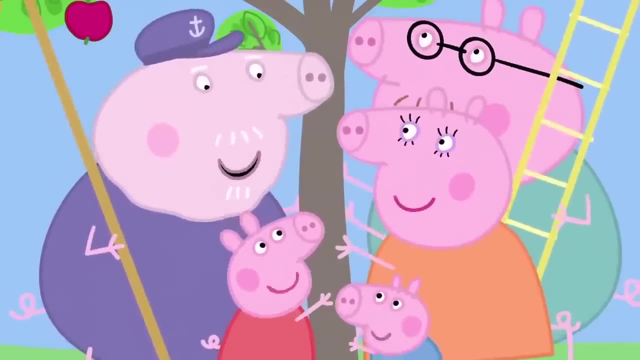 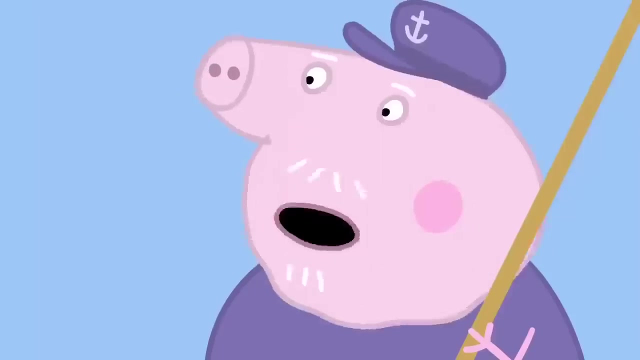 First the easy bit: picking apples On the count of three, shake the tree, One, two, three. Now for the blackberries. Why don't we just have apple crumble, Because blackberries are tasty too, Grandpa. 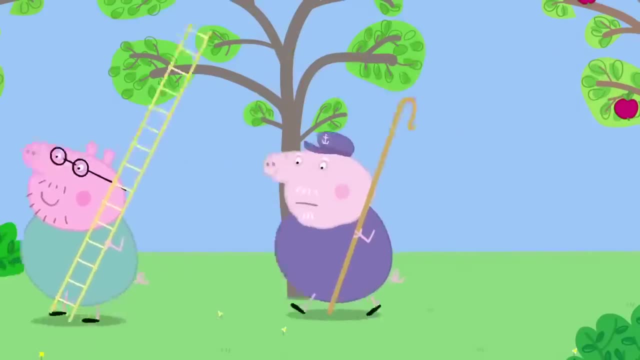 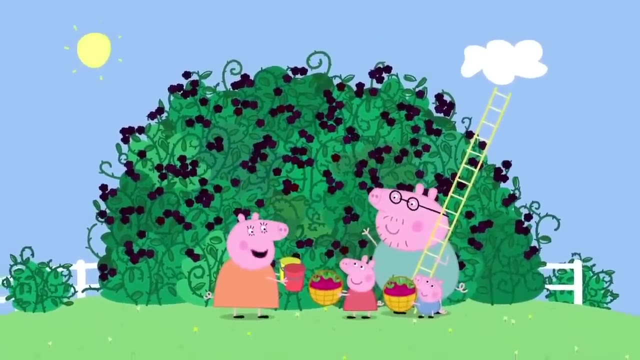 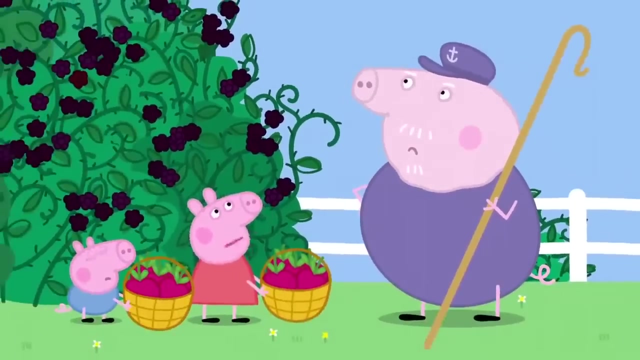 OK, now the hard bit. Now that's what I call a blackberry bush. This bush has been here since I was a little piggy. It's an overgrown weed. I should have cut it down years ago, Grandpa, why don't you like it? 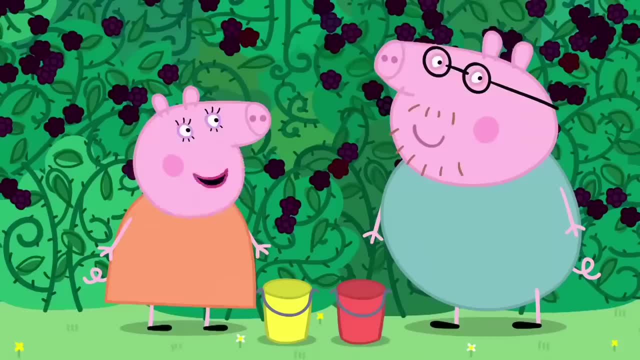 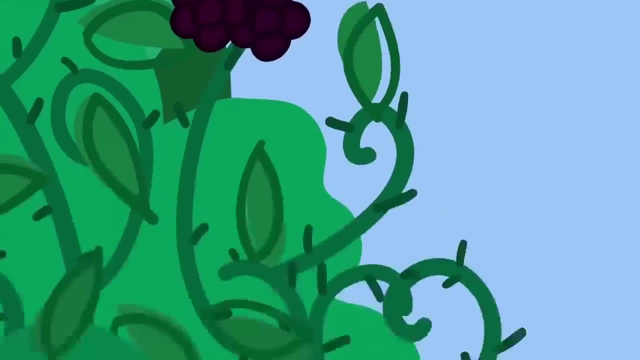 I don't like the way it looks at me. Silly Grandpa, it's just a harmless bush And it's covered in lovely blackberries. George has seen some really big juicy blackberries. Careful, George, or you might get tangled. 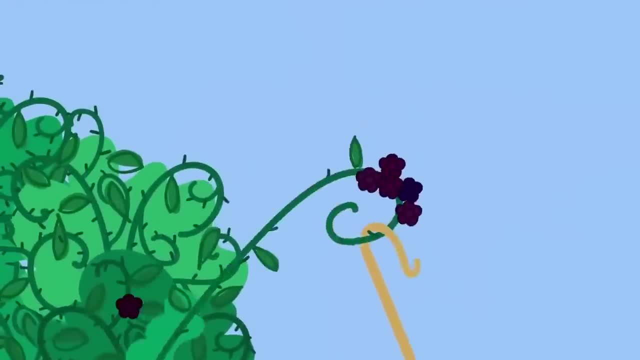 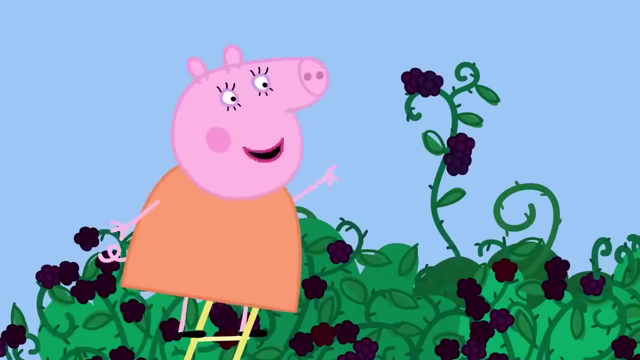 I have a stick for pickings. You're not making hard to reach blackberries, Clever Grandpa, But the best blackberries are right at the very top. That's why I've brought the ladder. Um, don't lean too far over Mummy Pig. 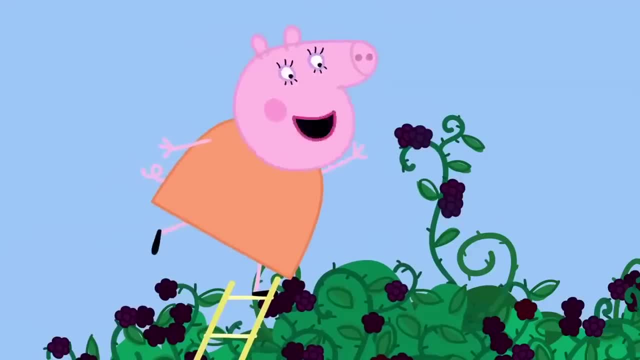 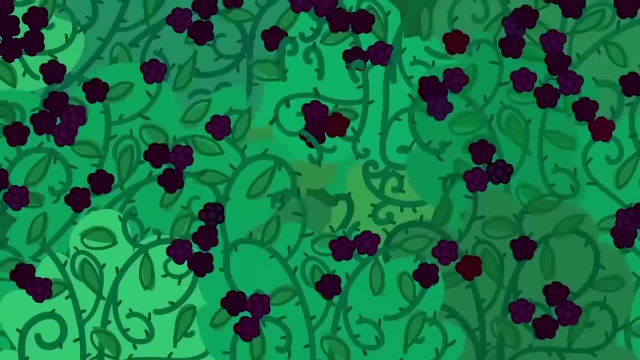 Don't worry, I've been climbing this blackberry bush since I was a little girl. Yes, but you're not a little girl now. I know what I'm doing. Oh, dear Mummy, Pig has fallen into the blackberry bush. 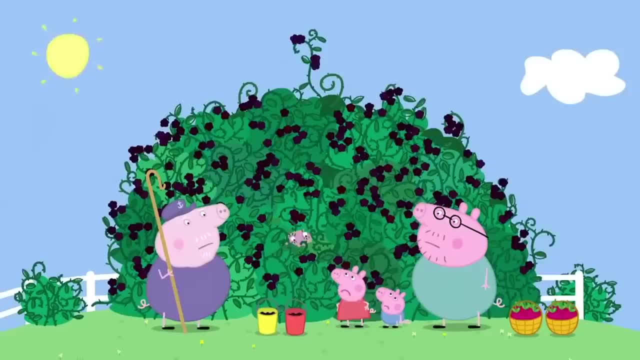 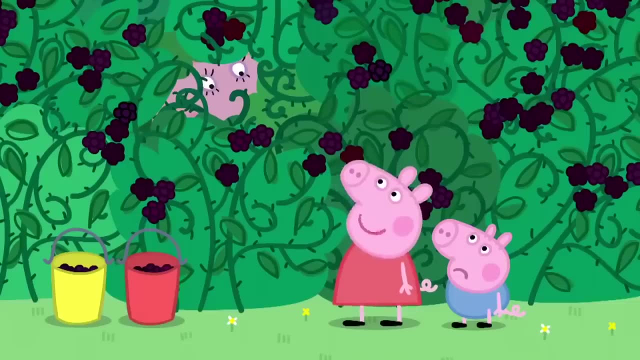 Mummy, can you get me a stick? Mummy, can you get out? Uh, no, I'm stuck. You're stuck in a thorny bush like Sleeping Beauty. What? Once upon a time there was a princess called Sleeping Beauty. 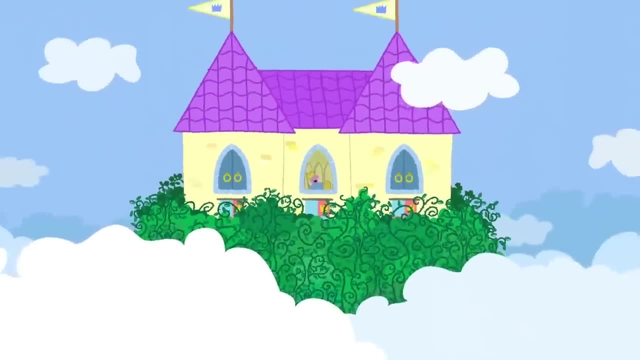 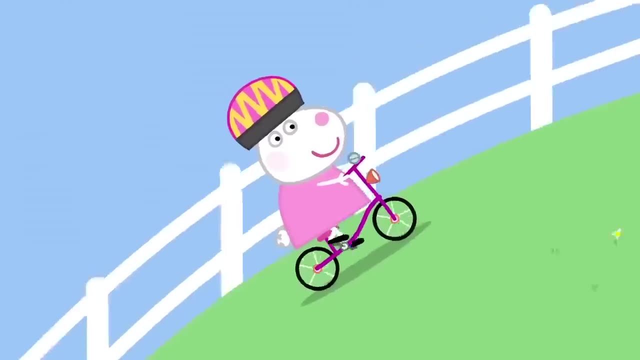 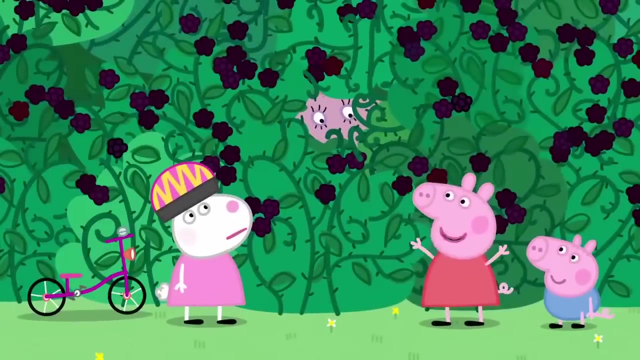 One day she fell asleep in a thorny bush and she stayed there for a hundred years. Yes, that's a nice story, Peppa. It is Suzy Sheep. Hello Peppa, Hello Suzy. My mummy is in a blackberry bush. 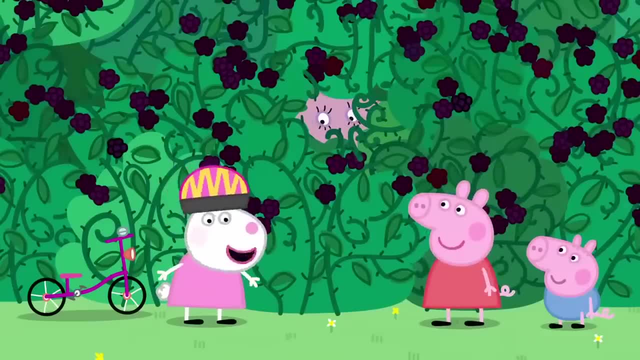 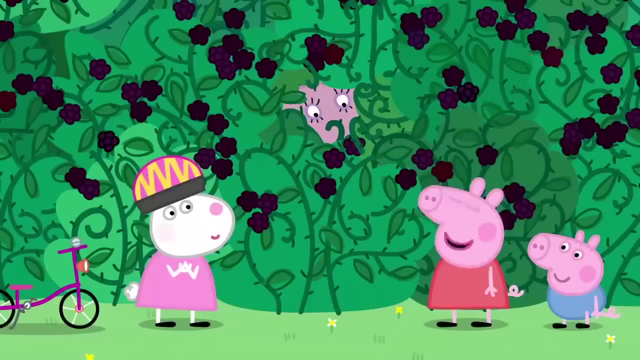 and she'll be there for a hundred years Like Sleeping Beauty, And she'll be rescued by a handsome prince who will give her a kiss. My mummy is having an adventure. I wish my mummy would have adventures like that. Um, can someone think of a way to get me out of here? 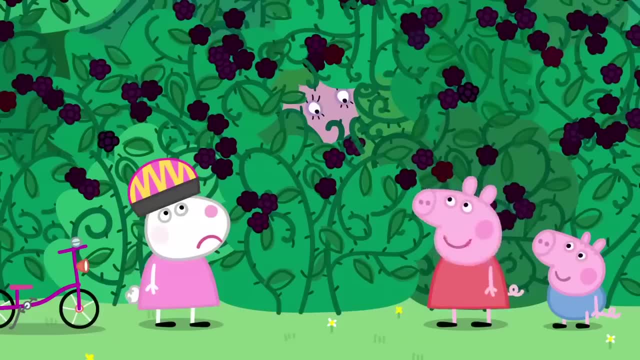 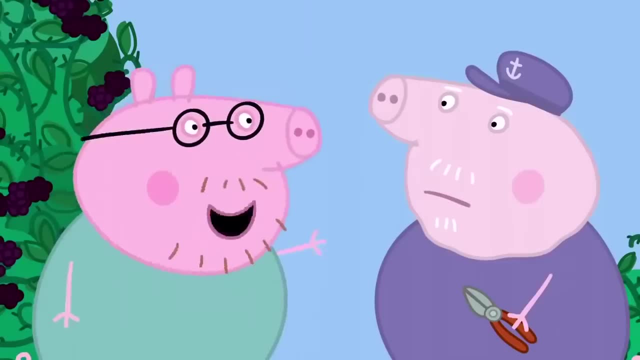 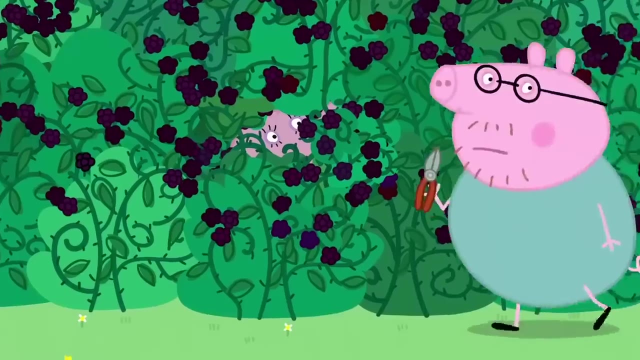 Don't worry, Mummy, In a hundred years a handsome prince will rescue you. I'll be that handsome prince. Grandpa Pig, may I borrow your pruning shears please? Of course you may, Brave Sir Daddy Pig, Stand back everyone. 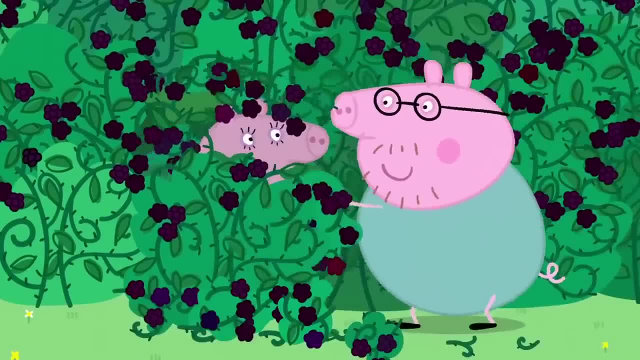 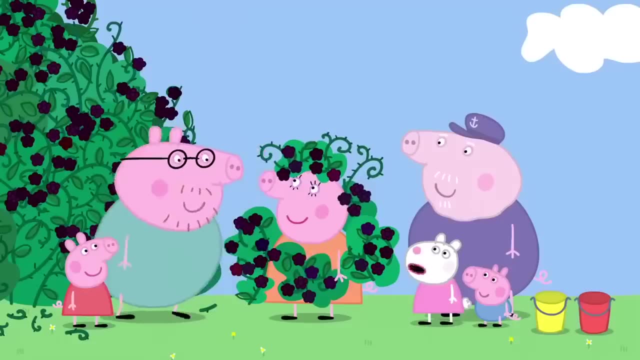 Take that, you thorny bush, you, Yay. Oh, my prince, My princess Mwah, You were meant to stay in there for a hundred years. That was quite long enough. thank you, Mummy is a blackberry, bush. 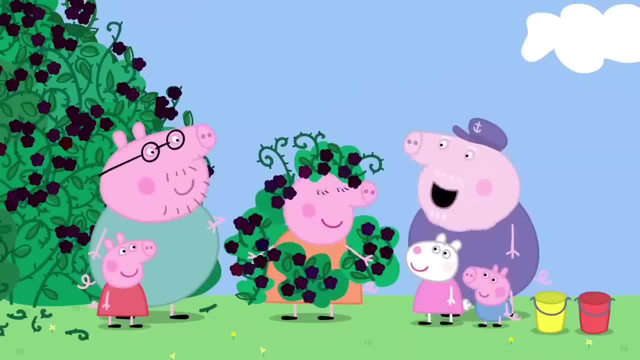 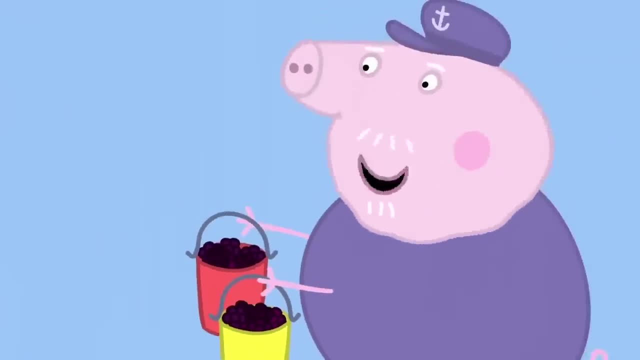 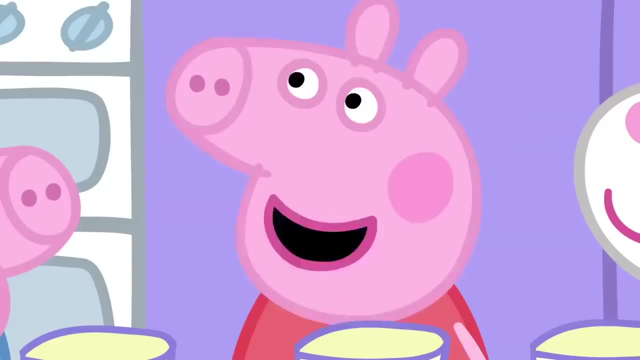 I thought this sort of thing only happened to me. Stand still while we pick you. Let's take all this fruit back to Granny Pig. Granny, Granny, Mummy had an adventure, And then Mummy fell in the bush. She looked quite silly. 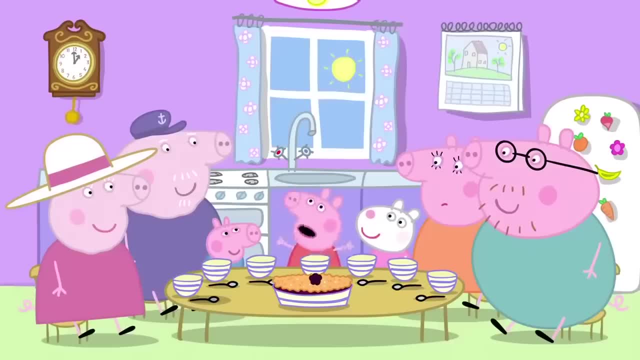 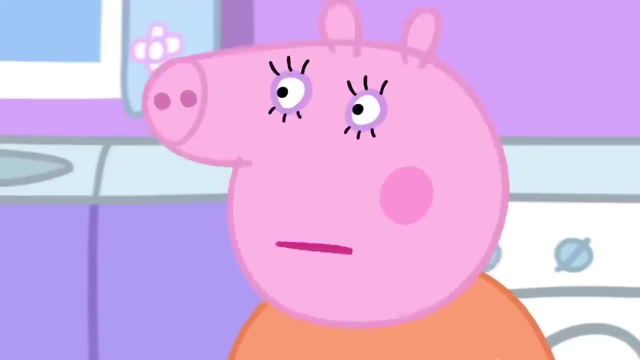 And she was going: Ah, Help me, Help me. And then Daddy came and rescued her- The end. Thank you, Peppa. I think we've all heard that story enough times now, But it's funny. I never want to see another blackberry in my life. 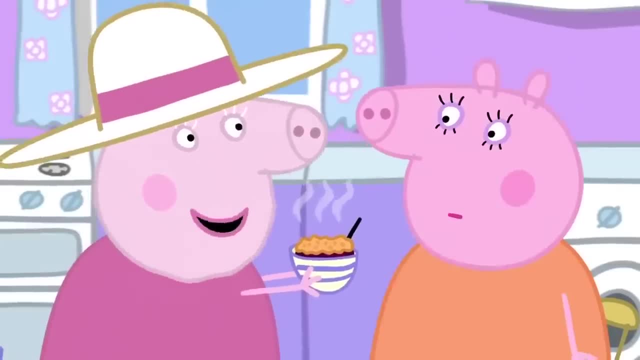 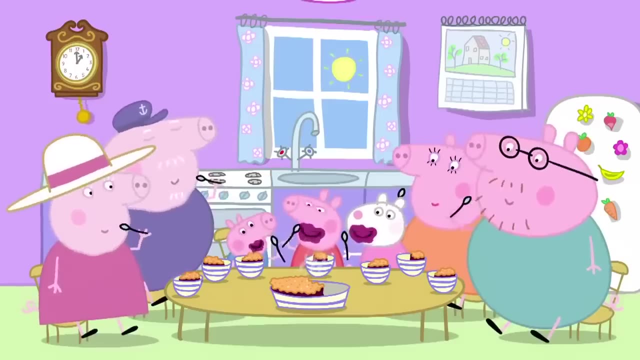 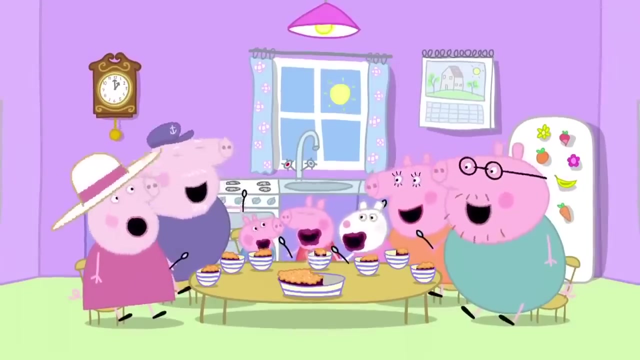 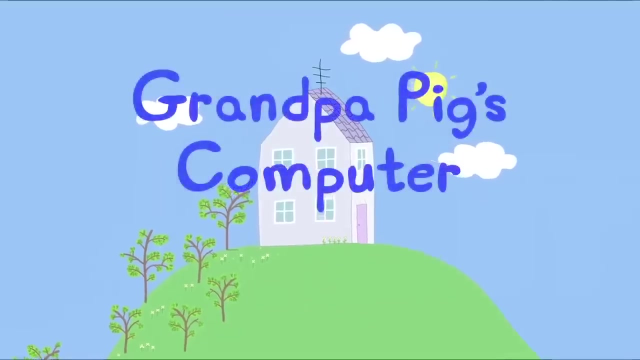 So you don't want any apple and blackberry crumble then Well, mmm, delicious. Mummy Pig loves apple and blackberry crumble. Everyone loves apple and blackberry crumble. Peppa Pig's Computer. Peppa and George are at Granny and Grandpa Pig's house. 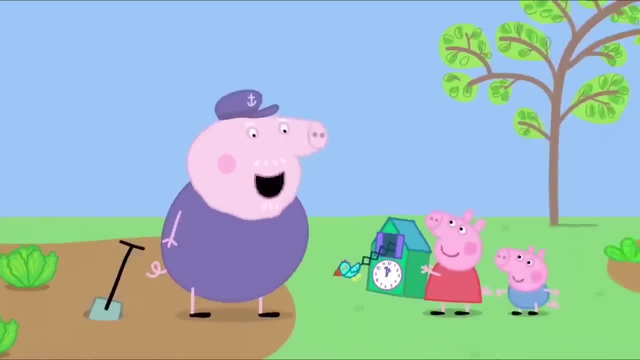 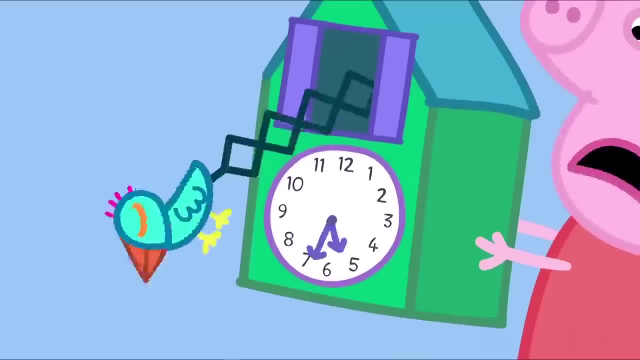 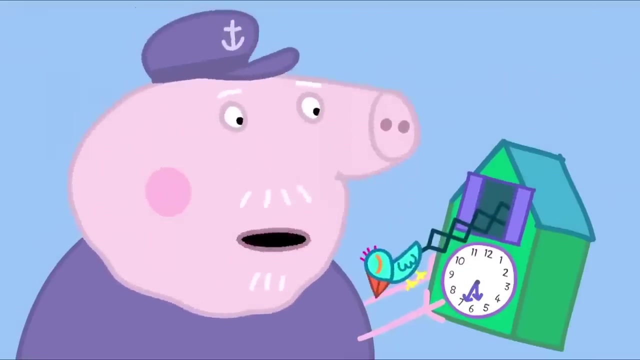 Grandpa Pig, Grandpa Pig, What's this? A cuckoo clock? Yes, it goes cuckoo, cuckoo, But it's broken. Can you mend it please, Grandpa Pig? Hmm, Let's take it to my shed. 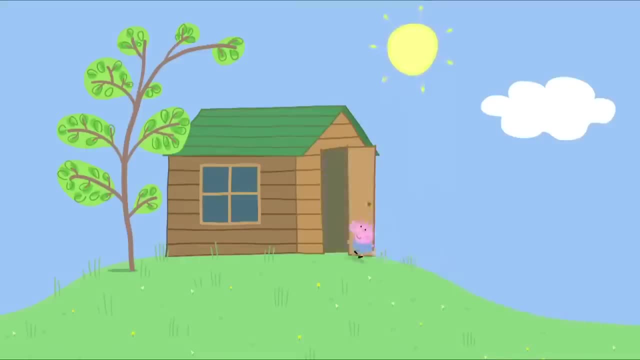 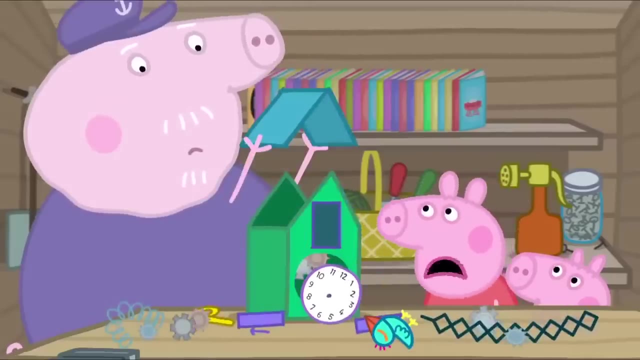 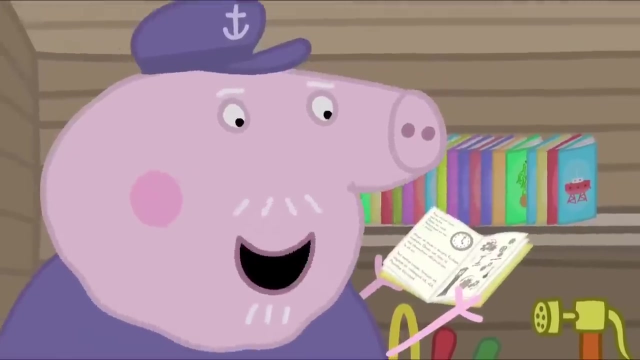 This is Grandpa Pig's shed, where Grandpa mends things. I'll take a look inside, Grandpa. Now you've really broken it. Oh, I wonder if I've got a book on clocks. Ah, Here we are. 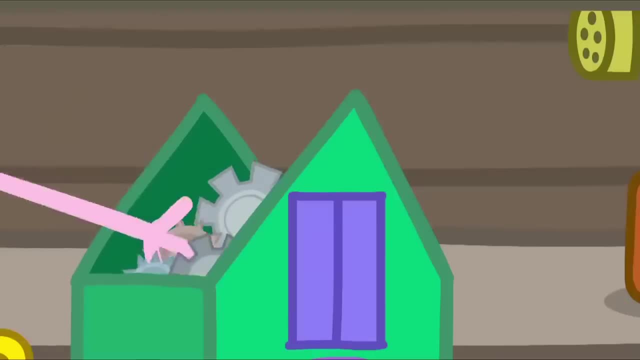 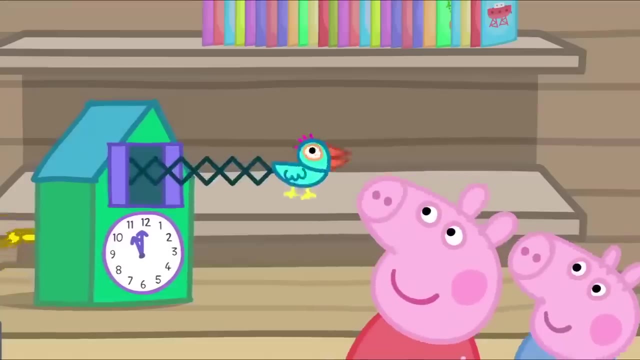 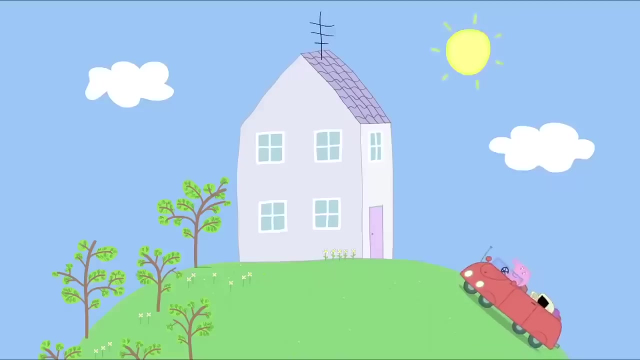 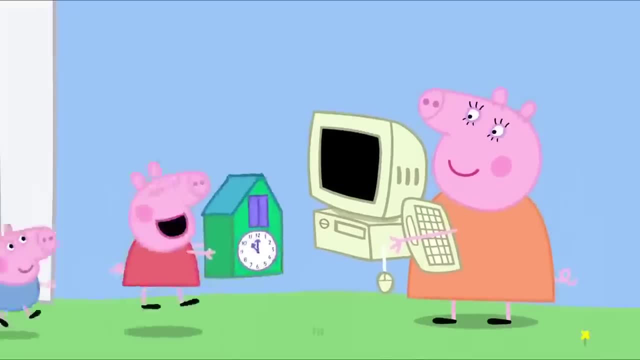 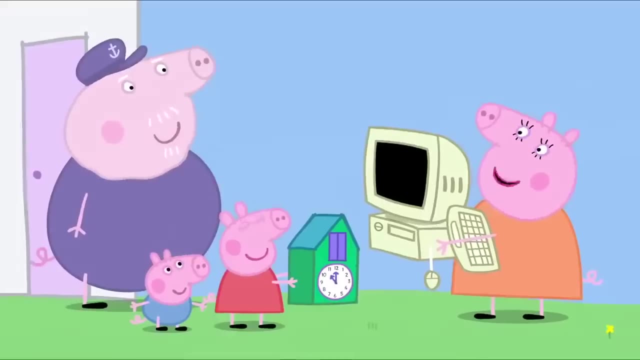 Mummy Pig has come to pick up Peppa and George. Mummy Grandpa's mended the cuckoo clock. That's nice. What's that? It's my old computer. I can't mend that, It's not broken. 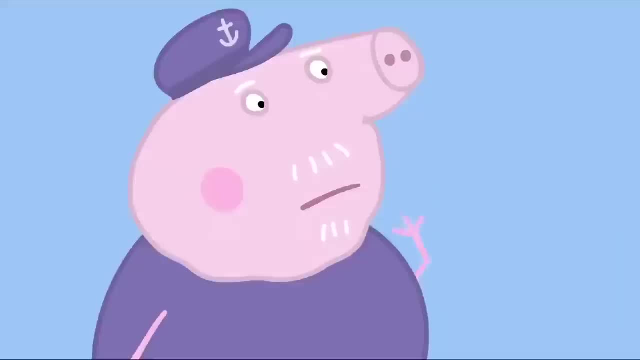 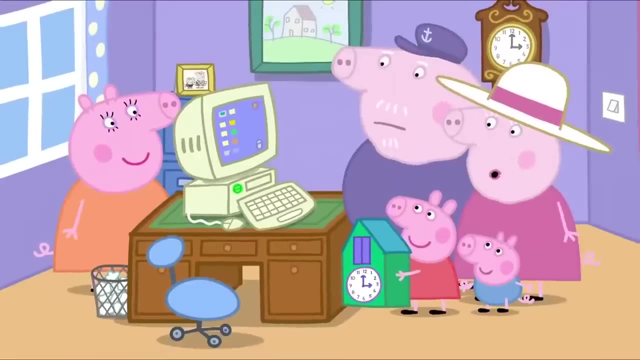 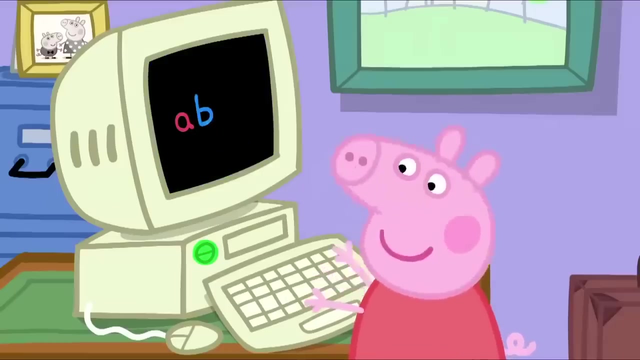 I've got a new computer. I thought you might like my old one. I'm not sure I really need one. Oh, A computer. What does it do? You can do letters with it. Look, Granny. A, B, C, D. 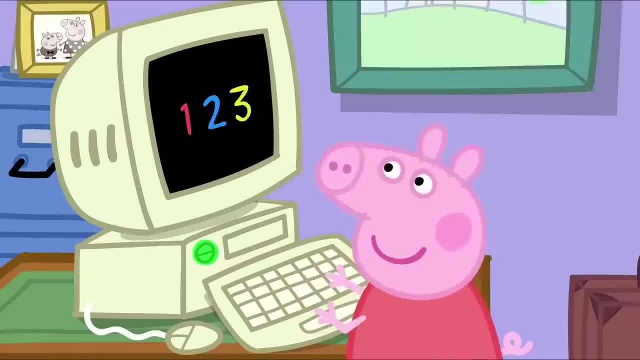 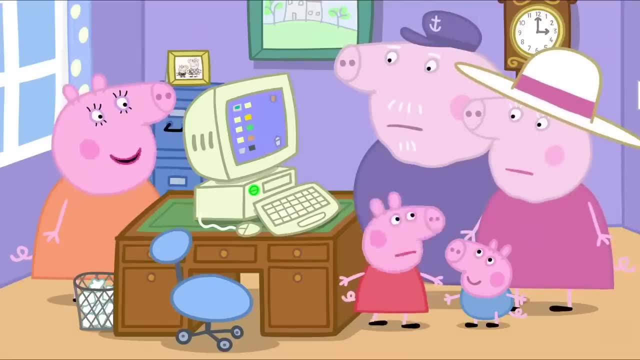 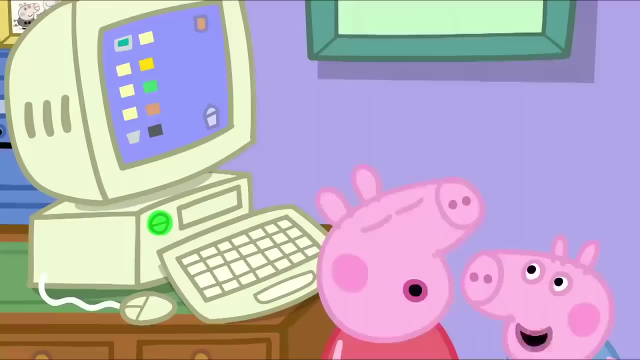 And numbers One, two, three. I'm afraid we might break it by pressing the wrong button. Don't worry, you can't break it. Just don't feed it milk or biscuits or jelly. The best thing it does is happy Mrs Chicken. 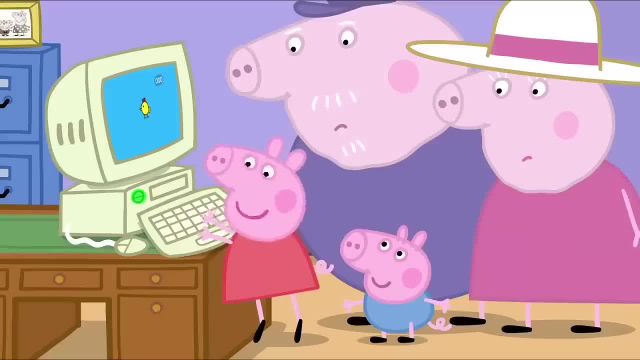 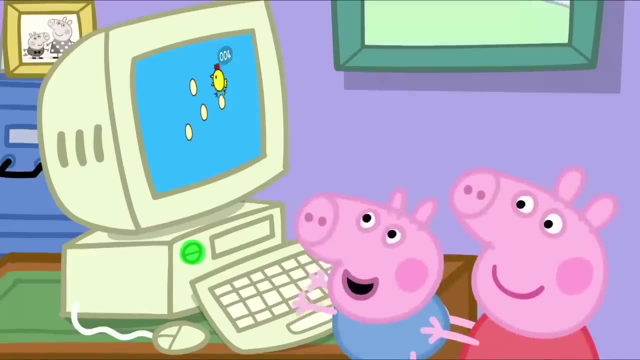 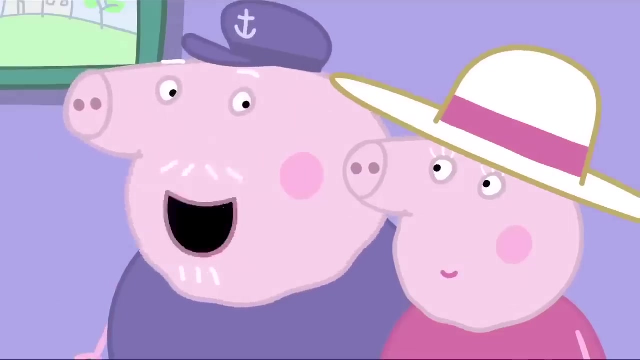 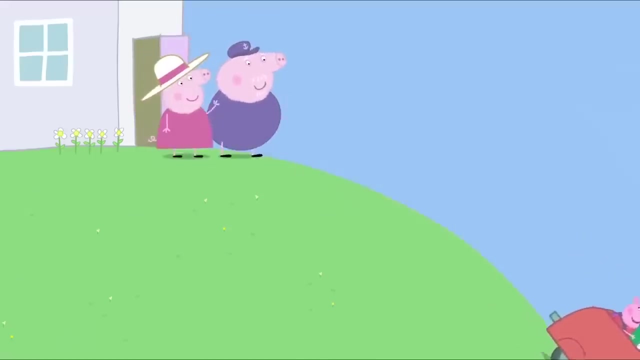 When you press this button, she lays an egg. I am very good at it, But George is the best. That's fun. Perhaps we should keep the computer, Granny Pig. Goodbye, Bye-bye, Shall. we do some work on the computer, Granny Pig. 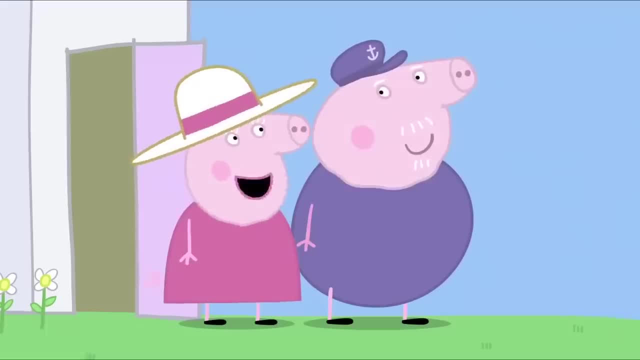 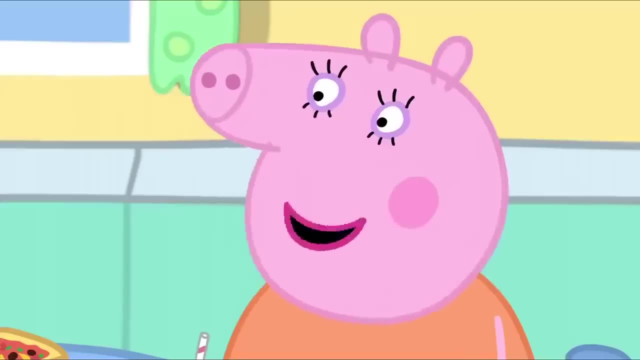 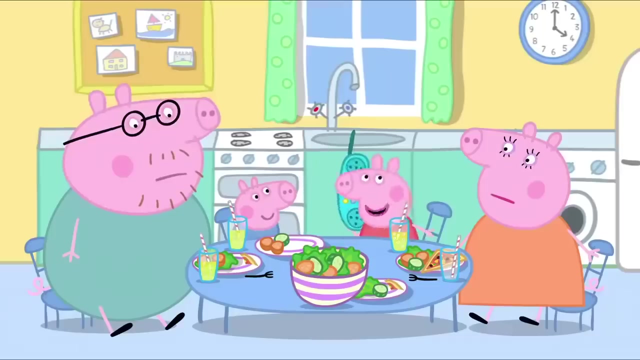 Yes, Let's do some numbers and letters. Peppa and her family are happy They're having lunch. I've given my old computer to Granny and Grandpa. That's nice. I wonder how they're getting on with it. Hello, Peppa Pig speaking. 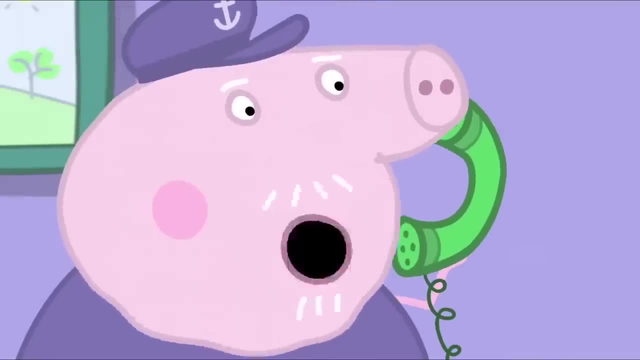 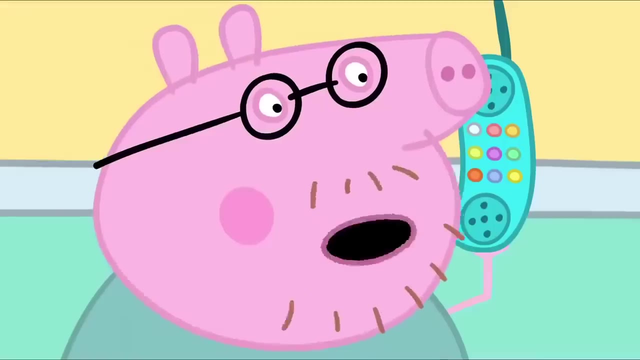 Ah, Peppa, I need to ask a question about the computer. It's Grandpa, He's broken the computer. What's the problem with the computer, Grandpa Pig? It's full of eggs, Eggs. Happy Mrs Chicken won't lay any more eggs. 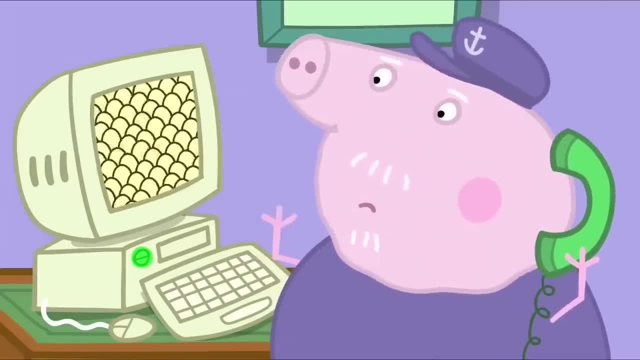 I'm broken. Turn the computer off Now. turn it back on again. Did that fix it? I am very broken. That doesn't sound good. Maybe it can't be mended. We'll come round and pick it up, Granny, we're here to take the computer back. 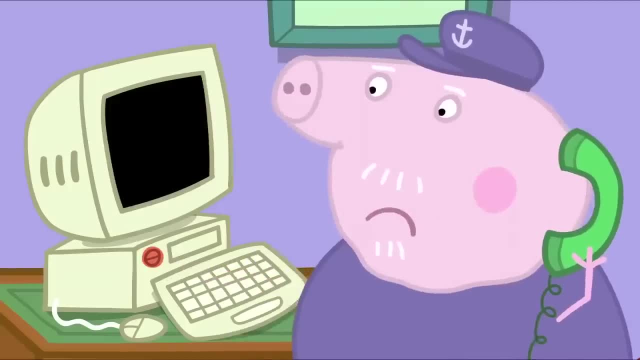 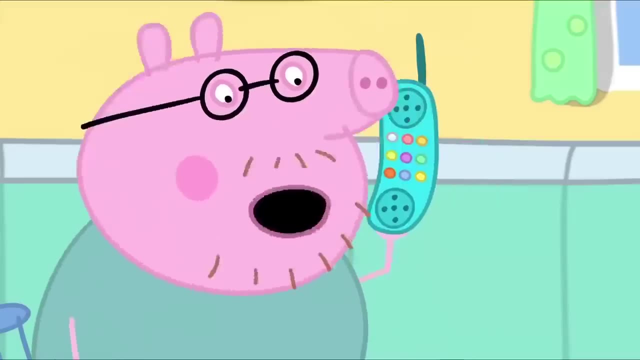 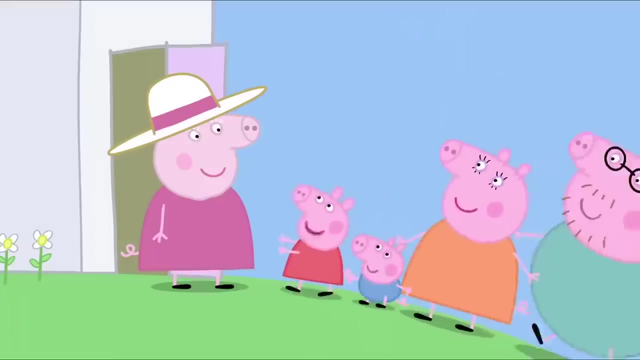